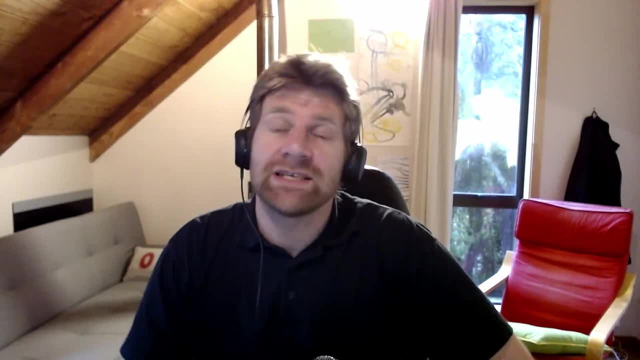 and what we as cosmologists can use them for, and partially his own recent work using those measurements to constrain dark sectors that would alter the thermodynamics of the early universe and thus alter those abundances. So welcome James. do you want to tell us briefly what you'll be? 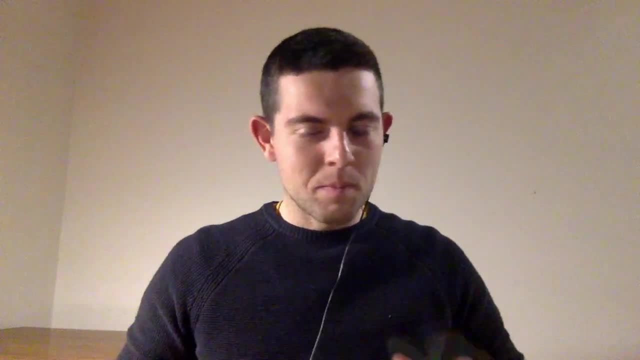 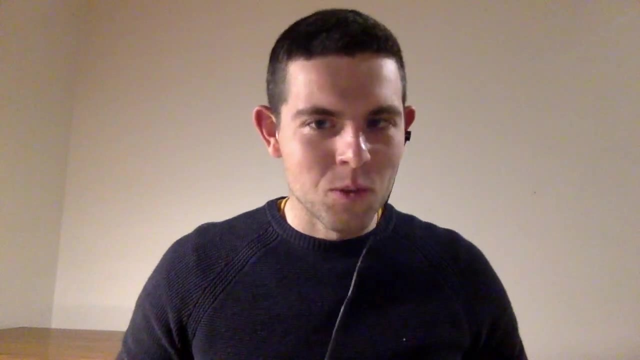 talking to us about today. My part in all of this BBN story kind of was started back in 2019 when I was doing my PhD at King's along with some excellent collaborators there who I'll talk about in a sec. You know we looked at constraints on these MEVs kind of scale because that's the right. 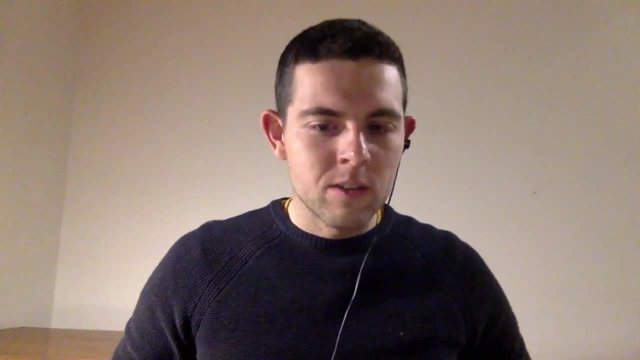 energy scale to pick out when you think about BBN dark sectors and how they can impact the abundance measurements. But in the interim, kind of fast-forwarding to 2021, firstly, I'm very happy that those constraints got used plenty, which has been really nice. But secondly, the lunar 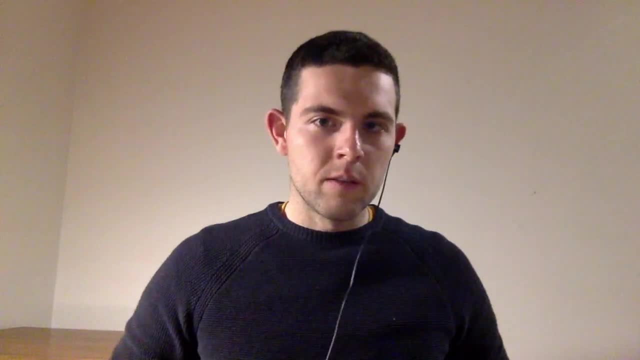 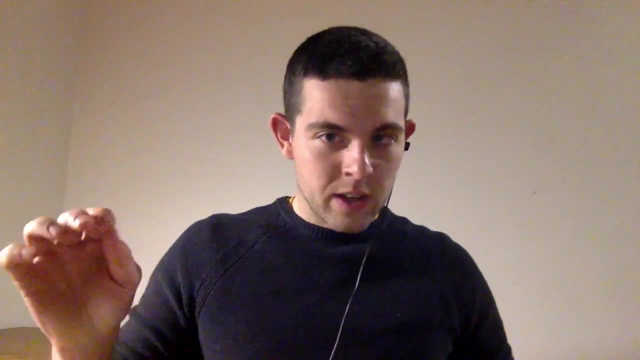 collaboration. so they measure reaction rates for nuclear reactions, things like deuterium going to helium, things like that. You know they made a new measurement and they significantly reduced some of the errors that were really dominating the theory predictions And we thought this is an 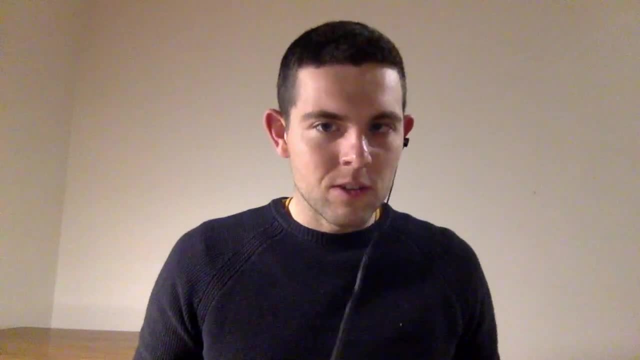 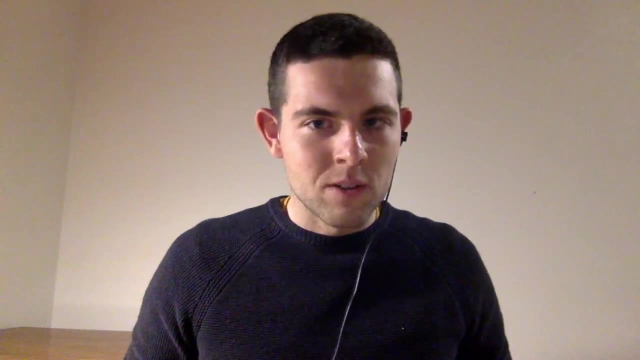 important thing that we need to understand how this decent step forward in BBN theory really affects our constraints. And from that, of course, it's been a lot of fun And I think it's been a nice learning process to understand the context of all of that. So that's, you know, my aim today. a. 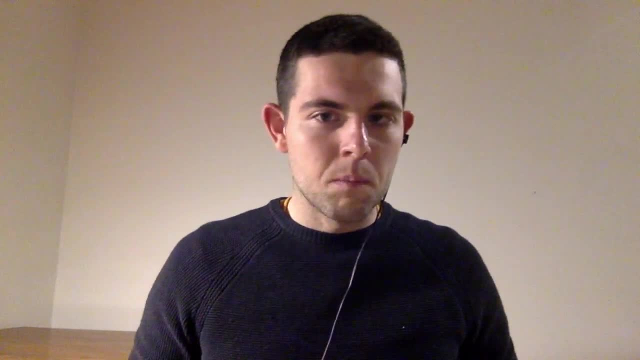 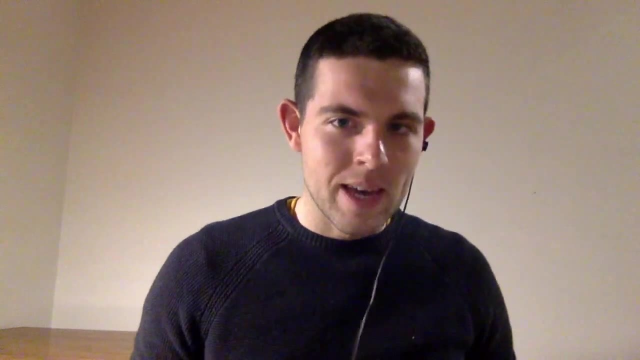 little bit is to discuss, of course, the stuff we did, but also mainly the context of all of this discussion and why BBN in 2021 is different to BBN in 2019,, for example. There were only two things that people did take away from the talk today. What would you want them? 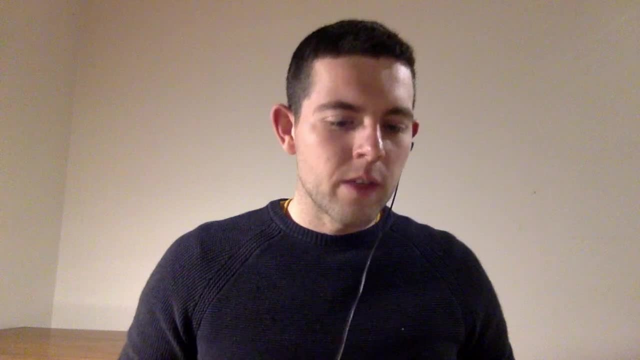 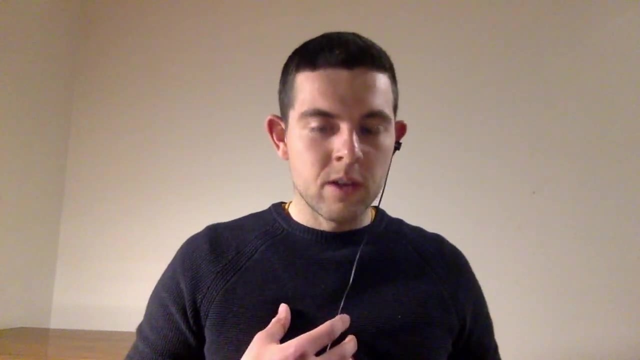 to be if they were remembering it six months from now. Yeah sure. So I think the first thing is that there are many different elements to BBN And especially if you are kind of like myself, a kind of beyond the standard model practitioner. 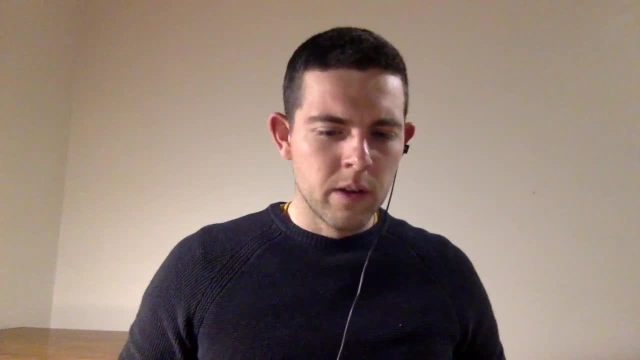 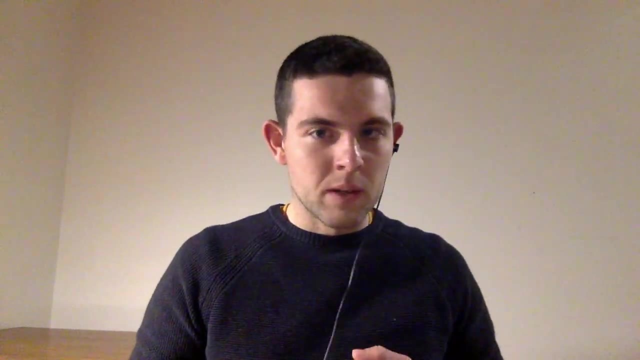 in this regard, it can be often quite easy to focus on modeling the impact of your new physics on BBN, But it's worth bearing in mind that there are many other elements. There are the measurements of the abundances, for example. There are the nuclear reaction rate, uncertainties or 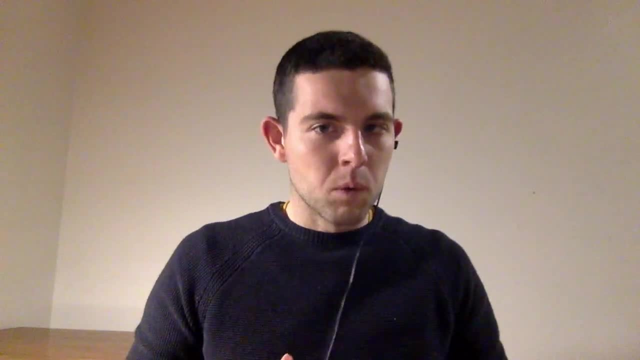 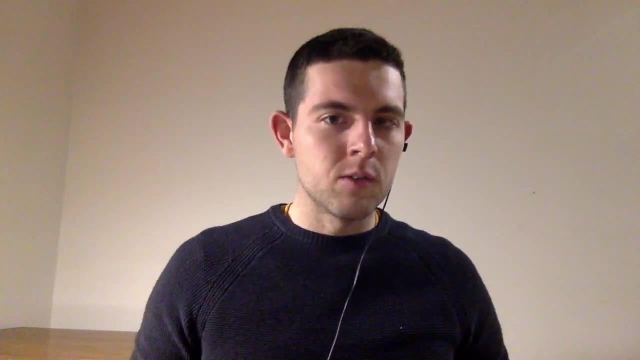 measurements, And all of those play an equally, if not kind of more, important role in, ultimately, what you deduce about the scenario you're interested in. So I think you know the first message from especially this 2021 work is that it's worth trying to understand these updates in. 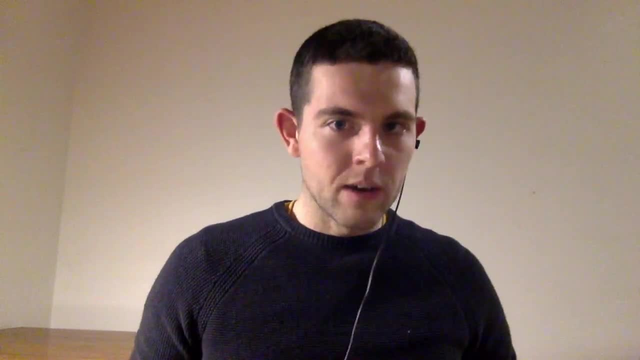 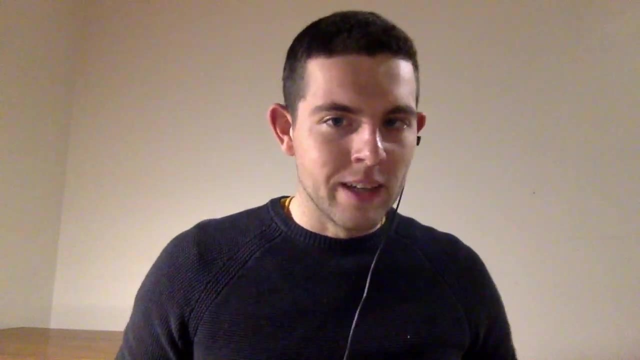 the BBN community And of course you know part of the role of that is from the people putting out the research along those lines. But it's also to really understand how that impacts what you're doing and where it might lead in the future. So that's kind of number one. And the second thing: 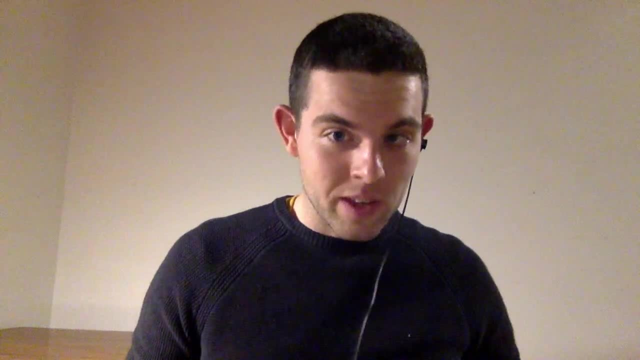 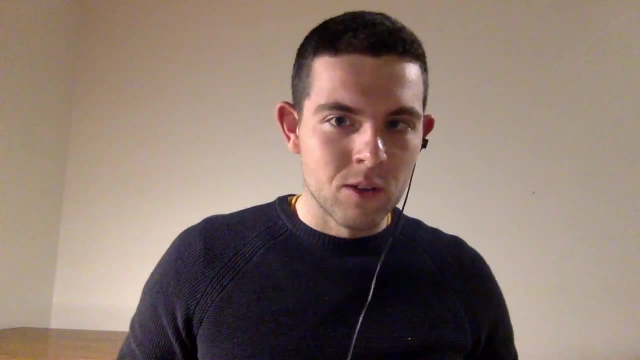 is that you know experimentalists are doing great things, So it's actually worth keeping an eye out for you know, often if you can really reduce your theory prediction, for example, you might be able to say more about your scenario than you thought. But that does rely on you. 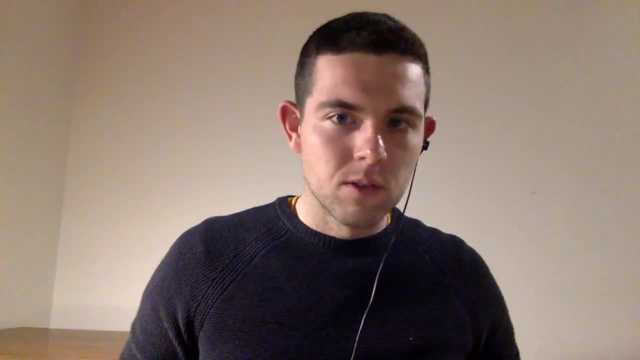 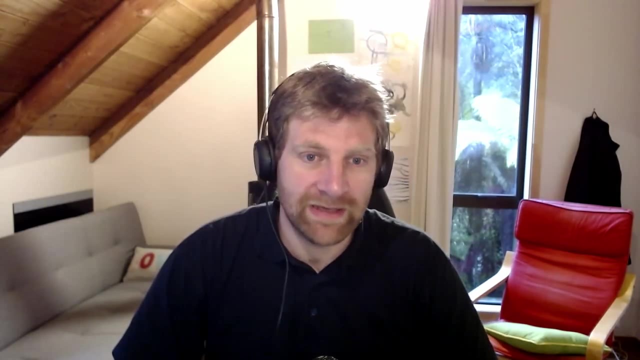 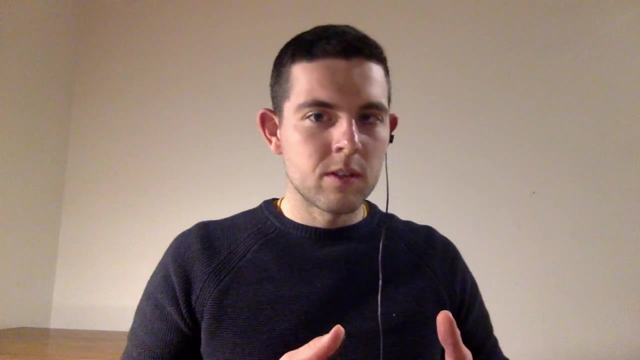 keeping in touch with these issues and measurements. You've sort of already been talking about why this is important, but let's go into more detail now about why this is important for us here in 2021.. Sure, So I think BBN just is a probe both of standard model physics and BSN physics, But I 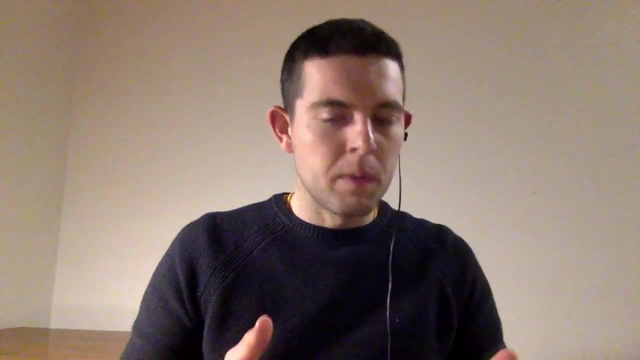 think you know the main real crucial consequences of this. in particular, things like the lunar measurements actually come from standard model BBN And I think that's a really important thing, And I think that's a really important thing, And I think that's a really important thing. 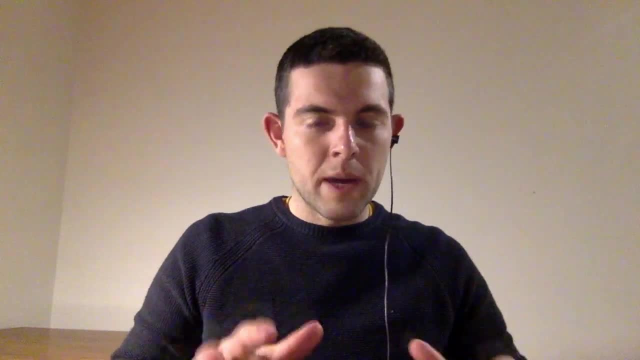 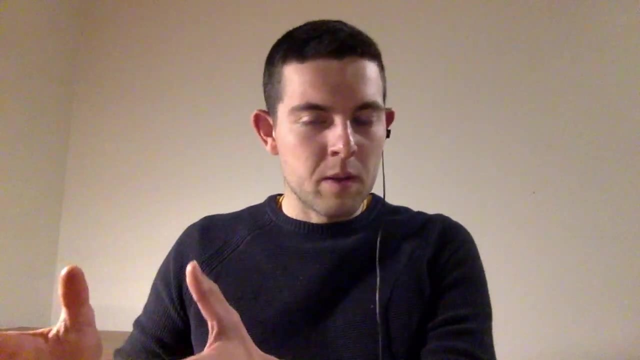 And using BBN, is a kind of so-called bariometer If you want to compare, for example, inferences of the baryon density, like you know, a fundamental parameter in cosmology, from the CMB to BBN. 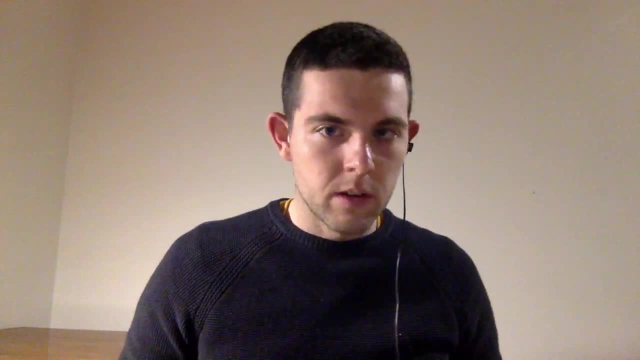 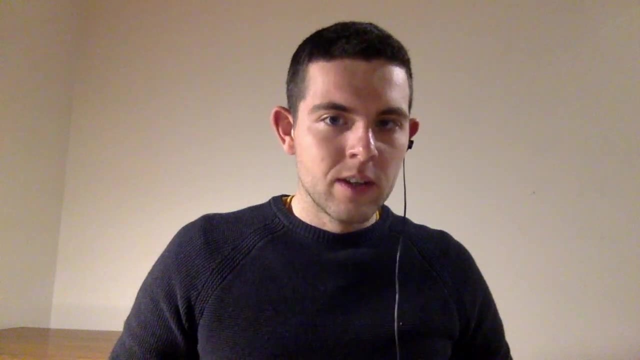 you need to understand the dynamics of BBN and you need to have excellent control over you know all of the different processes going on there And you know lunar. the role that it plays is that it really pins down one of these key bits of physics, which is the deuterium, kind of 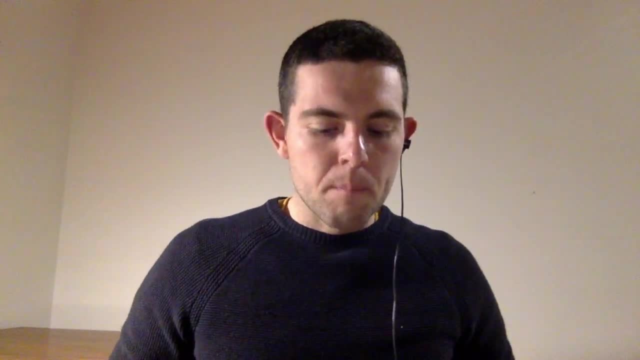 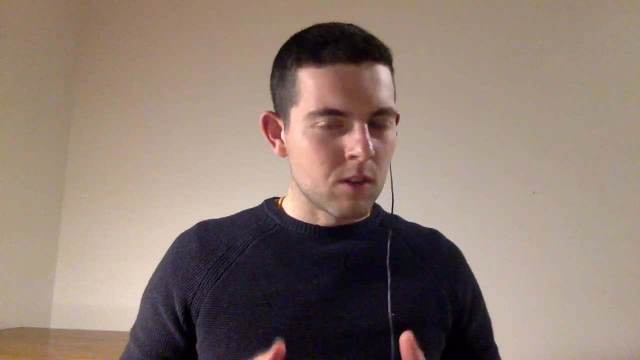 reduction and, you know, annihilation rates. Now there's more context to that and hopefully we'll get into that a little bit later. The context is that when you go through this process, it's not super trivial, Actually, you know there are a number of different ways to approach this. 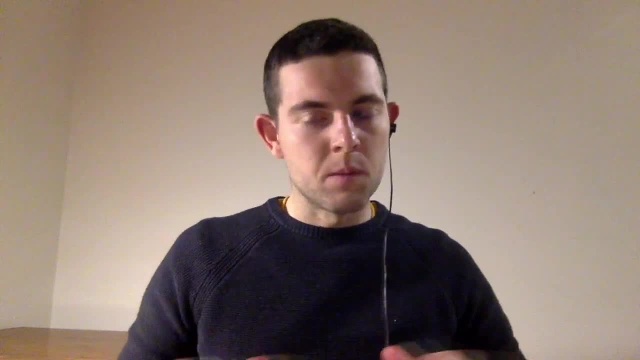 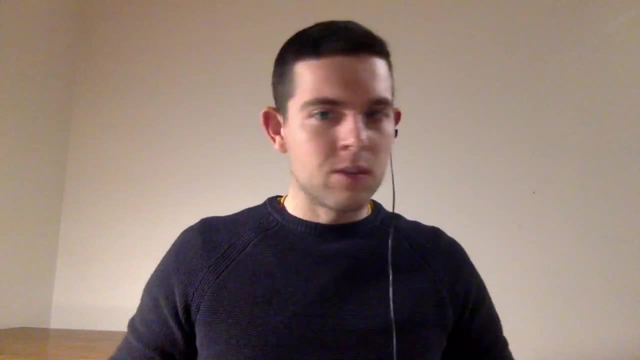 And there's a few kind of key groups across the world, some in Italy, some in the US, some in France, who went through, you know, with the same data and came to somewhat different conclusions about inferences about the baryon density from, you know, BBN And you know. 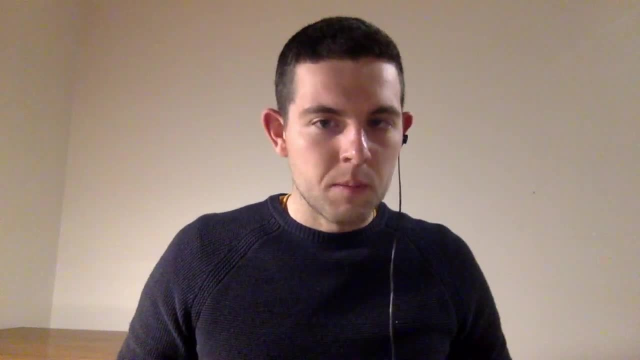 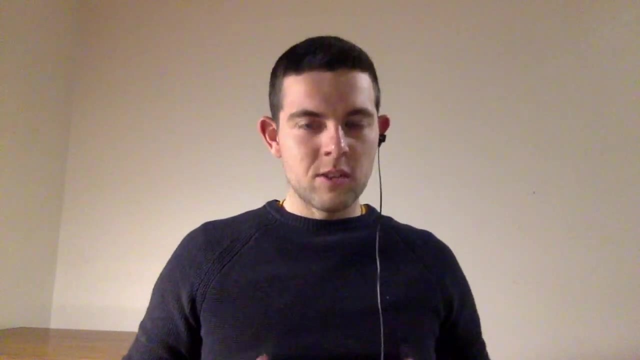 I think this is interesting. It's a crucial parameter right, It is a fundamental parameter in Lambda CDM and it's also the only free parameter in standard model BBN, You know. so coming to a consistent view on this story, even in the context of the standard model. 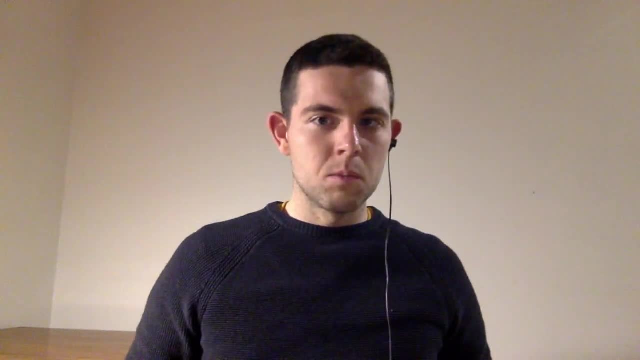 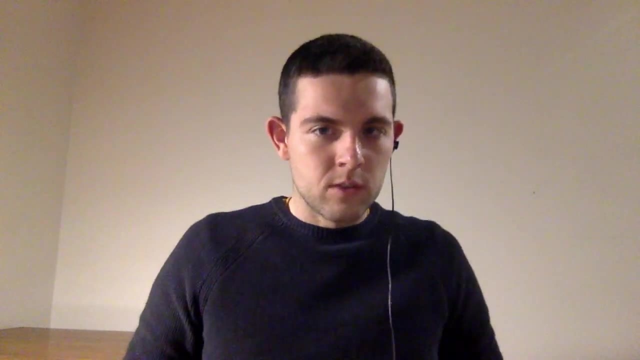 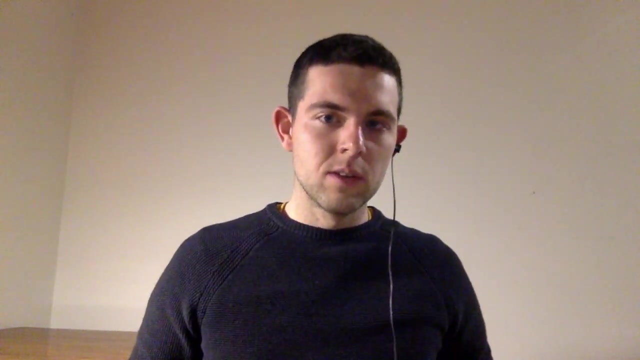 of course, like my personal interaction was kind of BSM, but you know, coming to a robust conclusion in the context of the standard model. I think is really important for you know using BBN as a precision probe. When you say it's the only free parameter is the baryon to photon ratio, then like a 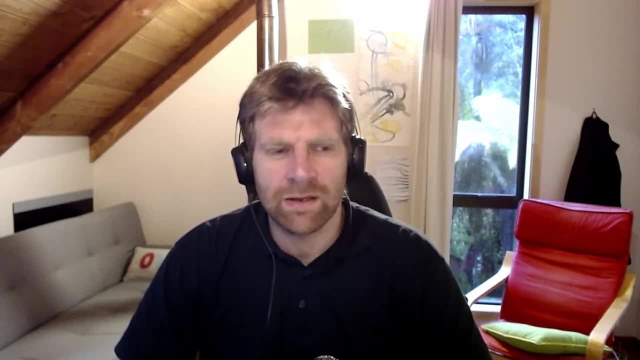 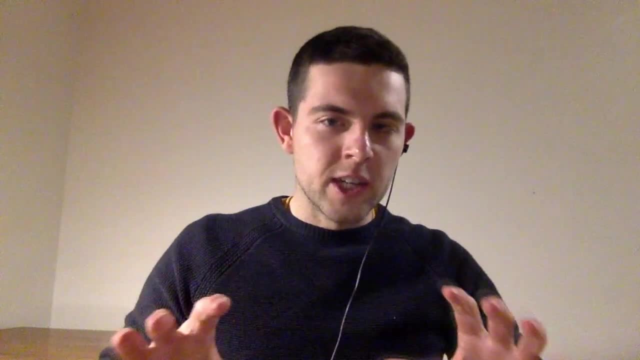 constrained parameter because we've measured the temperature of the CMB so well, or is that not somehow an important parameter? So the baryon to photon ratio- I'm kind of using that interchangeably with the baryon density. You know, one other way to see it is that you could actually take the baryon. density from the CMB. You know you could use that determination and plug that into BBN. So that's the only free parameter in standard model BBN. But if you do want to treat BBN as an independent kind of probe, you should let that vary and see what happens. 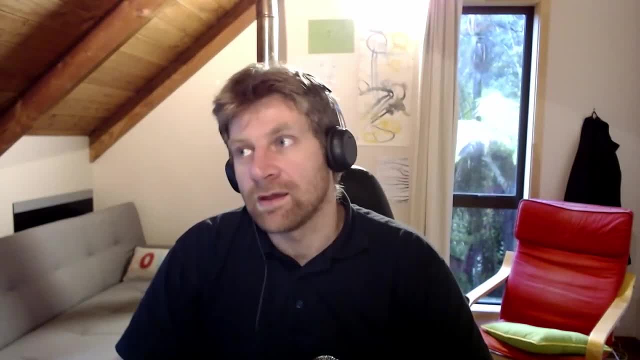 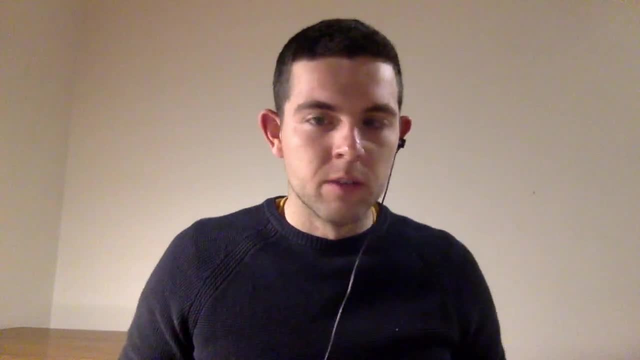 Yeah, and then I guess, if you go beyond the standard model, then the number of photons might be different, because you might have lost or created them. Yeah, exactly, Or any other physics you know, neutrinos or electrons. Shall we get into the details then? 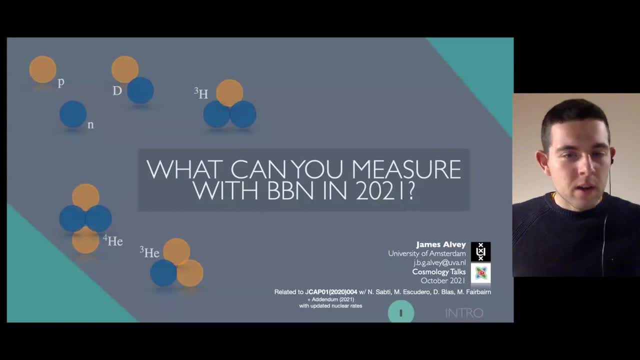 Right, So you know, to pick up on this story, I kind of want to ask this question, which is: what can you really make of the BVN? What can you really make of the BVN, What can you measure with BBN in 2021?? So this is. I say this is related to some work that we did with 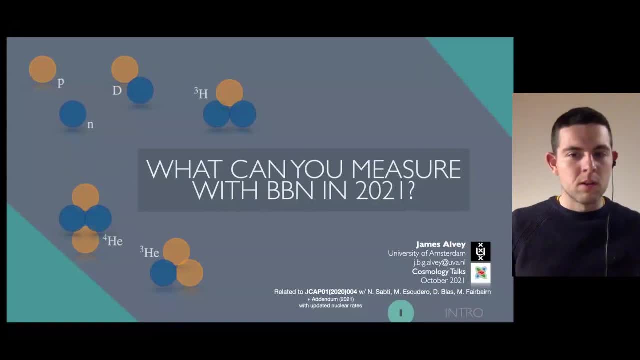 Nash Sabti, Miguel Escudero, Diego Blas, Malcolm Fairbairn back when I was at King's, But that was back in 2019.. And we recently released an addendum on this in 2021.. And the idea. 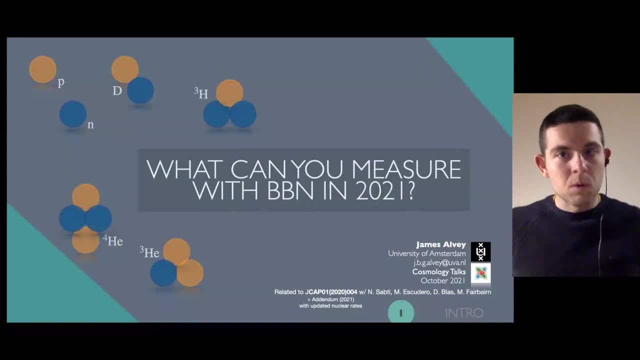 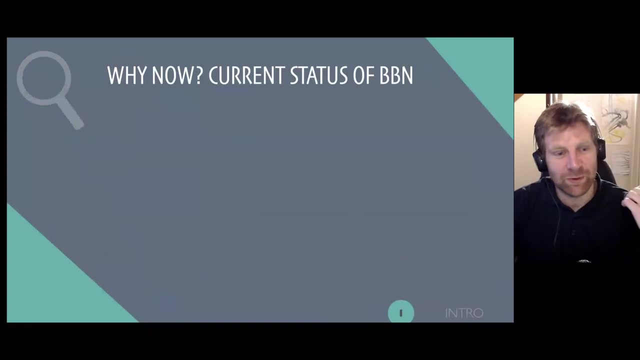 was to include these nuclear reaction rates. So this next portion is hopefully to tell that story about what the context of that is and why we did it. I just want to point out I love the fact that you had an addendum. It's so cynical to write a whole new paper when perhaps you're just updating a small. 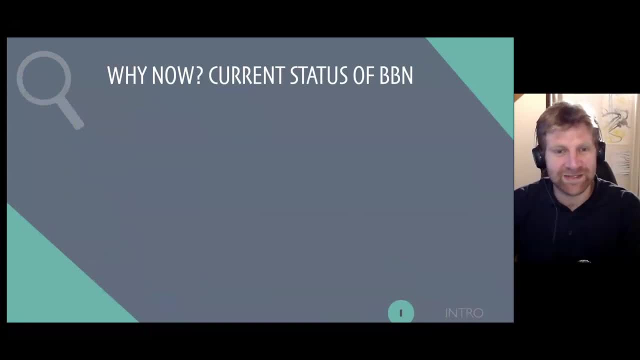 piece, And maybe in the mid 20th century you had to write a new paper because it had to be sent around the world. blah, blah, blah, blah blah. But in 2021, there's just no reason that we have to do a new paper for every tiny little piece of knowledge. I mean it even. 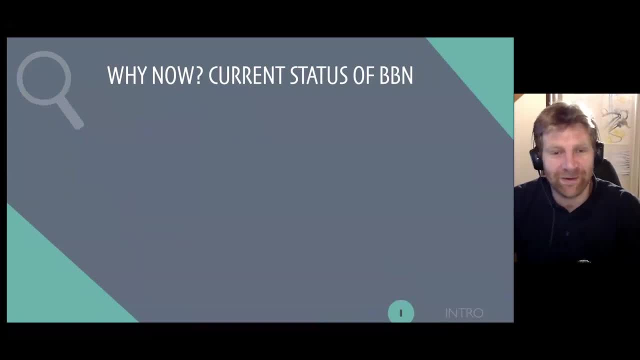 saves us trouble of having to write the introduction again, but in different words. and all of this when you can just say, hey, old paper, still relevant, new results. Here's just a new section, 100%. Yeah, I mean, that's what we want to do. We almost thought about submitting as like. 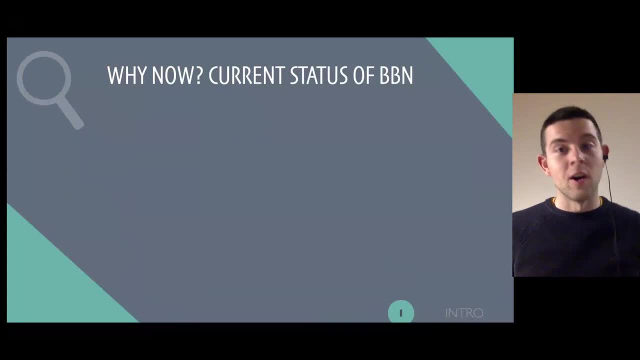 an appendix or something, but that messed up with all the publishing. Like you can't do that it turns out But yeah, I mean there was no point in writing a new paper. It's just like: oh, we did this check because we didn't have the data in 2019, and now we do. 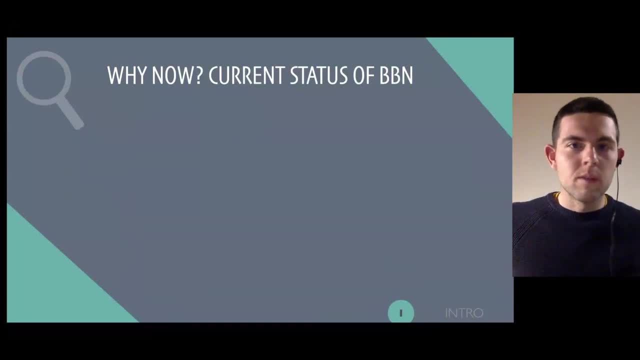 So we're going to use that. So this is the real question: Why now? And, I think, to understand why an addendum in 2021 was the right thing to do. it's good to think about the current status of BBN and all the 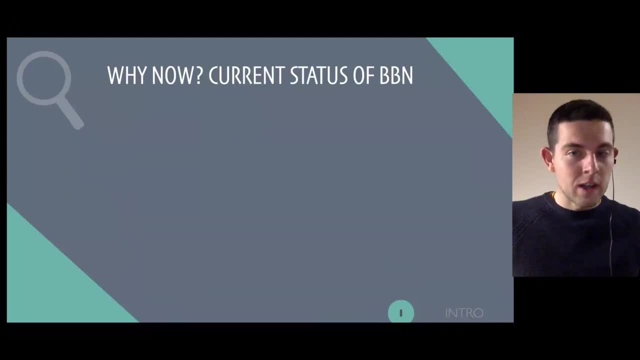 different parts that go into it. So first off, crucially, if you want to use BBN as a probe, you really need measurements of the abundances. So in particular, kind of the four helium abundance and also the deuterium abundance- Now at the moment from blue combat galaxies, for example, for helium. 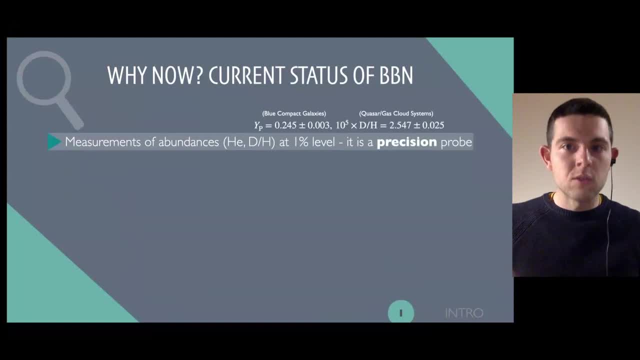 or quasar gas cloud systems. this is really like a precision probe today And it's at the level of kind of 1%. I'm not going to talk too much about that, but there are some excellent talks, kind of online, or slides, to explain how that process is done, And I think 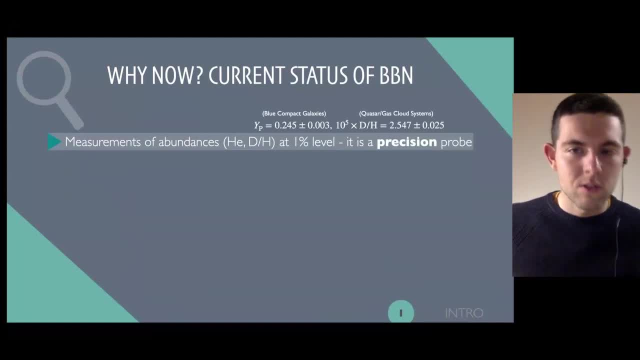 that's really important And how to extract that information from the astrophysics. But you know that's a crucial part of using BBN as a probe of any sort of physics, whether it's in the Sander model or beyond. 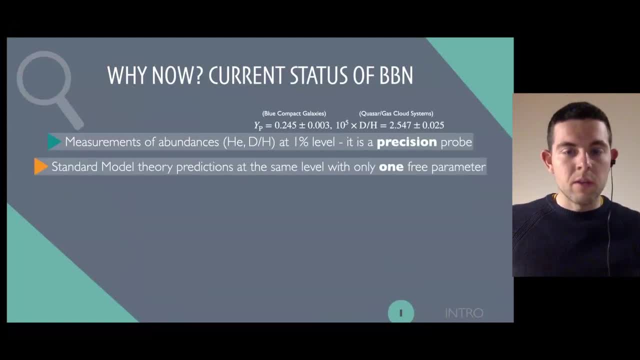 The next part is kind of what we discussed a bit before, which is that there's a theory element to this And within the Sander model, this is now super well controlled. I'm going to mention some of the different elements that go into kind of BBN theory in 2021 later. 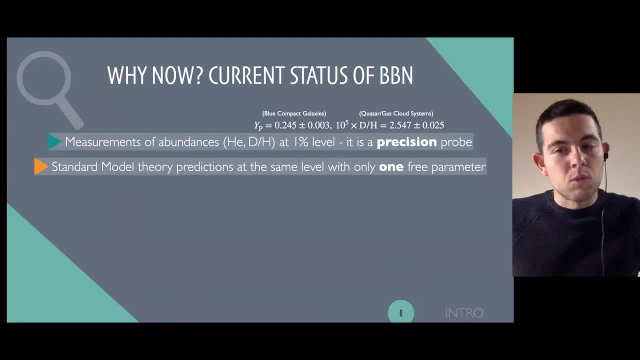 But at the level of kind of predictions, there's really only one free parameter and that is the baryon density or kind of equivalently, the baryon to photon ratio. Most relevantly to our work, there's also updated measurements of key parts of the reaction network And 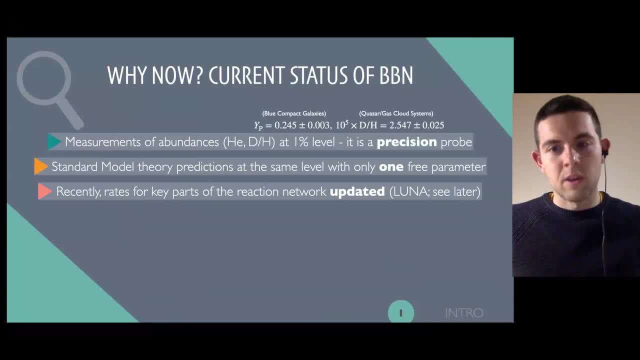 this is the Lunar Collaborations role in this And, as I say, we'll talk about that more later. That does require some context to really understand the implications, But for now, you know, the fact that there are updated measurements that came out in 2020 is kind of part of the key. 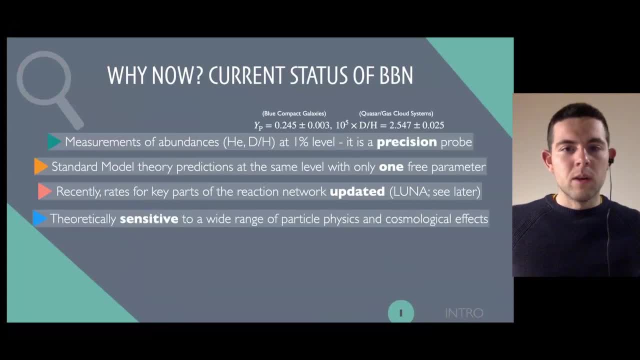 And then you know, finally, just from a standpoint of using BBN as something to learn about physics, you know it's very sensitive to a wide range both of particle physics but also cosmological effects. And all of the above reasons, the fact that you have 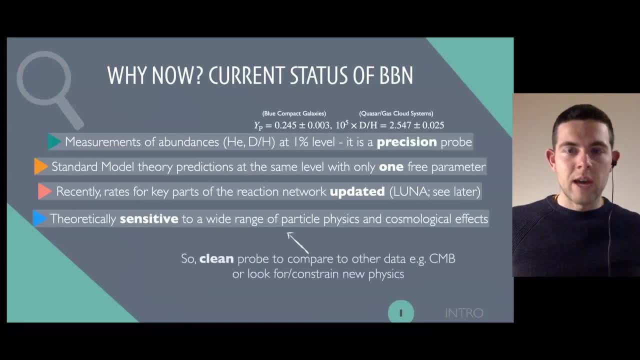 good measurement of the abundances, good theory predictions and also- you know now, very good control over the rates and the reaction network. that makes BBN like a very clean probe to compare either to other data, if you want to do Sander model physics, or to 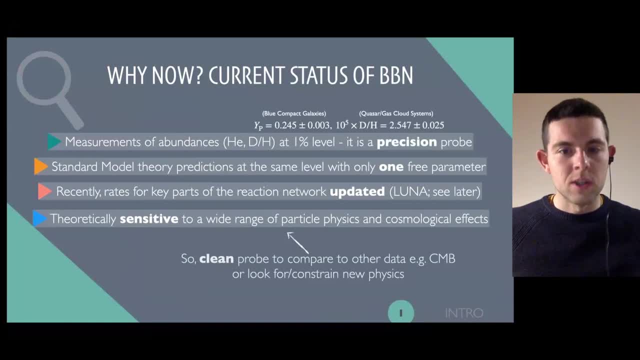 look for and constrain new physics, which was, you know, our motivation for it. I kind of have a couple of questions at this point. So when I was growing up, in cosmology, the primordial lithium abundance was a problem. Is lithium not as sensitive now, Like are? 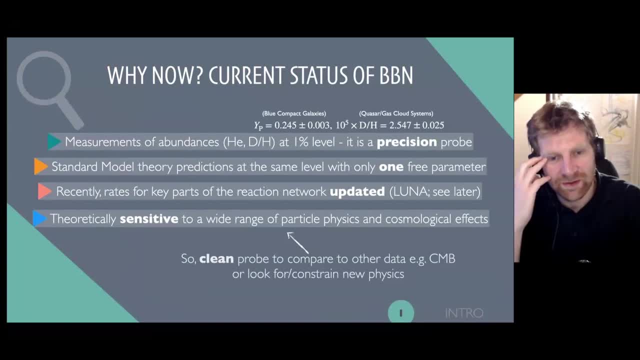 these other probes so much better measured that lithium is kind of not important. I think lithium is still a problem. It depends on you know. I think the measurement of lithium is not at the same rate. It's as robust as helium and deuterium, mainly because of these issues of do we know exactly? 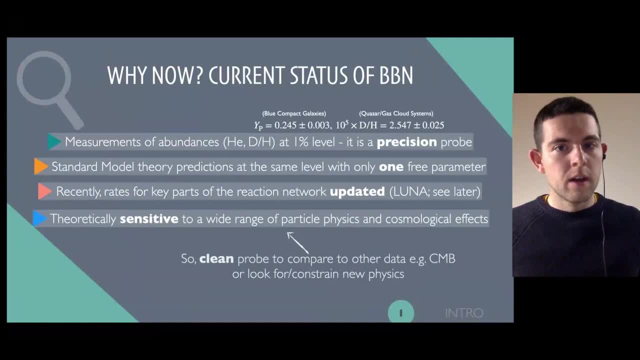 how it's, for example, produced and destroyed in young stars. However, you know that by itself is not a reason to dismiss a lithium problem at all. So I think that's actually part of kind of outlook as to where to go. you know where things might go next. But 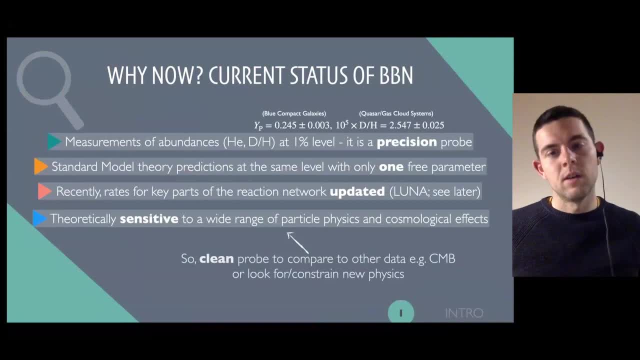 yeah, I think that that remains an issue, an open issue in BBN: either measurement- perhaps it will turn out to be- or theory. You know one of those two, I guess. the other thing that I find kind of interesting is that BBN is so, so useful as 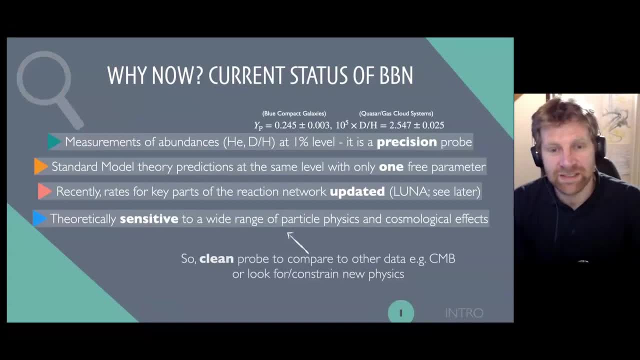 a probe that new nuclear physics measurements actually do make it a better probe, if that makes sense. I mean if it makes sense as to why I find that surprising. I mean it's one could imagine an alternative scenario where the uncertainties in the cosmology were. just so large that, yeah, okay, Luna went out and measured some cross sections better. and it's like okay, I mean, our negligible source of error is now even more negligible. Like thanks, Like if you went and measured the mass of the electron slightly better, it wouldn't. 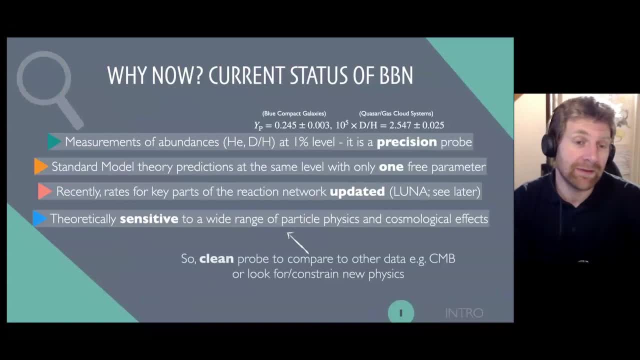 necessarily change cosmology that much, But instead it's the other way around, that these were the leading problems. I think that's, yeah, one thing that's worth saying there is. that's testament also to the first point on this slide, which is that one of the reasons that you've got into this position. 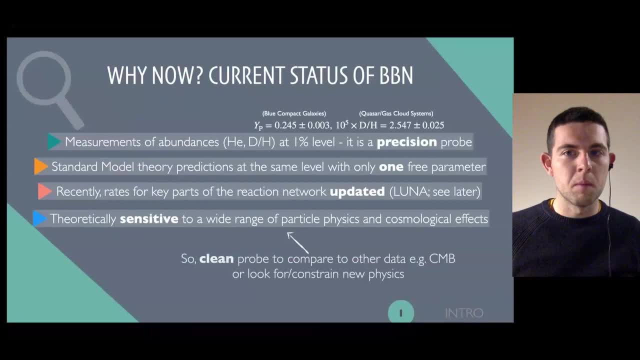 where measurements of, you know, literal nuclear reaction rates become important is because on, in this case, deuterium from these like quasar gas systems are so good. And you know, those are some people, people like Ryan Cook, for example, who worked very hard to get the 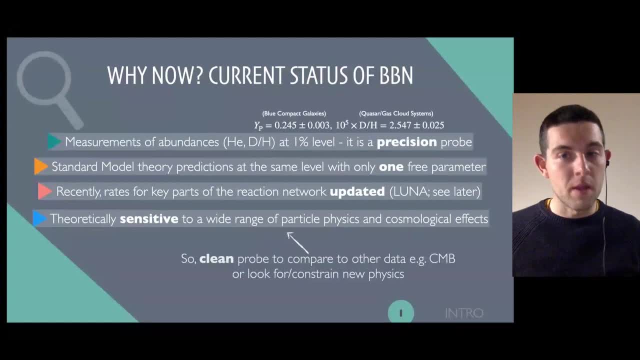 observing time to make that measurement And they actually. deuterium, for example, has very good prospects in that regard. There is helium. it's slightly less clear, but actually for deuterium there are prospects to reduce that, you know, below the 1% level And then 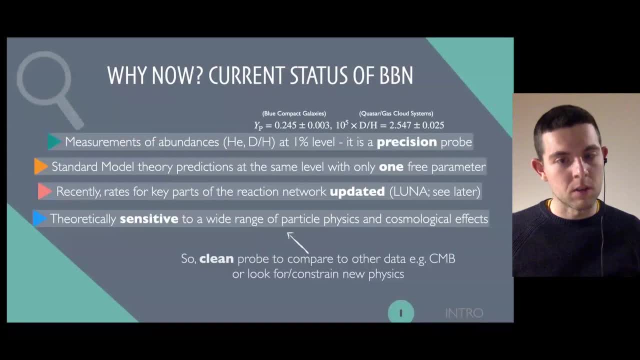 these lunar reaction rate measurements take on even more Significance in that regard. Is this still like an issue at all? Or maybe I'm just being naive here, but yes, okay, you can measure the helium in blue compact galaxies and deuterium and hydrogen and quasars. 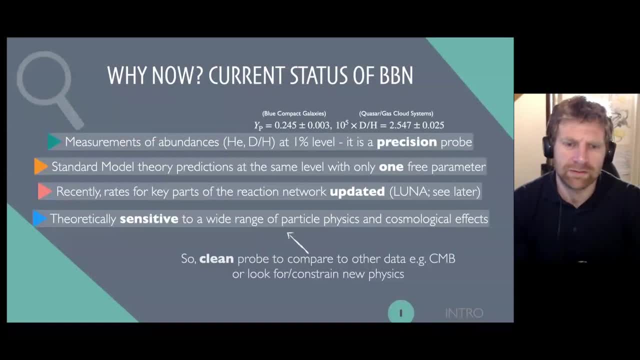 It's the same as that lithium problem. How do you know that that's primordial and not primordial, I mean, I think I think one thing you have to do is kind of play a bit of a Occam's razor game and say, okay, I also have BBN predictions right, And the BBN predictions are, you know? 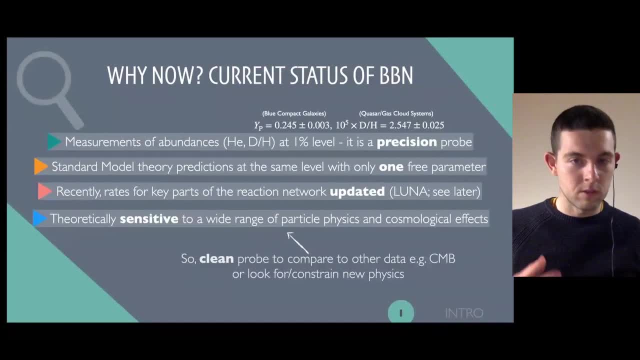 predictions agree very, very well with my measurements. I have no reason to go beyond that, given that I think the measurements. I've done everything I can to ensure that measurements really are measuring primordial abundances And I've done everything I can to control all the theory uncertainties in my BBN predictions and they come to the same. 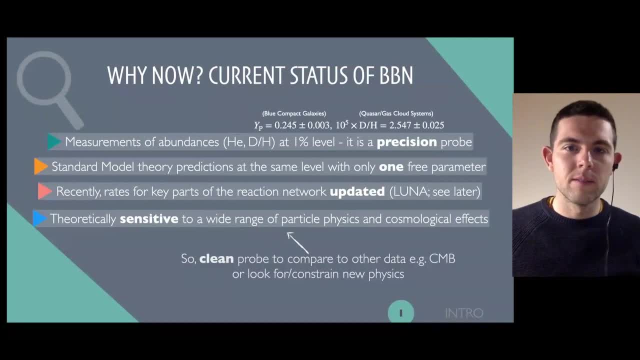 number. I don't know. again, that's not a, it's not a proof. but Yeah, I was wondering whether there might be some sort of like redshift convergence plot, that like, as you go to earlier and earlier times, you're converging on some number. 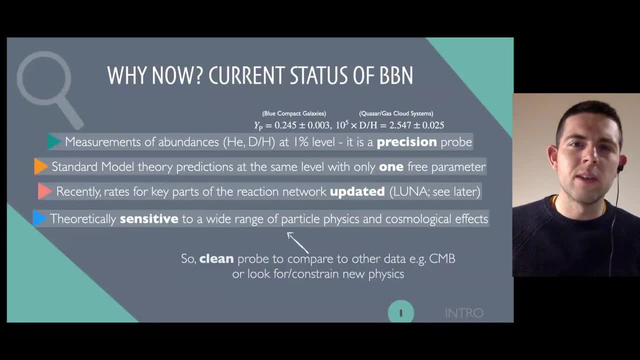 I think in terms of it may it might not be redshift convergence, but I think in terms it may it might not be redshift convergence but it might be some sort of like redshift. I think there is a kind of metallicity convergence plot. So typically in these systems you go: 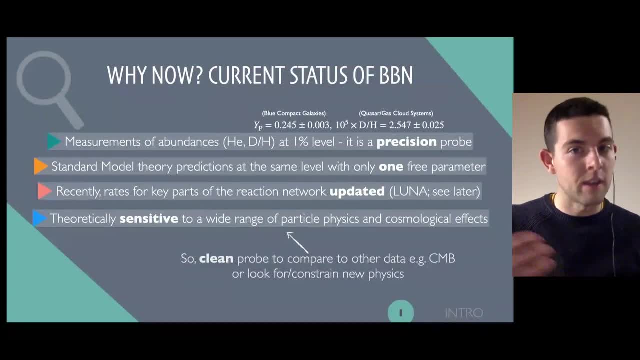 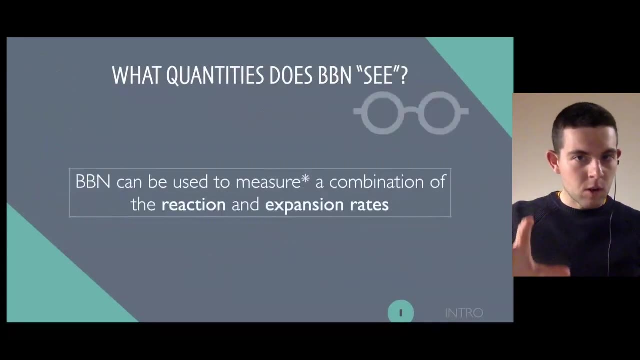 and look for very low metallicity environments, because that indicates like less star kind of activity. So I think you know that that's your measure in that regard. Yeah, So this is kind of the question I'd like to pose today a little bit, which is in this context. So 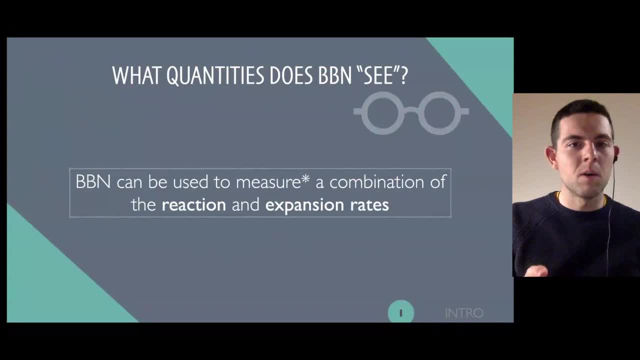 you know, not not in general, but in the context of 2021, with 1% errors in the measurements and very good determinants, Some, some of the reaction rates. what can BBN really be used to measure? And my argument: 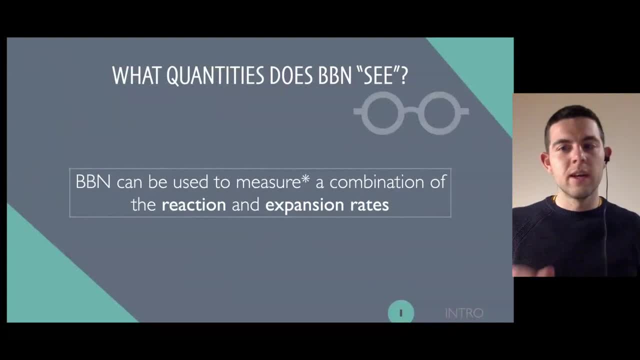 is that it can kind of be used to measure a combination of a couple of things. You can kind of measure, or at least be sensitive to, the reaction rates, be that weak or nuclear interaction rates, but you're also sensitive to the expansion rate of the universe And 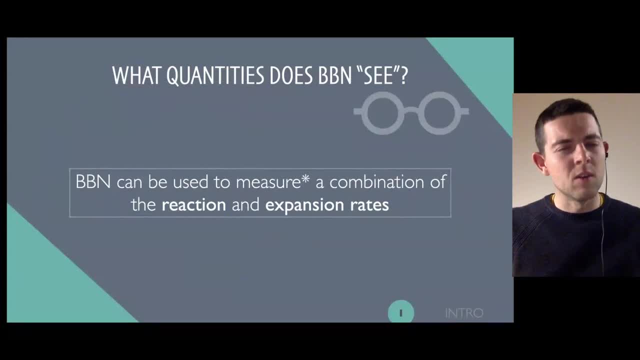 that gives you. you know- there's a little caveat here, of course- that the effect that you're looking for- perhaps it's in in the context of new physics- that has to be large enough compared to your measurement errors. But these are typically the things it's sensitive to, And this is kind of what I'd like to focus. 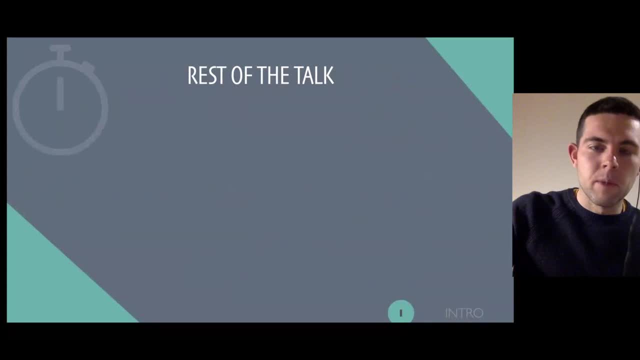 on, Right. So the rest of this little bit. we kind of went over the intro, which is like why now And what? what can BBN? what can BBN do, or at least what is it potentially capable of doing? To go beyond that, you know, I do think it's useful to think about the 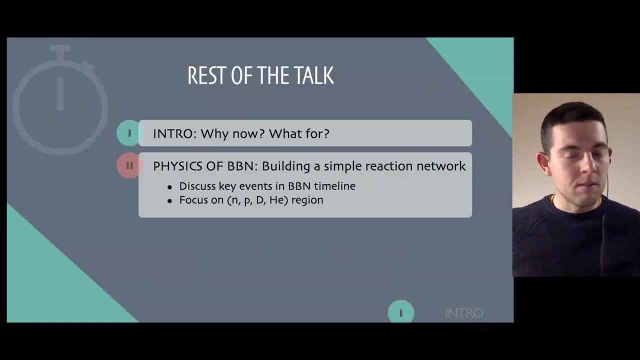 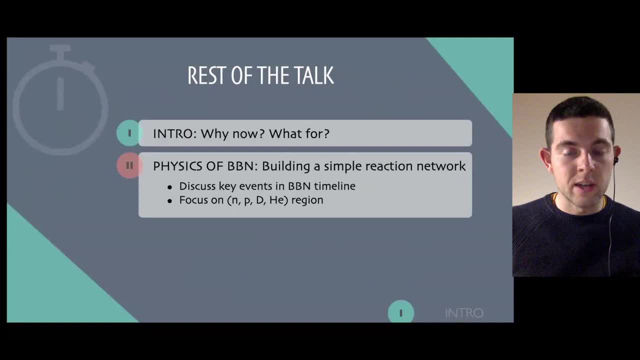 have time to think about it, but there's a lot of physics, mathematics that we probably could put that work on All right, So let's get started actually. So there's the full BBN description. I'm going to take a slightly smaller focus and focus mainly on this reaction network, Of course. 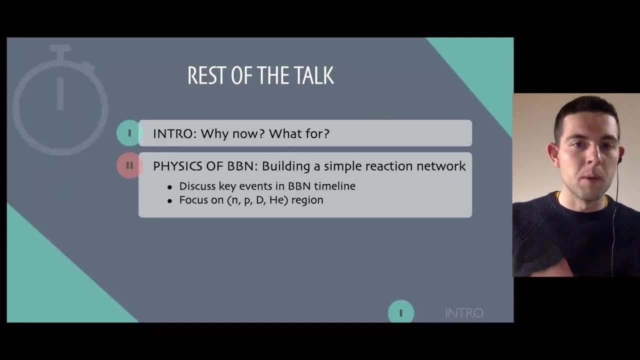 with a reason of. that is where Luna has the, you know, the biggest impact in that regard. And then finally, you know, take some outlook, given that both on Luna, the implications for you know, some of our work, and then just some conclusions and or like recommendations. 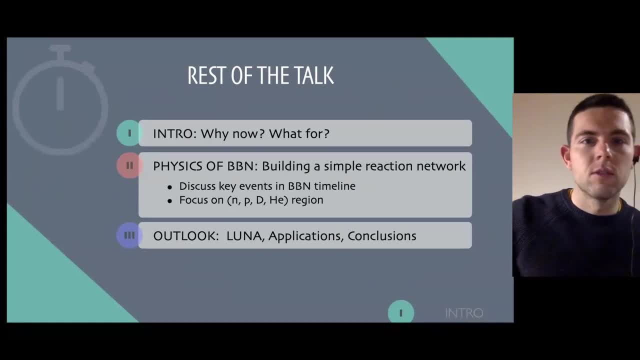 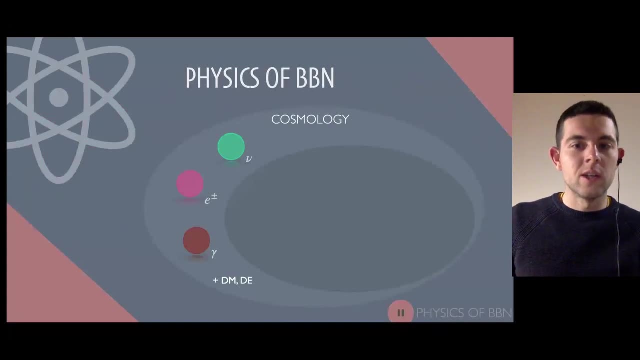 that sort of style, just to just to finish off. Okay, so the physics of BBN: it kind of splits into two parts, parts, I think. So you have cosmology, where you have neutrinos, electrons, positrons, photons, and you also have dark matter and dark energy, although we'll 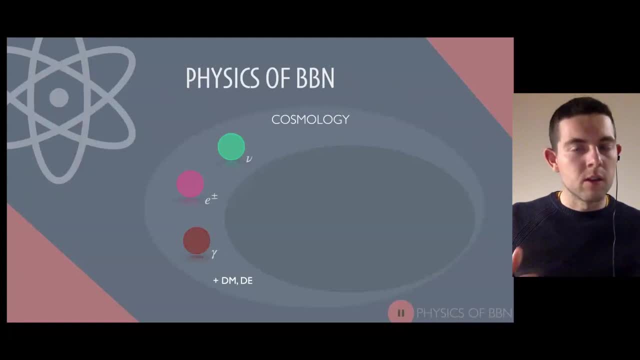 talk in a sec why actually, as far as BBN is concerned, those aren't really your kind of the focus. And then you have this nuclear reaction network, which can typically look relatively complicated, that sits almost within this system. You know you have neutrons and protons that interact, and then you have 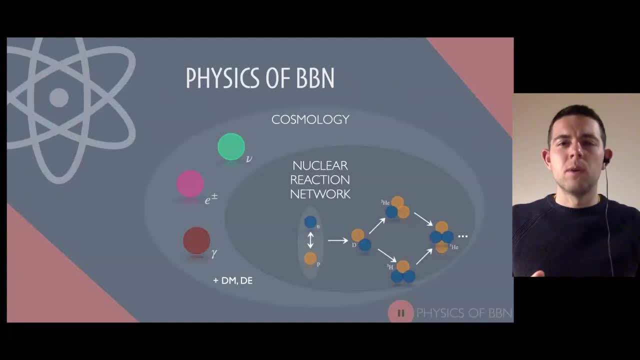 nuclear reaction rates that go into all of this. and somehow you have to put this picture together and solve it in a consistent way. And I say I think on the surface it can look like a relatively complicated system, but there's the following kind of key idea: and the key idea when you are looking to solve for 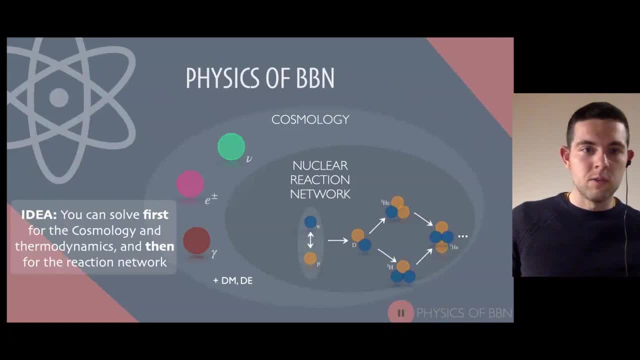 BBN abundances is the fact that you can actually solve the cosmology first and you solve for the thermodynamics, and the cosmology at this time is neutrinos, electrons, positrons and photons dominantly, because this happens during. 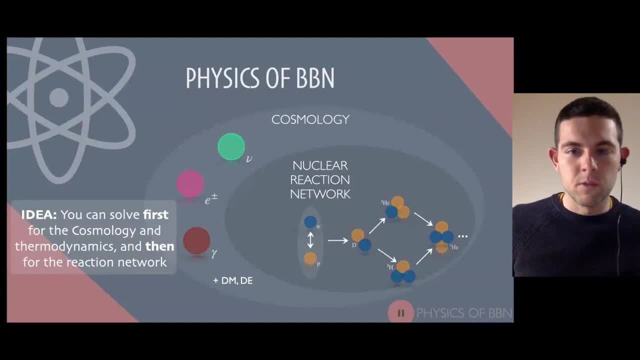 radiation domination, and then you have the thermodynamics, and then you have the radiation, And then you can solve for the dynamics of the nuclear reaction network, almost using your kind of cosmology as like an input into the reaction network. I think you know that's not. 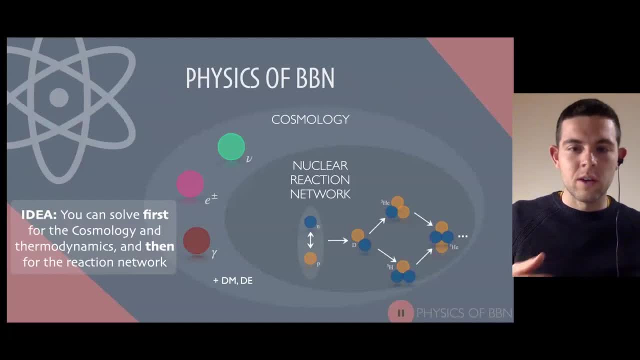 something that's immediately obvious or necessarily true, then in this case it happens because the nuclear reaction network has abundances that are always proportional to, like, a baryon density And in radiation domination that baryon energy density is completely sub dominant compared to neutrinos or 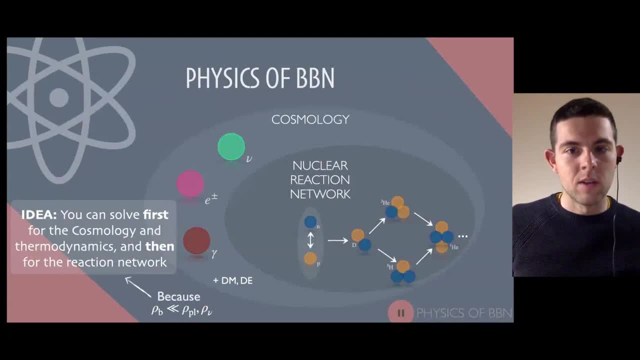 photons, for example. indeed like dark matter and dark energy. you know they are. they are subdominant components like this. feels like i might be asking a dumb question, but rho underscore pl. is that a typo? should that be ph or i should have said that? so i using that to generically describe the plasma. so the third. 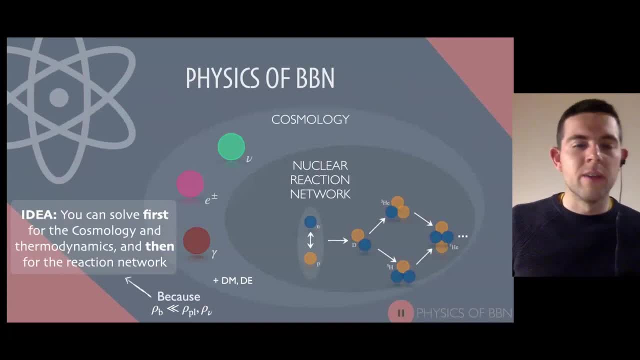 yeah, yeah, i should have said, but yeah, that that's kind of electrons, positrons and photons. i'm being a little bit careful there, because electrons during vbn do go from being a relativistic species to a non-relativistic matter one, so it's not quite true that, for example, baryons are always. 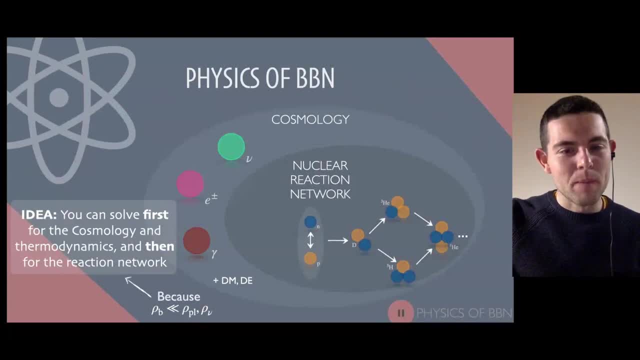 subdominant compared to electrons, but they are compared to the plasma. but yeah, you know it's, i think it's. there's the other non-obvious point about vbn, which is the fact that whenever you see it, you never see a spatial dependence to it, and again, that's the fact that vbn happened. 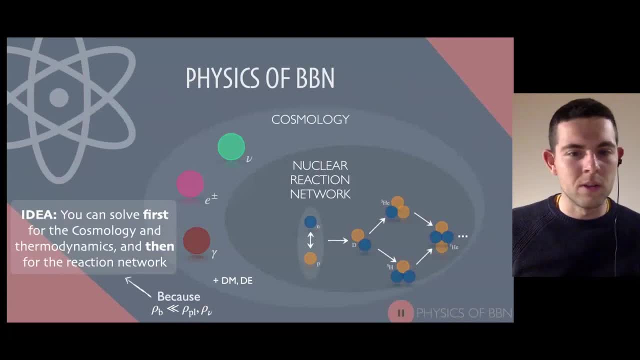 like early enough that all the anisotropies are completely subdominant. compared to the kind of homogeneous description, it's something that you never really think about until you think about it, meaning like: why is that true? you know, the reason is just if i propagate back information from the 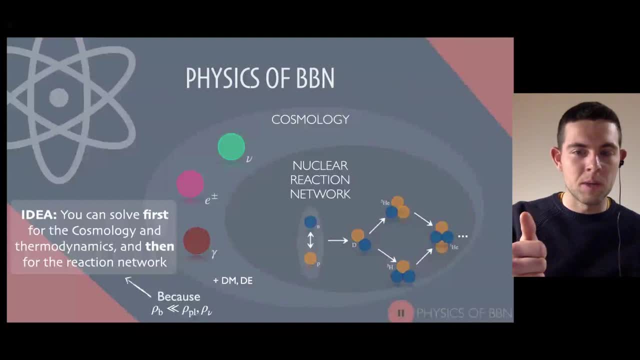 cnb. i can be really confident about these facts that radiation domination is is, you know, the dominant energy density in bbn and that the perturbations are very small. if i was thinking about this from first principles i might have suspected that there were, and in fact now that 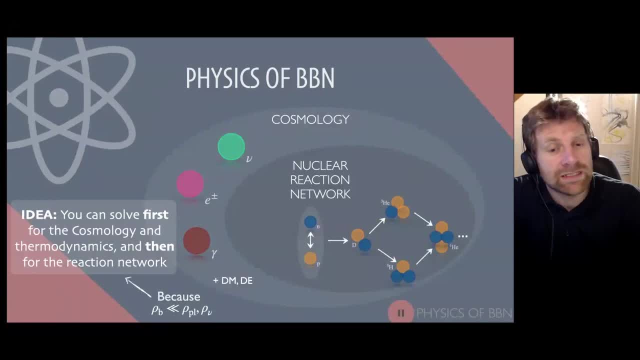 i'm thinking about this. i don't know the answer to the question i'm about to ask. um, not so much that the the like gravitational anisotropies would be relevant, but literally just shot noise in terms of there's not an electron at every single point in space. there's not a proton at 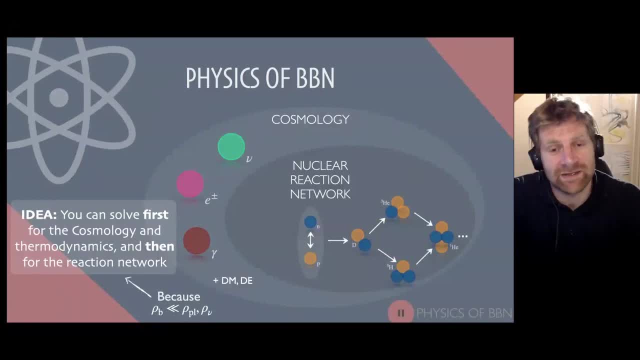 every point in space. so you might get some induced anisotropies because you know there's a proton here and there's not a proton here, and so the reaction right here will be slightly different to the reaction right here, just because there's different, different matter. yeah, so i never thought. 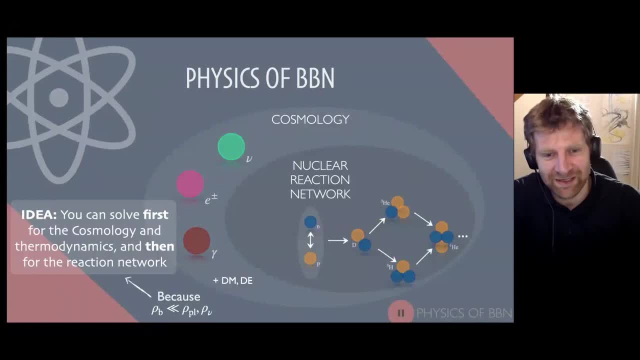 to ask that question before. but why are they not induced anisotropies during bbn? because i know that in other phase transitions there might even be gravitational waves produced, and people talk about that all the time. so, yeah, what is different about bbn you? 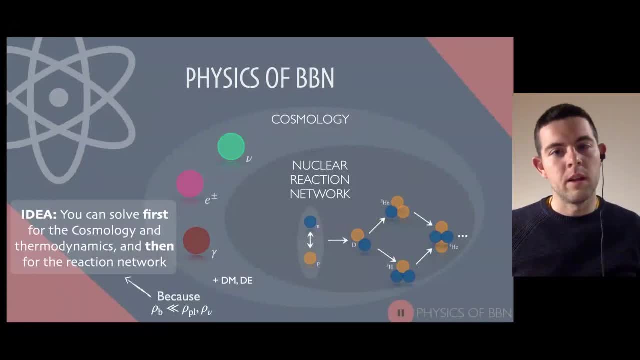 i think it's a statement that, especially when you're talking about the, the electromagnetic plasma, things like compton scattering at this point, are so efficient that you- you know you can transfer, if you want to call it, information. whatever you want to call it, you know you can. 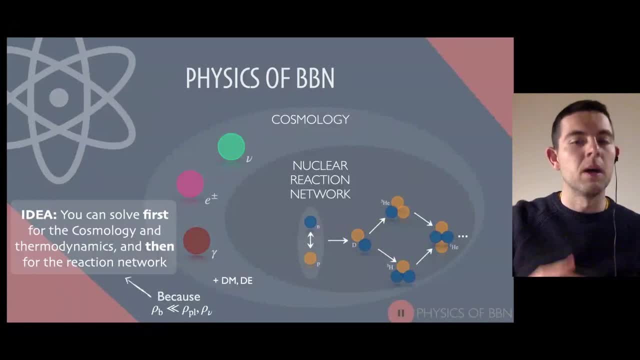 transfer information throughout your pretty dense plasma very, very efficiently and very, very quickly, and that's ultimately why a homogeneous description is is relevant, and the fact that you- just you- have a very thermal system. it does deviate- i'll talk a bit later. it does deviate in crucially from from equilibrium, but in some regards it doesn't deviate too far. 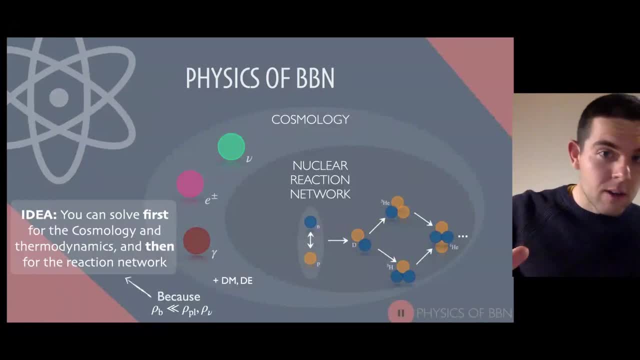 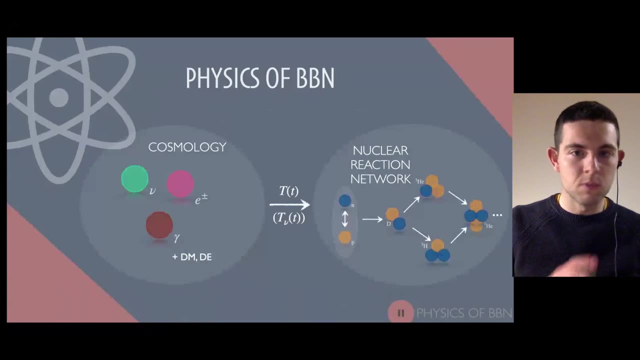 um, right, so you have the cosmology and the nuclear reaction network in principle sits inside it, but it doesn't really sit inside it and really the picture kind of looks a little bit more like the following, which is, you can solve for the cosmology, in particular the dynamics of neutrinos electrons. 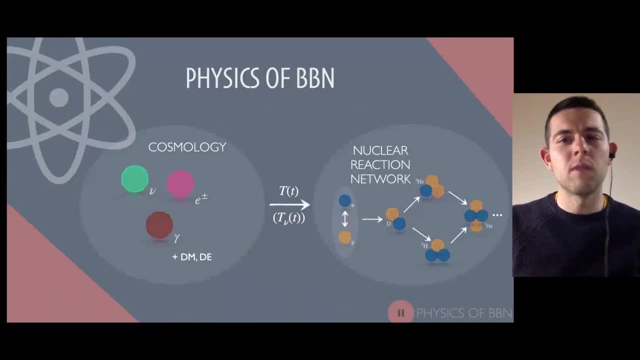 positrons and photons, and really the result of that that you need is a little bit more of a the temperature to time relation. i'm going to emphasize that a little bit more in a sec, but it's a statement that actually many events in the nuclear reaction network occur at, kind of. 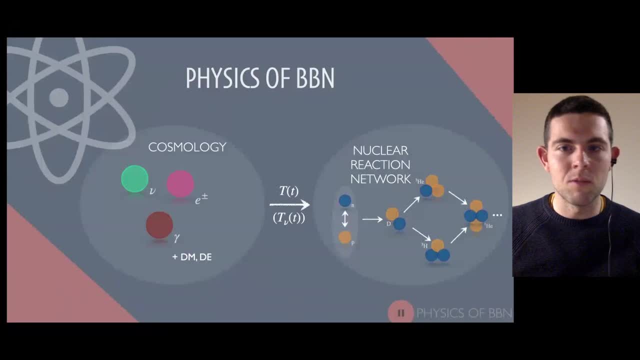 similar temperatures. you know actually not much. bsm physics, for example, even would change when the deuterium bottleneck was overcome. but the time at which they happen is very, very sensitive to the cosmology, the expansion rate of the universe and you know the dynamics of the plasma and actually 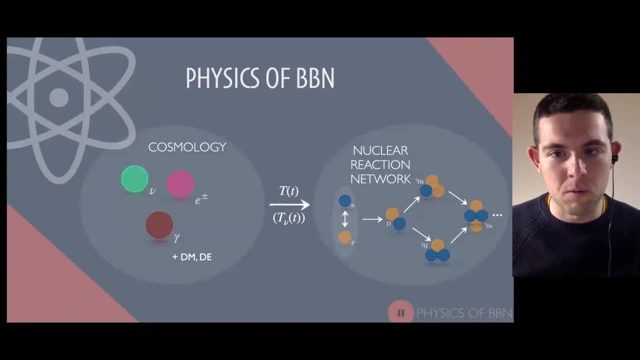 because this nuclear reaction network is very sensitive to the cosmology. the expansion rate of the nuclear reaction network is is out of equilibrium, for example. that means that your, your abundances, your final abundances, are very sensitive to this mapping between temperature and time, and we'll talk about how to, how to get that from cosmology. if you want to go in a little. 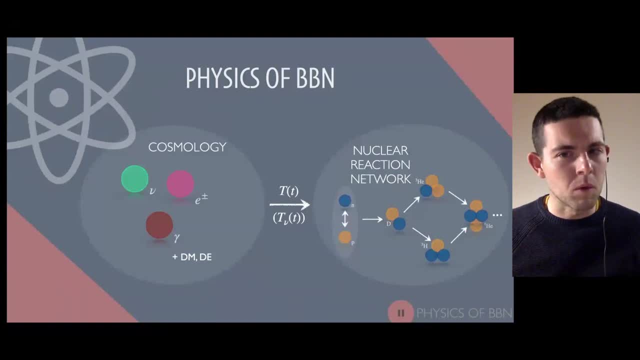 bit more detail, um, and that's why it's in brackets- you also probably want not only the plasma temperature, but you do also want the neutrino temperature too, which is typically not the same as the temperature of the photons. and the reason for that is quite simple: it's because 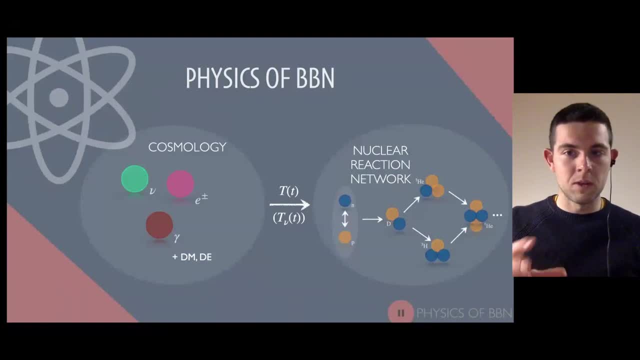 the neutrino temperature is not the same as the temperature of the photons, and the reason for that is because the neutrino temperature and the photon temperature, or more specifically their ratio, typically goes into calculating the weak interaction rates, things that between neutrons and protons, for example. so you do need the neutrino temperature as well, which takes a bit of work. but 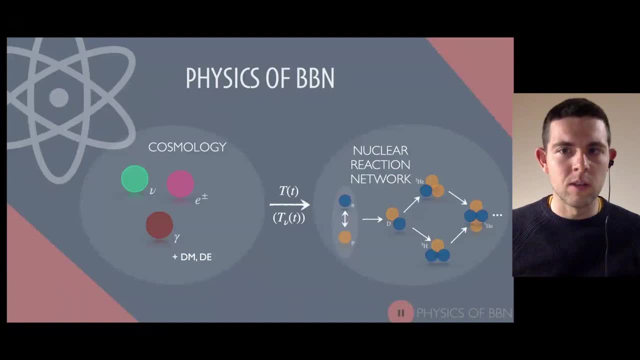 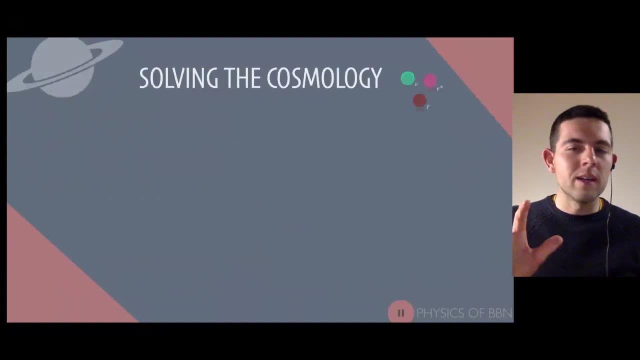 you know, in spirit, what you need is a temperature to time relation that you can then use as initial conditions for for the reaction network. so this is not really the focus, but it is a kind of important enough part that it's worth, um, you know, reviewing very briefly. so how do you? 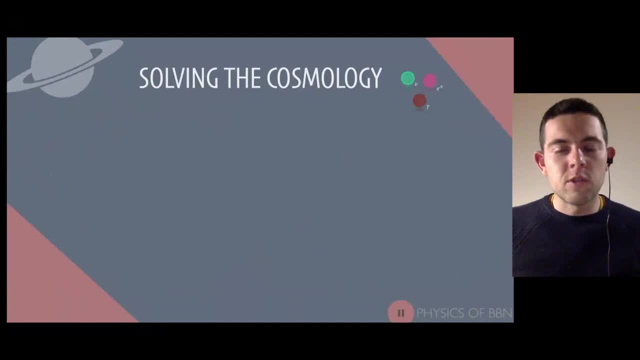 actually go about solving the cosmology. there's kind of two steps, i think, and the first one is to solve for the thermodynamics of the system. so i put in neutrinos, electrons, positrons, photons, and i know the interactions between them, for example compton scattering between photons and electrons. 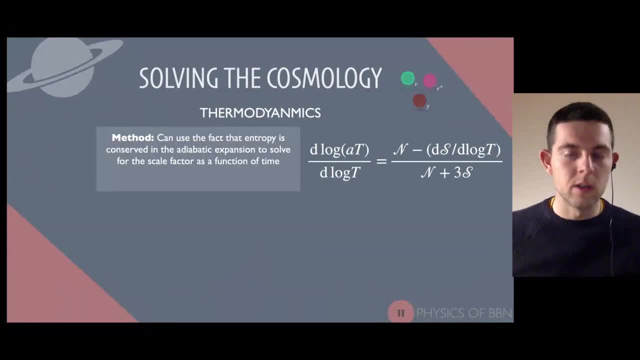 or neutrino electron scattering between. you know the neutrino and electron plasmas and i can use the fact that entropy is conserved in this kind of adiabatic expansion of the universe at this point on the right hand side, you know, i i don't know if you've seen the video on the right hand side. 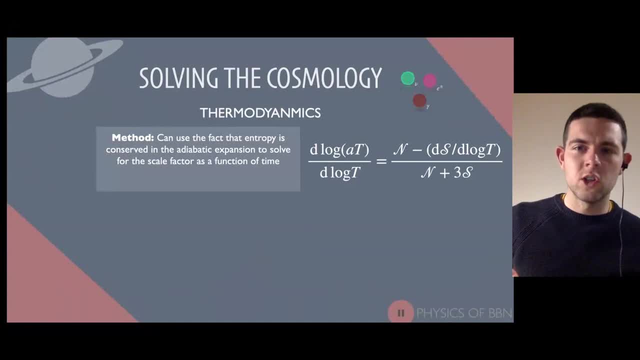 i've flashed an equation- i'm not really going to focus on it here, but it's just to show that you can do a couple of interesting things- and the goal is to get a as a function of t, so the scale factor is a function of t, but this is to kind of highlight what bbn in 2021 looks like. and it looks 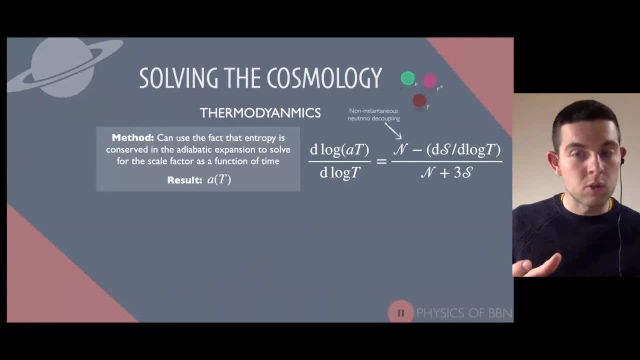 like the following, which is that you can take into account some very non-trivial effects in this plasma. one of the very difficult things to do is to take into account the fact that neutrinos, they do decouple, which we'll talk about in a sec, but they don't decouple instantaneously. 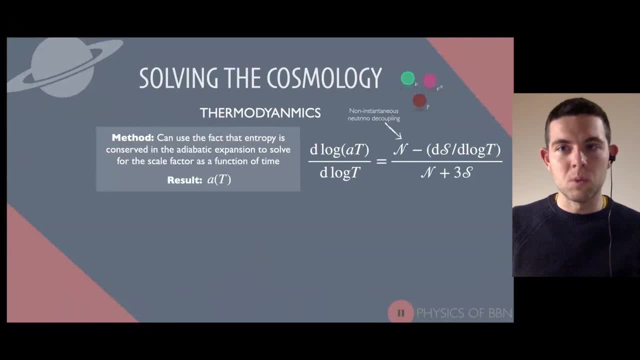 there is some shared kind of entropy between the electromagnetic plasma and the neutrinos and you have to take that into account somehow, and you also have things like plasma effects. so the fact that an electron is sat in a plasma of photons means that it gets some correction to its mass as a function of the 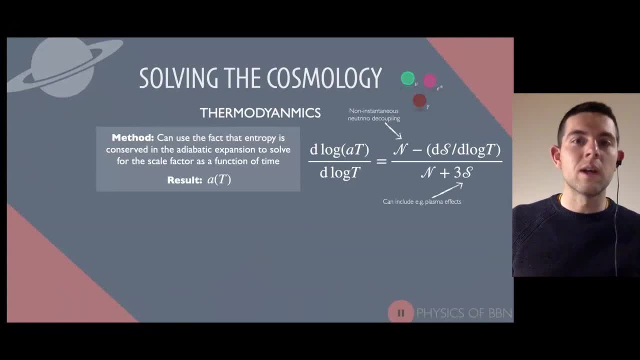 temperature, for example. you know, all of these things are possible to include in the thermodynamics and this is part of this statement. the theory predictions today are very, very precise and they include a wide range of physics, but they do sit at the bottom of the pyramid and they're not. 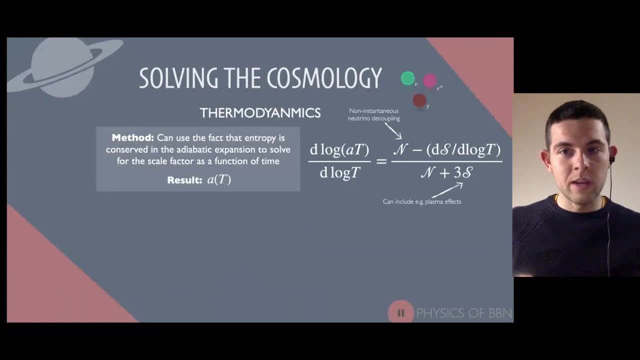 at the level of kind of thermodynamics, and i say ultimately, once they're taking into account. the result is quite simple, and it's the scale factor as a function of temperature. the next step is to kind of then take that and in in the meantime you can also write down the energy densities as a. 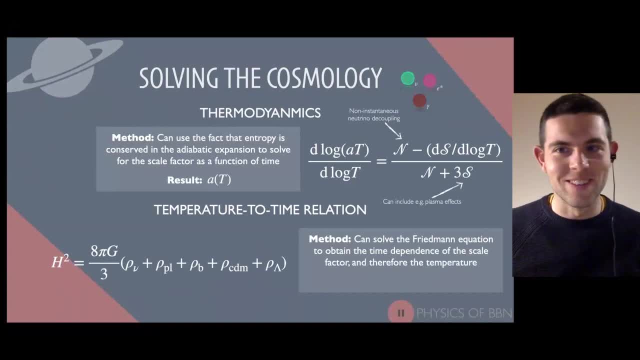 function of temperature. for example, here pl is the plasma, which is gamma plus electrons, and you can solve the friedman equation and really the only only role here is to obtain the following: so you know the energy densities as a function of temperature and solving the friedman equation. 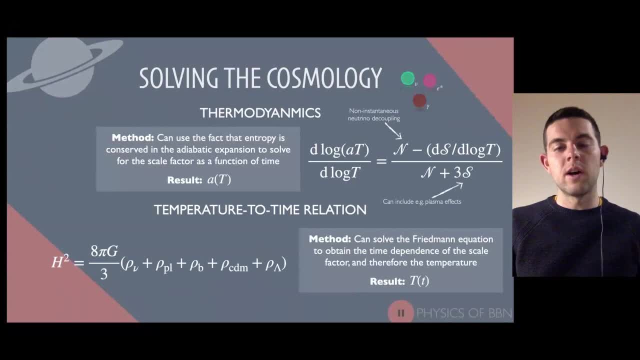 you really are just looking for either the scale factor as a function of time or equivalently, because you know the scale factor is a function of temperature, the temperature as a function of time, and this is, this is your input into into the nuclear reaction network. but yeah, so you know. 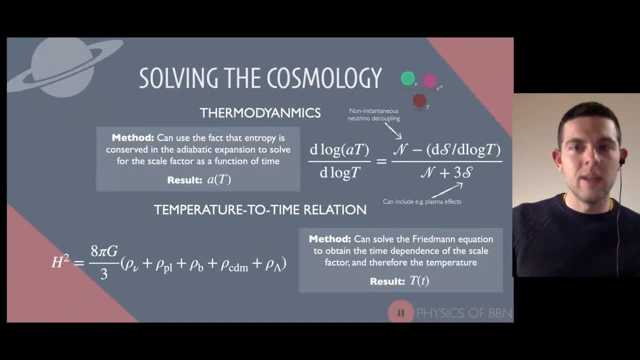 what's the result of this? i say i've kind of put a little bit in in standard model bbn you can move some of these numbers around if you do some, some beyond the standard model physics. but just for now, you know, we'll view this as kind of like a result and the result is this relation, this mapping. 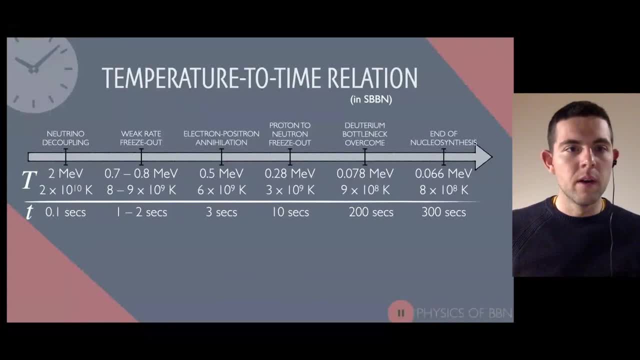 from above the white line to below the white line. so you know you have these key events and we'll go through them shortly. you know we will go through them. they're important both for kind of the cosmological evolution, things like neutrino decoupling or electron positron annihilation. 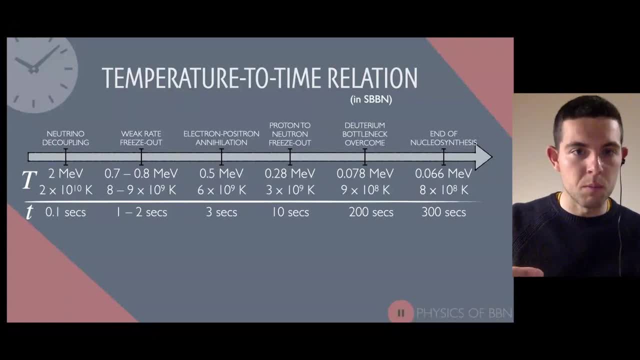 and then, crucially for the nuclear reaction network, kind of evolution of the abundances. but you get this mapping between the temperature at which these things happen, which i say is relatively unchanged depending on what sort of physics you put in, and the time at which they happen. and it's 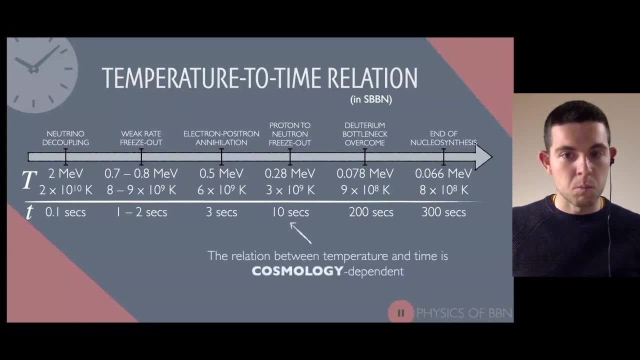 this relation between the temperature and the time. that's actually the cosmology dependence in your problem, and i say we're going to argue later that- because bbn is an out of equilibrium process. it really does know not only about the temperature but it also knows about the time between things. 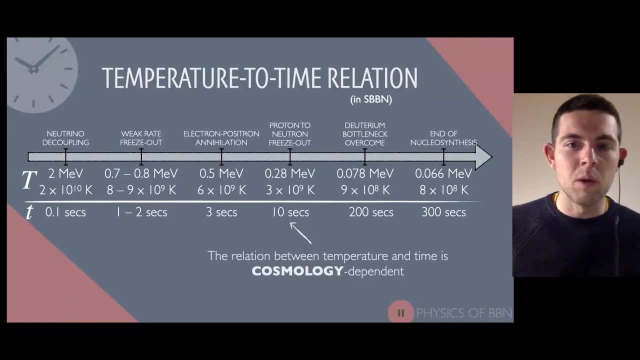 so you know an exercise is worth thinking about. if i look at an equilibrium system, i can tell the difference between an equilibrium system, one temperature compared to another. i might look at like the abundance, for example, of something you know if it drops below its mass, something like that. but i can never tell in an equilibrium. 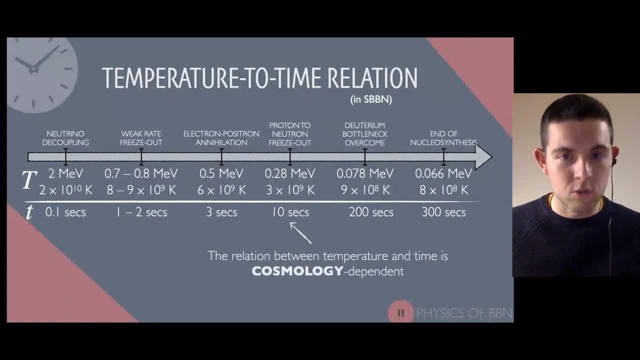 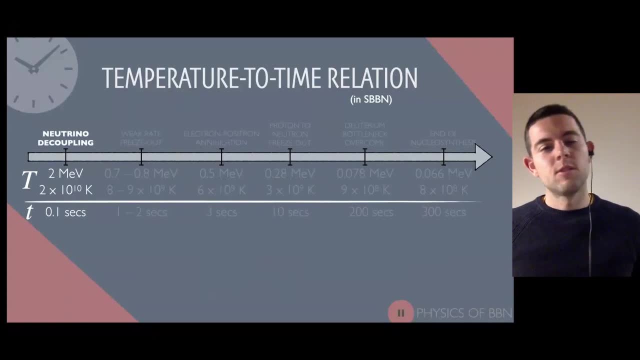 system. how long that process has taken, you know. the same is not true for an out of equilibrium system, and that's this is why the temperature, the time mapping is, is so important in bbn. okay, so, uh, you know, the first important event that comes about in the cosmological 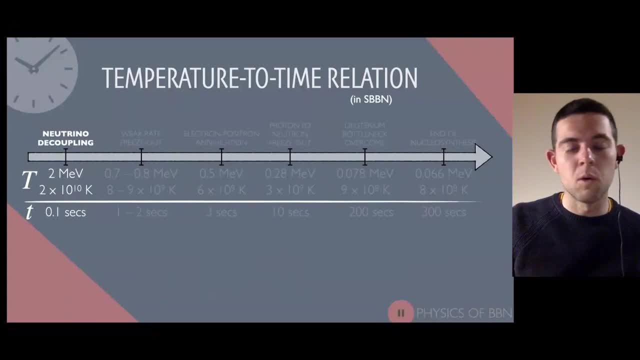 evolution. is this neutrino decoupling, and we, you know, we kind of alluded to it before that at some point in the evolution. um, in particular, as the temperature drops, neutrinos are no longer kind of in contact and they can no longer communicate with the electrons and the photons. it's worth thinking. 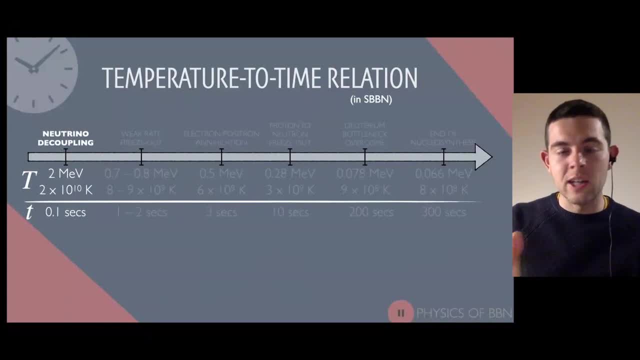 about how neutrinos actually, you know, actually share energy with, for example, the electro electrons and positrons, and it's through these sort of scattering processes. now the rate of these processes scales. it's a weak interaction and it's temperature dependent, like many interaction rates. so it's a weak interaction and it's temperature dependent, like many interaction rates. 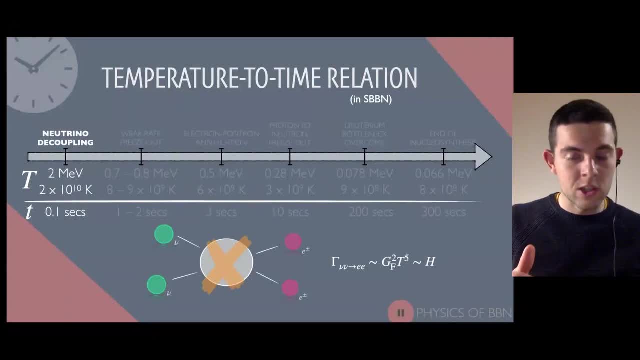 now to understand when this becomes inefficient, we have to think about the hubble rate as well. so all of these interactions are happening in a box that's getting bigger, and as soon as the rate of these interactions is kind of small income in comparison to the expansion rate, they typically freeze out, as they'd say. so we'll use that concept in a bit as well. 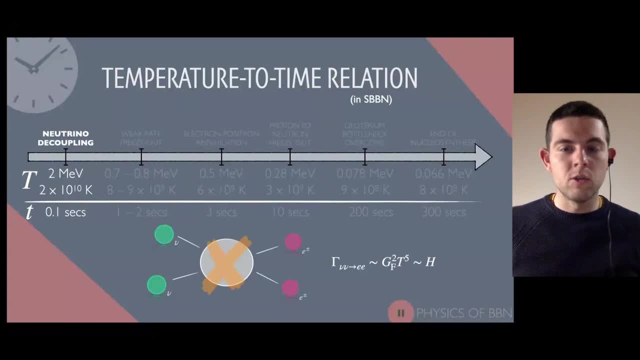 but they freeze out and after this point neutrinos and electrons can no longer efficiently share your energy. that leads on really nicely to kind of the next key cosmological event, which is electron positron annihilation. and this is where um below the electron mass effectively the equilibrium for 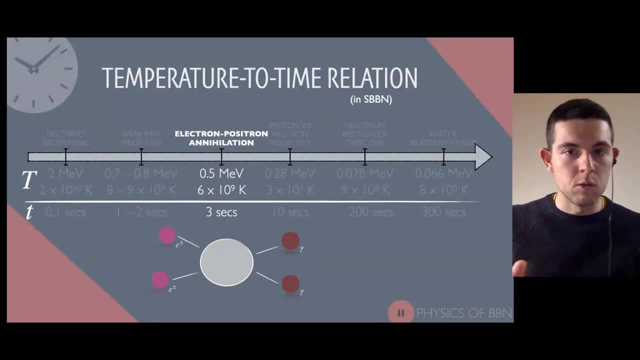 the reaction that's shown- so electron positron pair goes to two photons- shifts really really far to the right, and the reason for this is very simple: it's just because photons that you know thermalize typically just don't have enough energy to pair produce the electron positron. 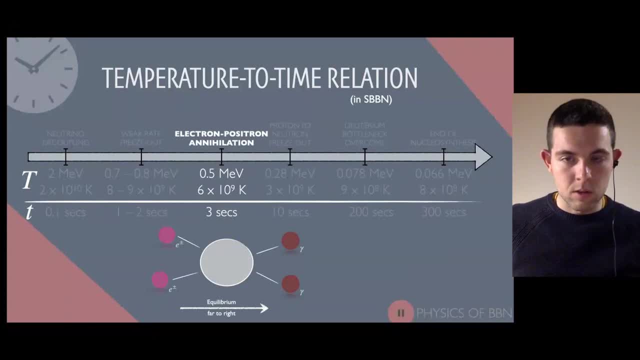 pair, but the the result of this, as far as you know, cosmology and bbn is concerned, is the following: fact that neutrinos- at this time we argued that they were decoupled at higher temperatures- they no longer see this kind of entropy or energy density that comes from the electrons and positrons. 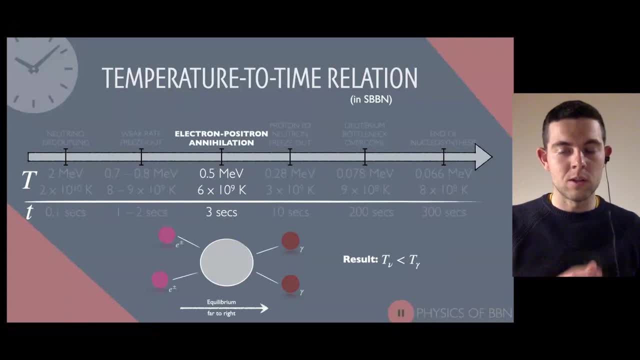 and that means that the photon temperature is boosted, but the neutrino temperature, crucially, isn't. and so, after this point, you have neutrinos that have a a temperature that is less than the photon temperature, and then you have neutrinos that have a temperature that is less than the. 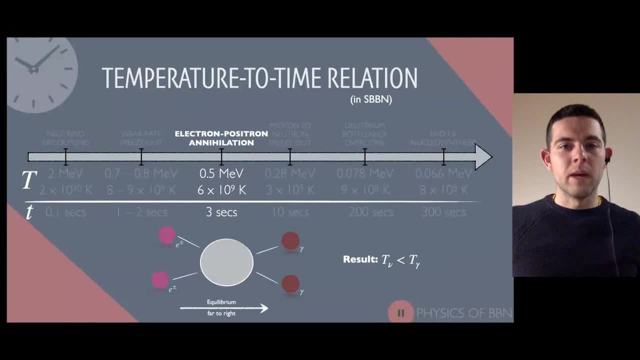 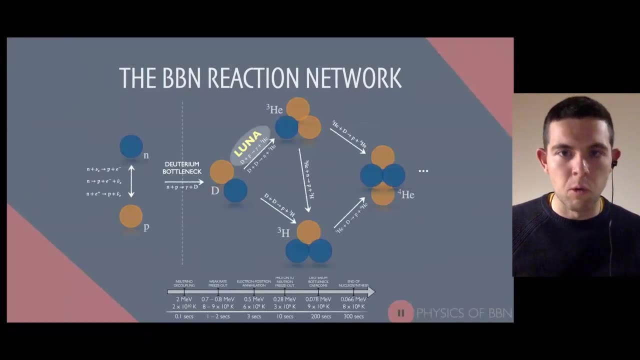 photons. so that's the cosmology out the way. it's now time to kind of go to a relatively complicated, i think, looking reaction network. so at the end of the day, we're interested in using bbn as a probe and we need to understand how you produce things like helium-4 or deuterium, or maybe in the future. 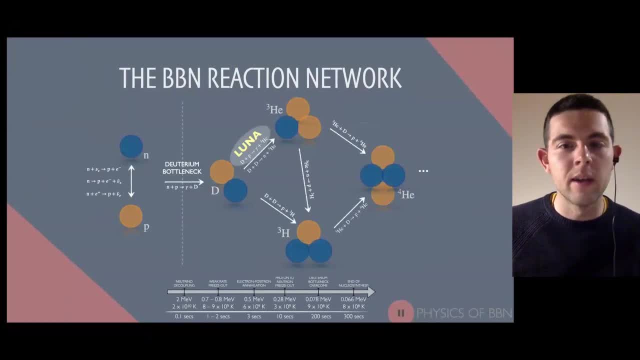 if we have, like you know, good measurements for and things like helium-3. but getting through this reaction network takes a little bit of understanding. fortunately, you know, there are some simplifications, much like the cosmology reaction network split, that you can make to kind of make this process. 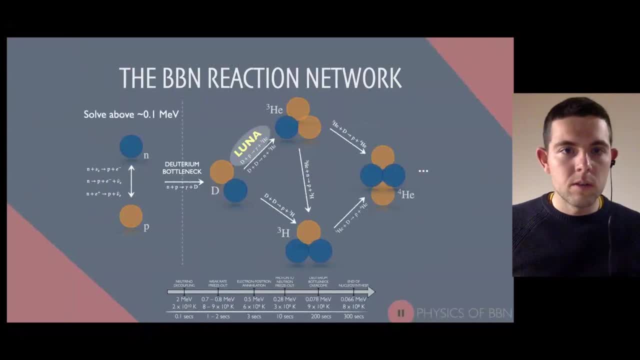 a little bit easier. so the first thing you can do is that you can split the network in two and it's this kind of vertical line, and above temperatures of about 0.1 mev you can solve just for the dynamics of neutrons and protons- and we'll talk about that in a sec- and then below about 0.1 mev, once you've 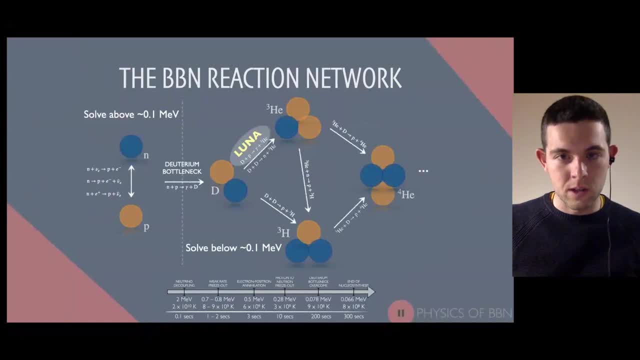 overcome this so-called deuterium bottleneck, which again we'll review in a couple of slides. you can then solve for the kind of full dynamic of you know, the the actual nuclear reaction network, and i've highlighted here, for example, where the lunar rate comes in. so this is just to motivate. why do we want to focus on this little? 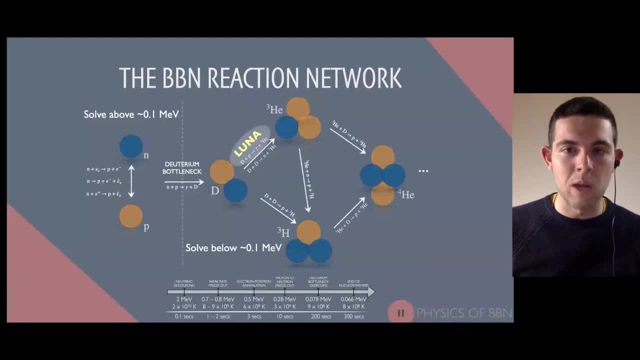 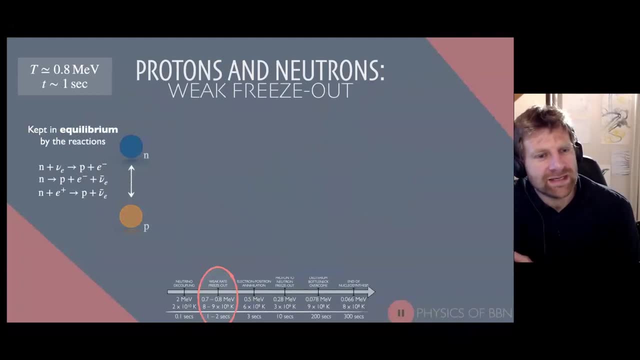 little square of reactions that come about, and it's you know. this is where lunar plays a role. i guess just can i ask one maybe stupid question on that previous slide. yes, it's complicated for me to look at as a human being, but it doesn't seem inherently. 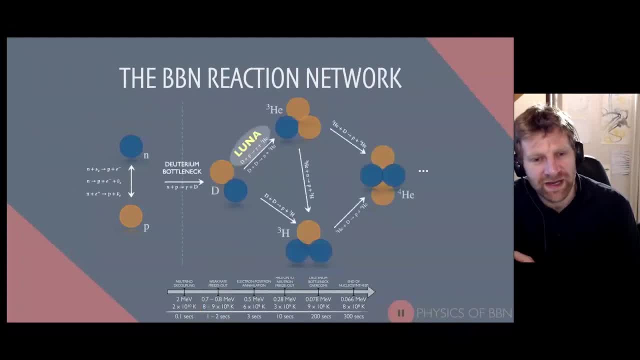 complicated for a computer to just have each interaction rate coded up. so so why? why is it helpful to have this pre-point one mev and post-point one mev split and not just have the powerful computer calculate everything at all times? so i think you definitely can do that. that's definitely an approach with kind of modern, i think, precision. 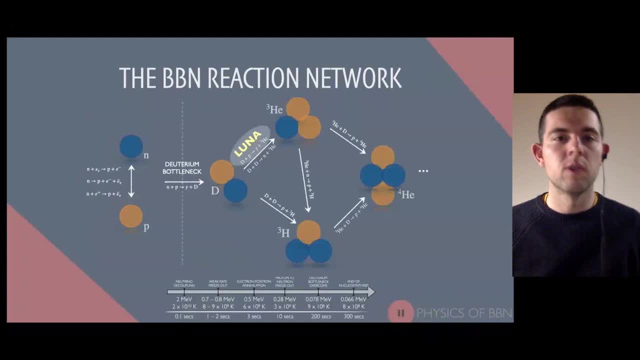 approaches. it's not really beneficial to track the abundances of every single element at all times, but there's no kind of reason for that, apart from computational efficiency. you know, it's just the fact. for example, if you want to track the abundance of lithium-7, 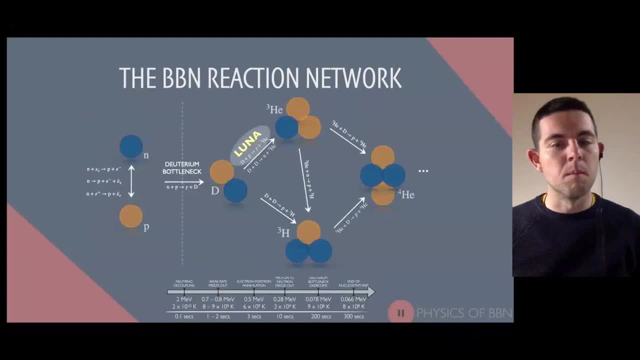 really you don't need to track it until very late on in the process and you can track it, but you're going to find that the abundance is practically zero, complicated i mean in the sense of you know there's a lot of, i think potentially, especially from a theorist perspective, there's that you know there's a lot of kind of potentially unfamiliar. 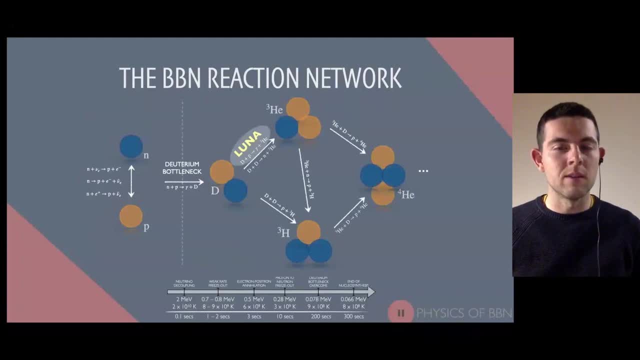 nuclear physics going on here. that's what i mean in terms of complicated and having an intuitive of the dynamics, in particular of the square part of the network on the right hand side of the line. i think that's challenging even for kind of like people who are familiar with the different. 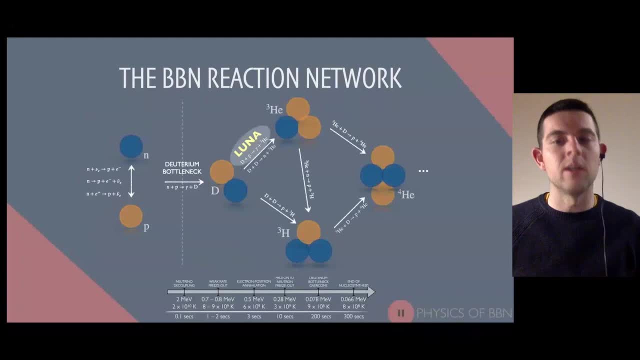 reactions, so like predicting how much you know intuitively, how much tritium, for example, i end up with. i think that's quite a complicated task, so i say you can solve it above 0.1 meb and below 0.1 meb. so we start off with this kind of simplified neutron proton system. so again, there are a couple. 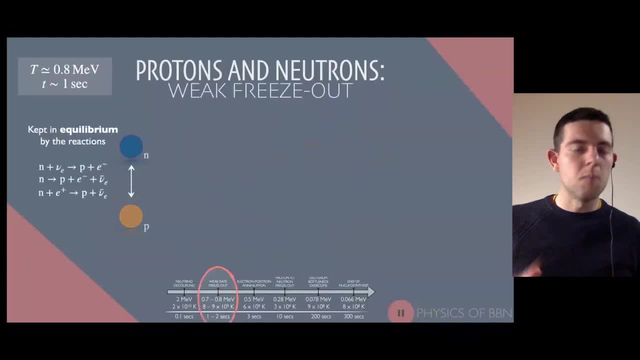 the first one is at temperatures typically above kind of 0.8 mev say before, kind of one second. at that time neutrons and protons are in their thermal equilibrium abundances, and the reason is because the three reactions there are very efficient at interconverting. 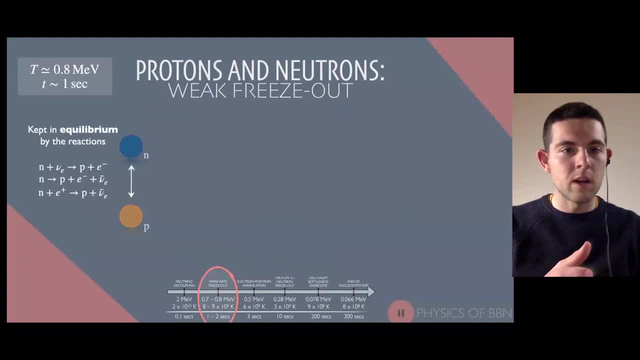 protons and neutrons, you know, said in the way of neutrino decoupling. the rate for these reactions is is much higher than the hubble rate at this time. but this is not always true. and actually until around 0.8 mev this is true, but then it you know these, these reactions fall out of. 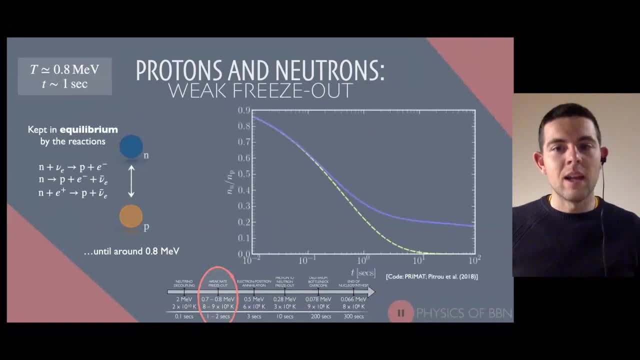 equilibrium, and the following plot highlights that a little bit. so we're looking at the the neutron to proton ratio and the yellow dotted line is the kind of equilibrium abundance that you would expect if, if these reactions were very, very efficient and if you want to, you know, think about. 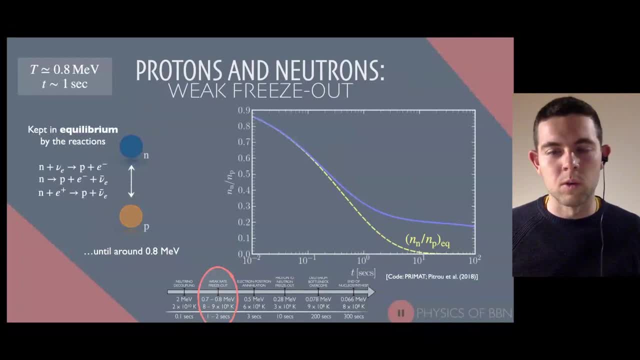 that for a little bit. this is probably a good thing, because otherwise we'd end up with no neutrons to kind of make helium out of, so that we kind of needed it to go out of equilibrium. but this is the actual abundance that you see, and i say it's simply for the reason that those 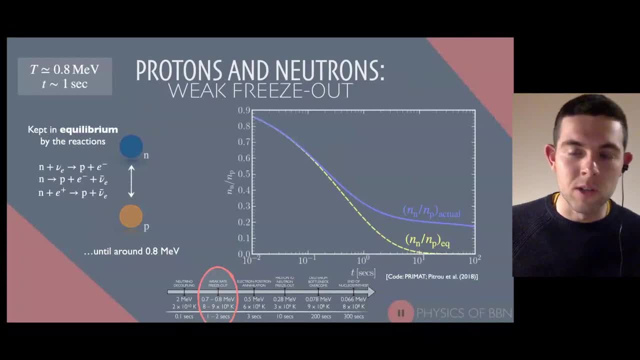 reactions that inconvert proton and neutrons become pretty inefficient at some point, and it's around this kind of temperature here, this, this time of kind of 0.1 to 1 seconds, that this, this, this tends to happen. but this is not the end of the story for neutrons and protons. 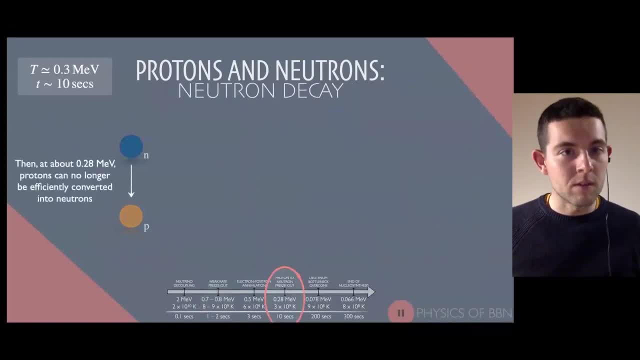 and if you drop the temperature a little bit further or wait for about 10 seconds into into kind of the the early universe evolution, then it actually turns out that not all of the neutrons are very efficient, and not only do the reactions kind of fall out of equilibrium, but 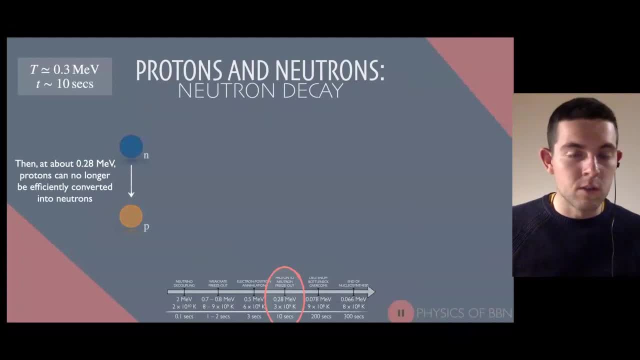 actually the the kind of backwards reaction of protons being converted into neutrons is not is not very efficient and actually below these temperatures the only process that can really happen is neutron decay. so that means that until you get to this point which we're going to talk, 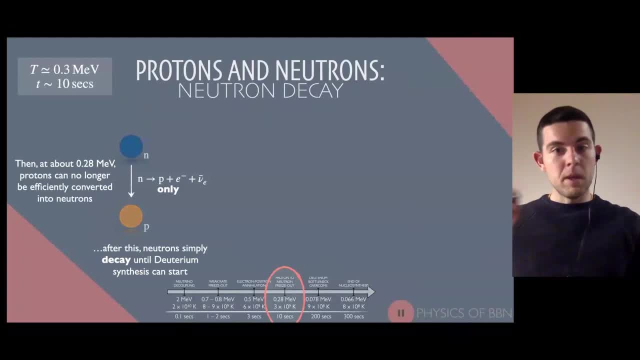 about in a second. really, the only thing happening in the whole bbn nuclear reaction network is that neutrons and protons- which set the abundances, kind of that we saw on the previous slide- and neutrons just decay, because that's the only reaction that's actually kind of relevant at these. 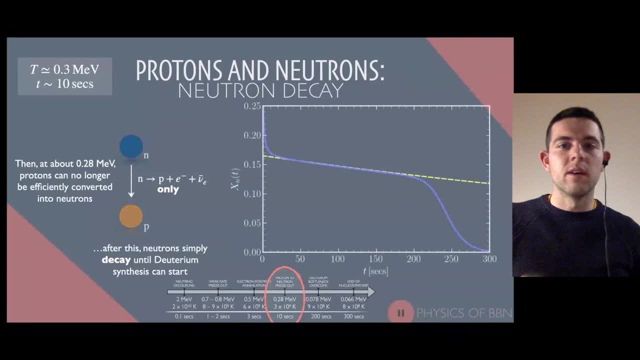 times and you can kind of see that here. this is just tracking the, the neutron abundance, and this yellow dotted line, you know the blue is just the neutron abundance, or you know, in particular compared to baryons, but just in the neutron abundance and this is the abundance of neutrons. 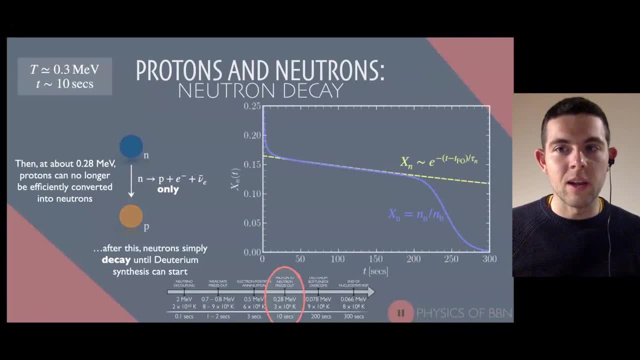 if you just let it decay with some decay, decay lifetime tower. so you know, you see, after this kind of 10 to 50 seconds, for a good chunk of time, about 150 seconds, the only real dominant process that's going on is neutrons are just decaying into protons. so you know. 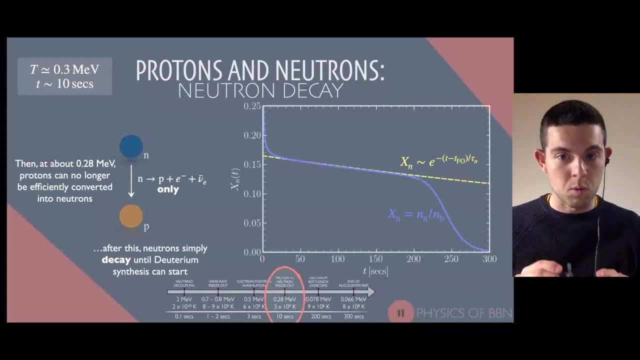 you're. if you let this run on and nothing else happened, we're going to talk about what else happens in in two seconds. if nothing else happens, the neutrons would eventually just decay away and the only the only baryonic component you'd be left with would be protons. and i said, you know, in this: 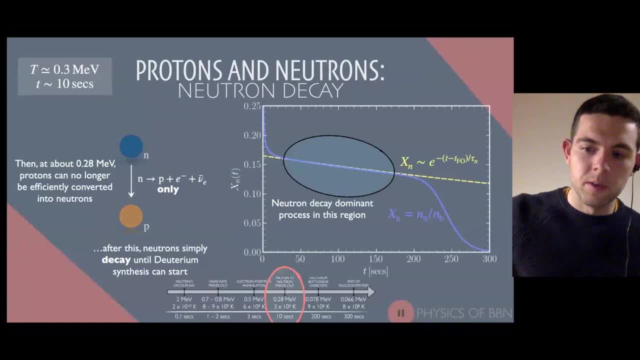 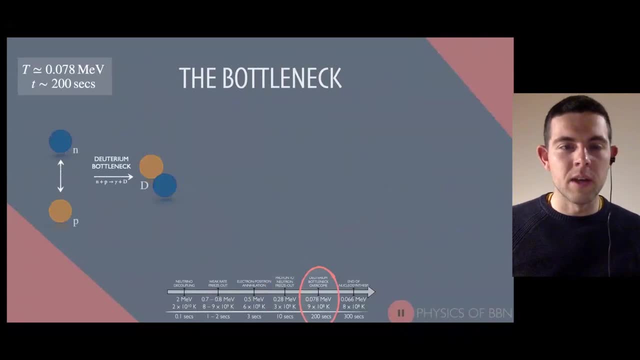 region. the neutron decay really is the dominant process that's going on, but fortunately something does happen. otherwise, you know, there would be no way to end up with the the heavier elements, and the idea is that we have to get over this so-called deuterium bottleneck. 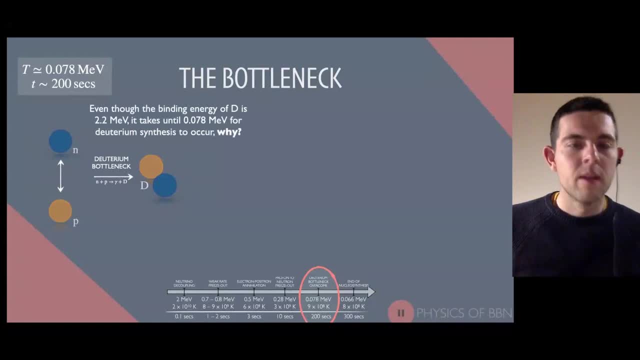 deuterium has a binding energy of a couple of mev and that means that you know, below that temperature it's kind of energetically preferential to make deuterium out of a proton and a neutron. it's better to be on the right hand side of that equation, kind of from an 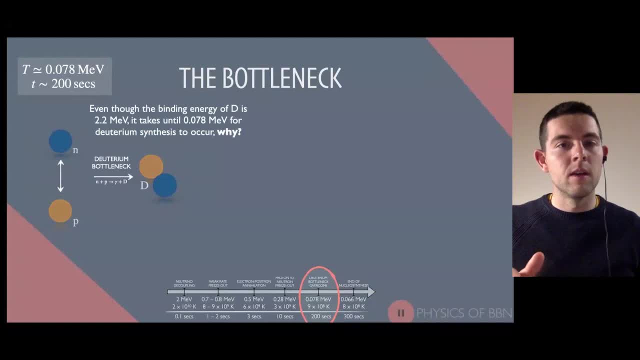 energetic view. but if you actually look at the evolution which i'll show in a second, you really have to wait until temperatures kind of, you know almost kind of a factor of um, what's that factor of kind of 50 smaller, to actually significantly produce any deuterium. so the question is why? why? 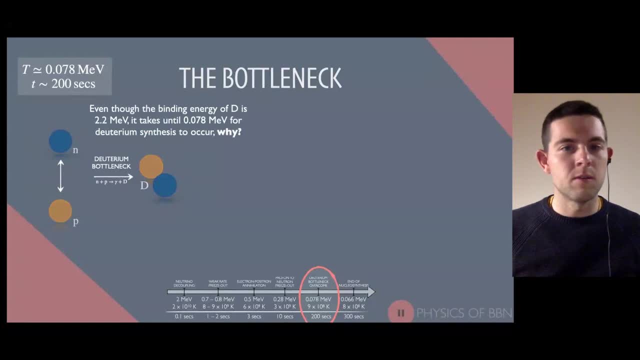 does this happen? and the answer is photons, and the answer is the fact that there are way more photons than there are baryons. so at a typical energy of, say point, you know, 0.1 mev, the average photon does not have enough energy to kind of dissociate the deuterium. however, there are about 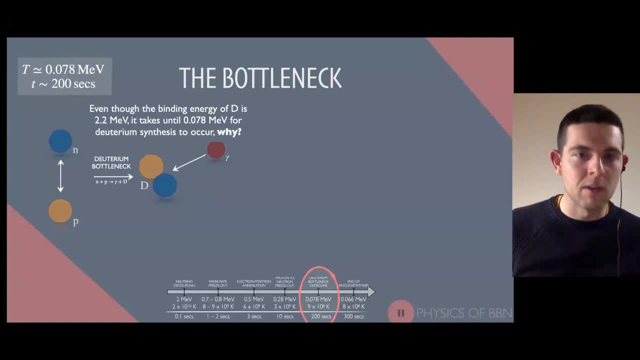 10 to the 9, more photons than there are baryons at this point. so it means that even though the kind of average one doesn't actually the tail of photons, which is where the capability of kind of dissociating this is, you know, the ones that are in the very, very far end of the kind of whatever. 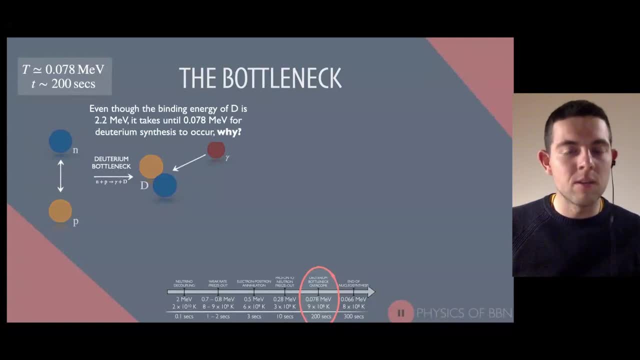 kind of distribution you're considering. um, there's still plenty of them around and this is ultimately the reason you know there is. even though the average photon doesn't have energy, there are still plenty of them as kind of parameterized by this baryon to photon ratio. 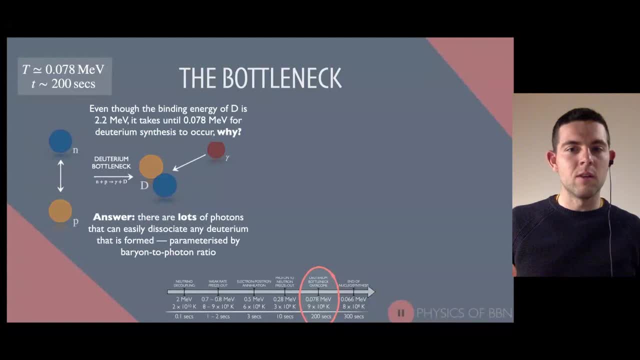 and you know this is this is the fact that deuterium synthesis is kind of delayed compared to a couple of mev is excellent evidence for a very, very numerous that you know, uh, thermal bath of photons around this time. if, if that was not there, if, if the baryon to photon 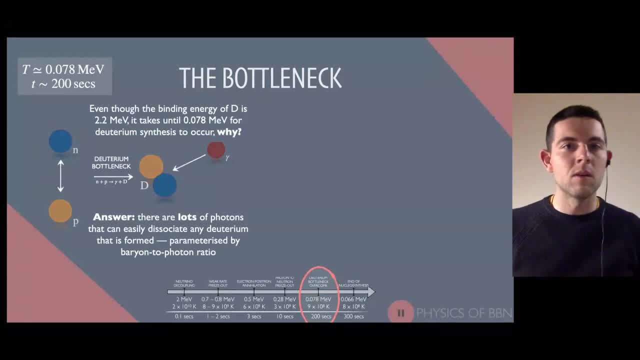 ratio was one. for example, you know, there was one photon for one baryon deuterium could be produced at two mev without any any issues. if you wanted a quick way to estimate where this 0.78 mev is, the thing that you might do. 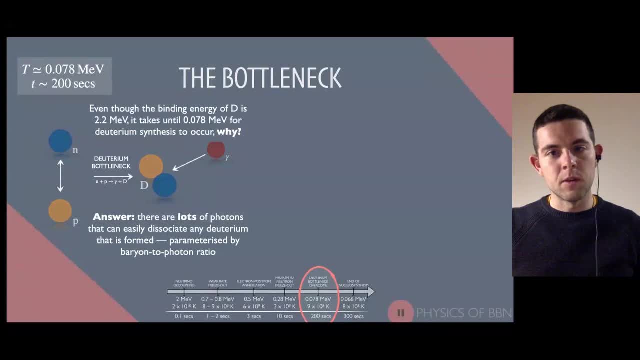 for example, would be to integrate the number density of photons with a, with an energy above 2.2 mev at a given temperature, and compare that to the number of baryons, and you're going to find that, you know, you typically get this factor of something about about 50.. and, and that's the point, 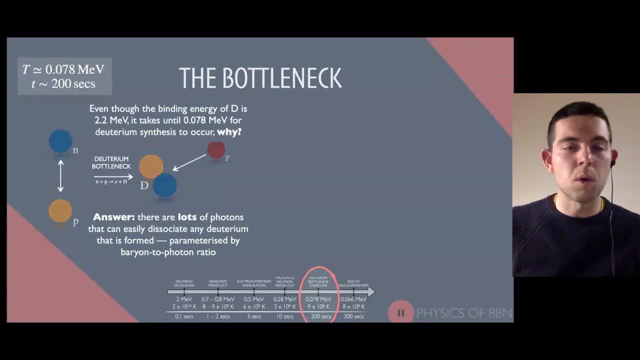 at which deuterium can then be, you know, synthesized. the problem is not synthesizing it. this is the point. protons and neutrons are more than happy to make deuterium at this point, just from an energetic viewpoint. the problem is, once you make it, you don't keep it. so to kind of see how that actually. 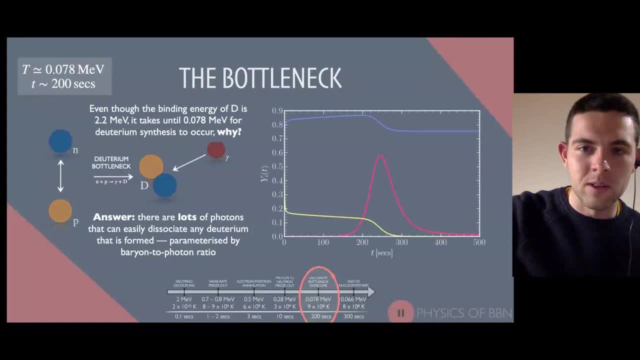 goes ahead. you know, here are some the kind of the evolution of the abundances. so the yellow curve is is is just the neutron. so we kind of saw the evolution of that. and the top curve is the is the protons. so in this intermediate regime where neutrons are decaying, you see that. 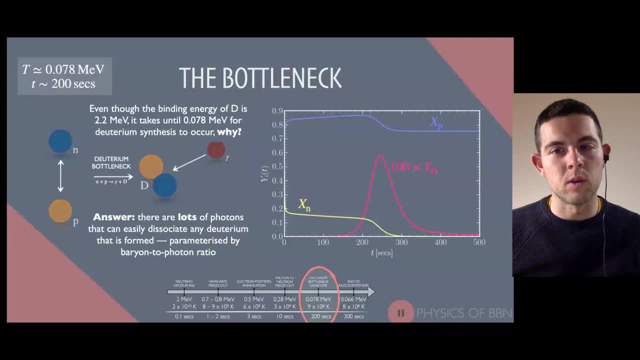 protons, just if they just decay into protons. so the proton number density just increases in exactly the same amount that neutrons decrease. but then eventually you get to this point about 200 seconds or about you know, 0.078 mev, where suddenly you can produce deuterium and i you. 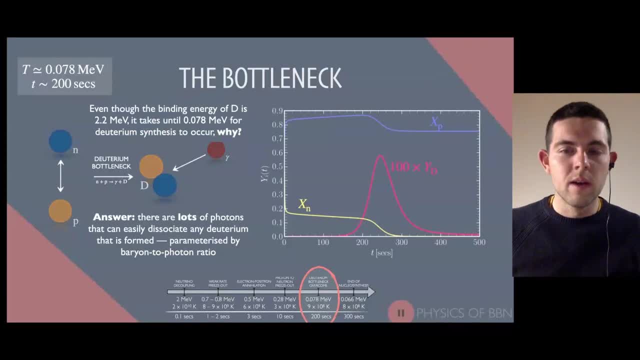 know, i've kind of scaled it up a little bit just to kind of make the point. but you see that very, very quickly the production of deuterium ramps up and then it's used up again and we'll think about what happens to it in kind of the next slide- and i say it's only after this point, about 200 seconds. 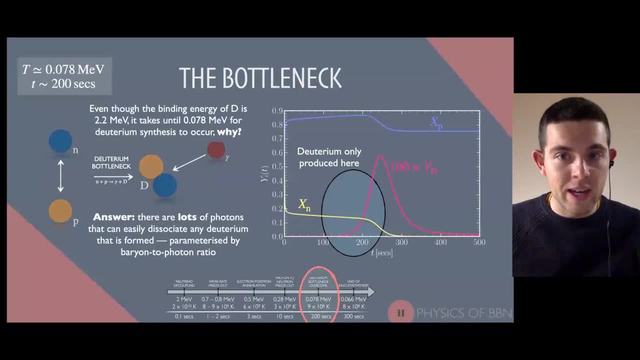 that you really start to have a dominant energy, to have a dominant production of deuterium that actually hangs around for any reasonable amount of time, and that's exactly what you need. some people call deuterium a kind of catalyst, so you create it and then you use it up to go further, you know. so it's not like. 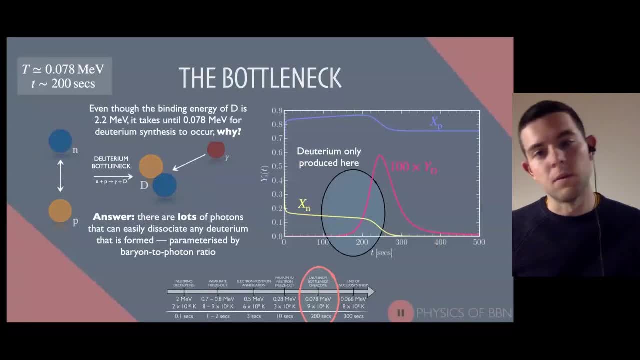 it stays around, but you, you do need enough of it in order to move further on in the network. so we're finally at the point where we start to see again luna, but also we have enough deuterium to really start thinking about the dynamics of 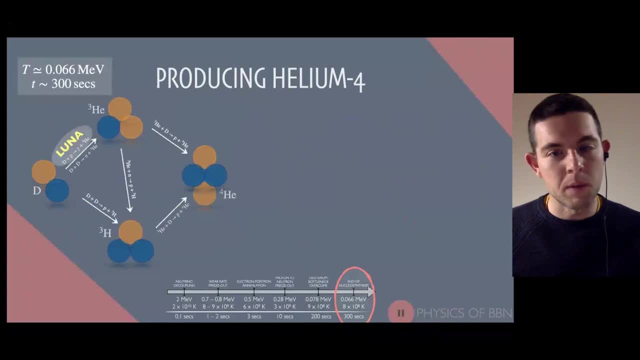 this kind of square part of the network and, crucially, where you end up with something like helium-4. so this kind of proceeds as soon as you have plenty of deuterium and because the binding energy of helium is so high, so it's about 28 mev. that means that these temperatures of you know, 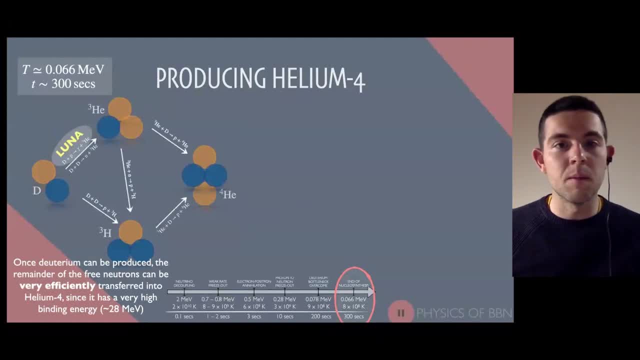 0.05, 0.06 mev. once you make helium, you know the backwards reaction rate is actually very small. it goes like something like e to the minus binding energy divided by temperature: 0.05- 0.07 mev. so you can see that this is a very good reaction to go to this 4-helium state. 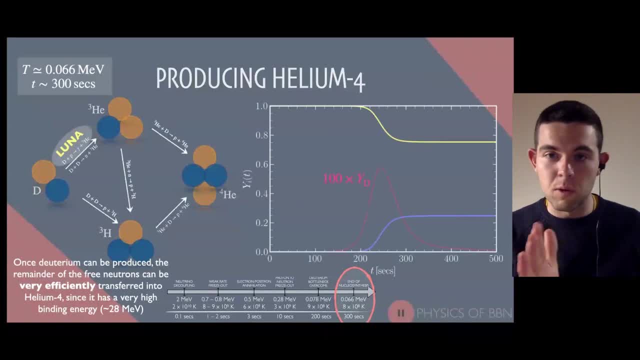 is is very much preferred. and in terms of abundances, you see the following. so i've just- you know, there's a deuterium, just to give you a reference point for some time. here's the neutrons plus protons, so the sum of those two abundances here's the 4-helium and this shows you basically. 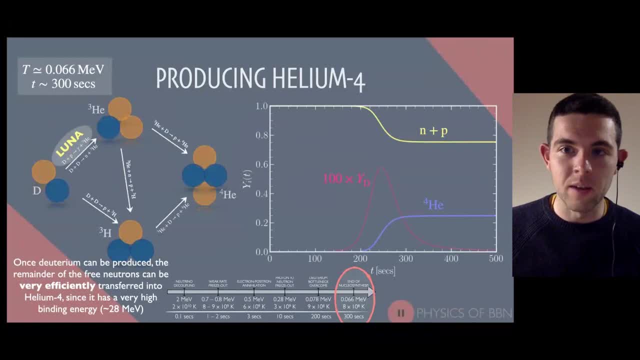 that all of the neutrons and protons. you use up all of the neutrons that you can and they all go into kind of 4-helium, that effectively 4-helium. i think now it's worth taking a thought and i've kind of just said: oh, you use up all of the. 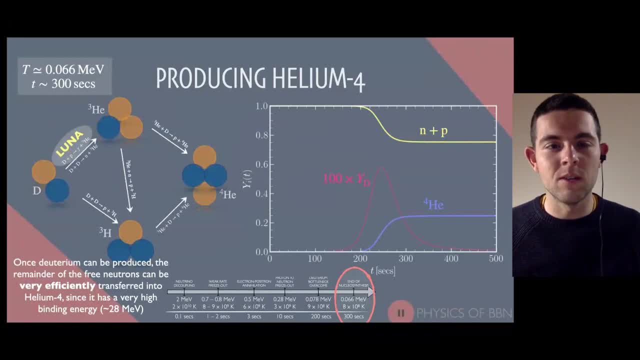 neutrons and it's super efficient and make 4-helium. and then you, you ask me the question of: but isn't luna measuring deuterium rates? so why are they so important? i think you know this is kind of the next step and this is the step of doing precision. bbn 4-helium is, you know, very. 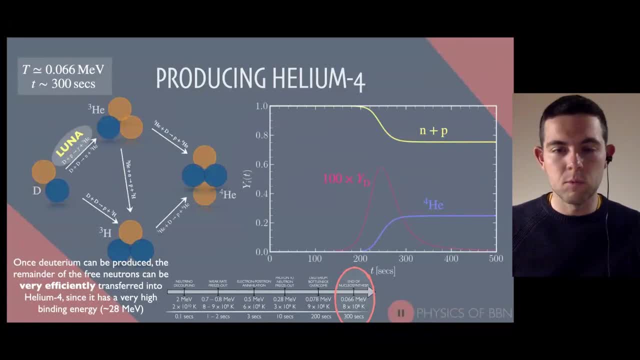 much the dominant abundance for basically any realistic model of bbn. but deuterium 3-helium tritium are still produced in trace amounts and we can actually measure those trace amounts. this is this quasar gas cloud system. that's the importance of that is the 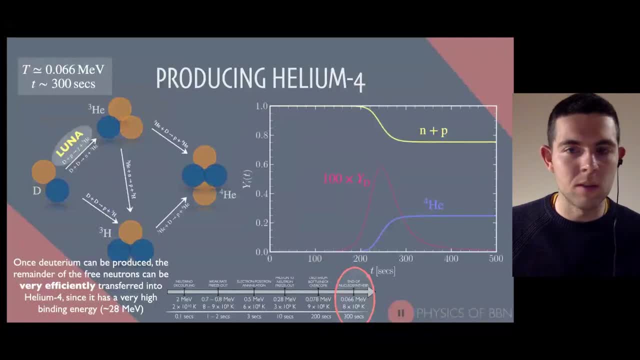 fact that, even though the abundance of deuterium might be five orders of magnitude below that of helium, it's still a very relevant abundance for understanding the dynamics of the bbn network. the one question that maybe i would have would have asked: why is it that direction? that was the 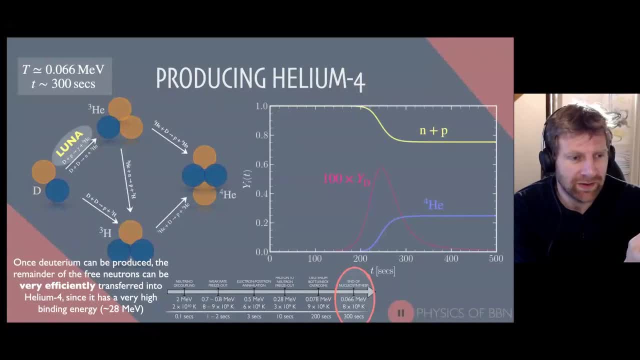 one that was needed to be measured, to be better measured, and not the d to 3h direction, but but maybe it's just that that is an important thing to measure and it hasn't. it just needs to be measured better, i don't know. yeah, no, so i mean, it's a good question and i kind of touch on it a little bit later. 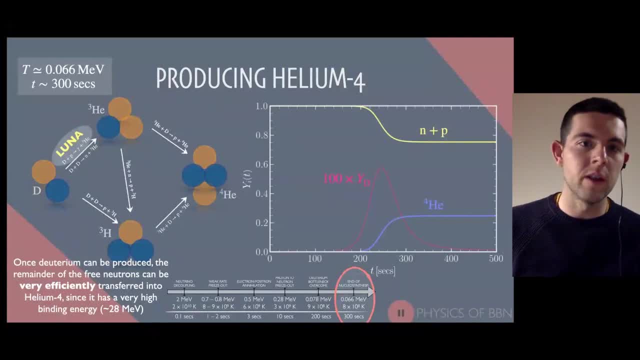 the answer is that the three reactions that you see that if we just think about deuterium for a sec, you do have to worry about the others. but if you're just worrying about deuterium- and the reason you might worry in particular about those- is because deuterium is the element that you also 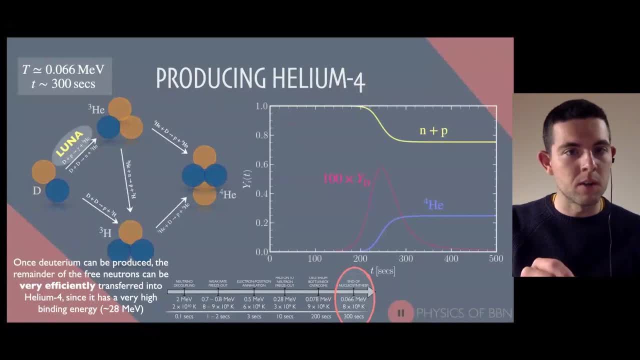 have the very good abundance measurement, for you don't actually have great abundance measurements for helium-3, for example. so actually the two, the two on the furthest right. you might not be so kind of concerned about measuring super well, but you are really concerned about measuring those. 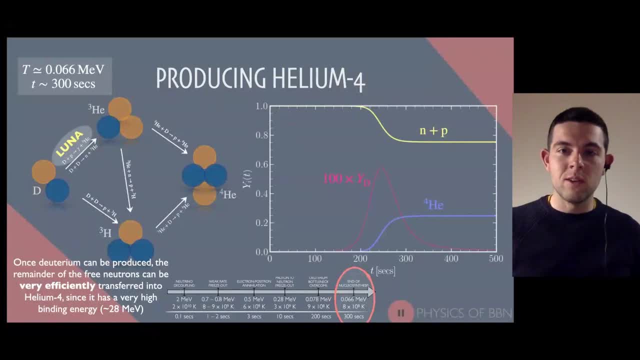 three and it turns out that the status kind of pre-2020, pre-lunar, was. you had those three reactions, so d plus p goes to gamma plus three helium. i'm going to, like you know, enumerate them because i think it's a good idea to do that. but i think it's a good idea to do that because 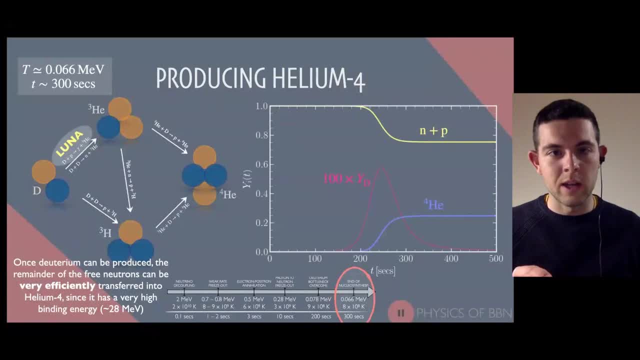 it's kind of useful. deuterium plus deuterium goes to neutron plus three helium, so they're the two on the upper arrow. and then deuterium plus deuterium goes to proton plus tritium. now you have those three reactions and you have some uncertainty, some like measurement reaction rate. 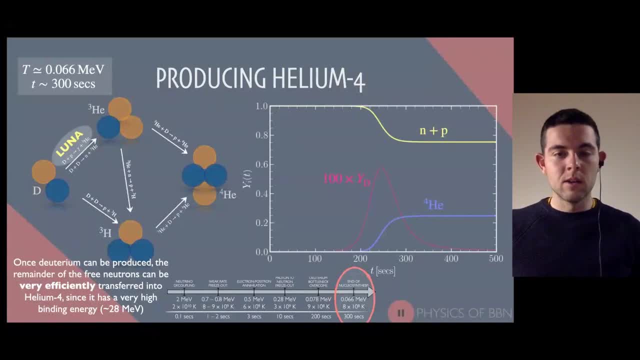 uncertainty associated to them which gets propagated to your prediction in the deuterium abundance and it turned out that kind of pre-2020, the one that lunar measured. there was the absolute dominant theory, uncertainty. so the answer is that the others were just measured better than the one that lunar measured. so you know the reason why lunar is so important. 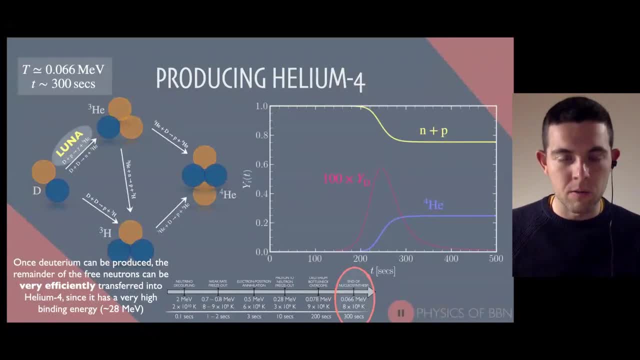 is because it reduced basically the theory error in that part of the reaction network by a factor of about kind of i think it was a factor of about 10.. were lunar directly trying to improve big bang nuclear synthesis or or is there some other reason why nuclear physicists care about this particular? 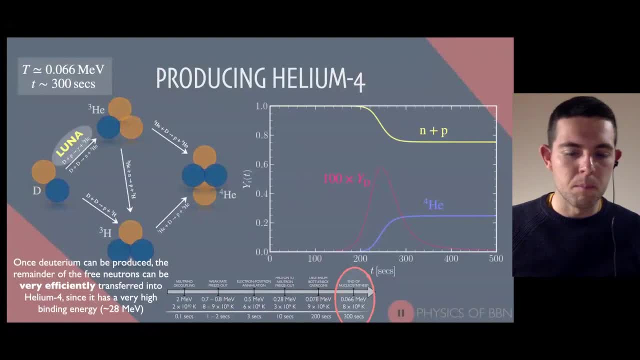 reaction rate. i'll show the lunar plot in a second. but the energy range that they, you know, really focus a lot on is the energy range that they're trying to improve and they're trying to improve the effort into measuring was exactly the vbn energy rate, you know. i think it's a quantity that 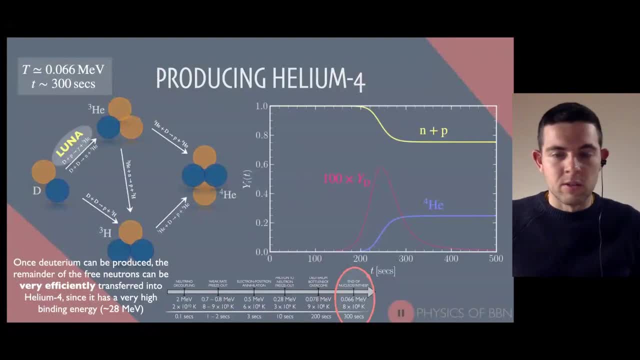 of course is is useful to know regardless because it's a, you know, a standard nuclear reaction that can occur. if you want to think about energy range for a sec, you need to: basically there's an energy range between 0.066 mev and 0.078 mev, that that kind of corresponds to some energies for these. 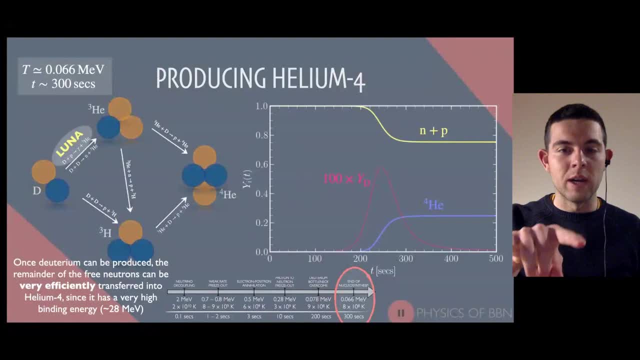 reactions in the lab, that that really does correspond to an energy range that you have to target. so yeah, i think it was very much kind of on purpose. maybe another dumb question while we're while we're on a tangent: it's not possible, or at least if it is possible, you can't do it as as well. 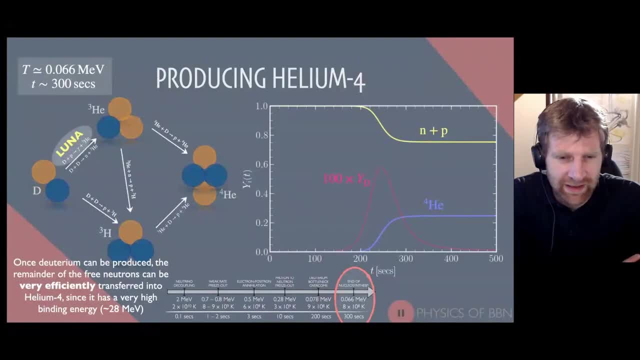 to just like predict this from first principles, from like a nuclear physics theory. this is not a dumb question. this is part of the disagreement, which is: what is the right way to go about using this data in particular, what's the right way to use this data in conjunction with the other two? 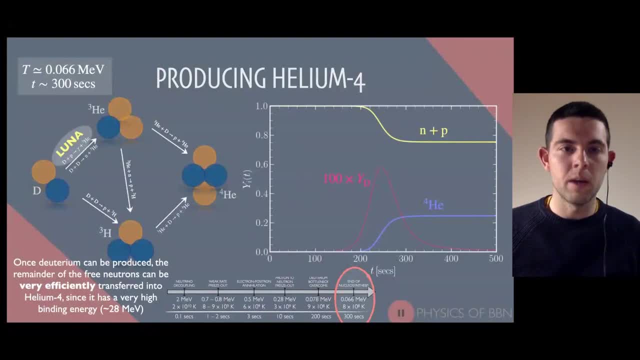 rates, because this is the right way to use this data in conjunction with the other two rates. there are two ways to go about it. the other way, one way is to use exactly what you suggested. you do some you know, some theory predictions based on, you know, whatever kind of perturbation theory. 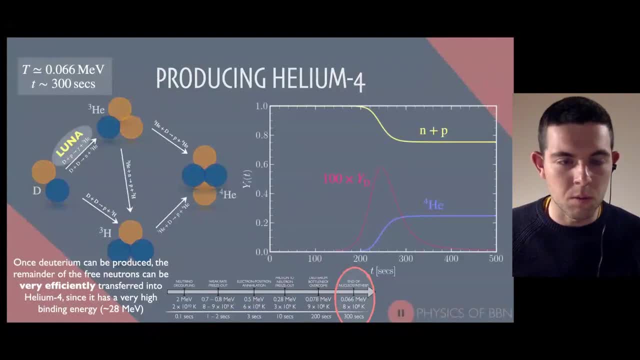 models you want to use, for example. or you can take a kind of data-driven approach, purely data-driven, and you only use data that's available and you basically take no theory, prior view on what the rate should be. you basically just make kind of data-driven fit. 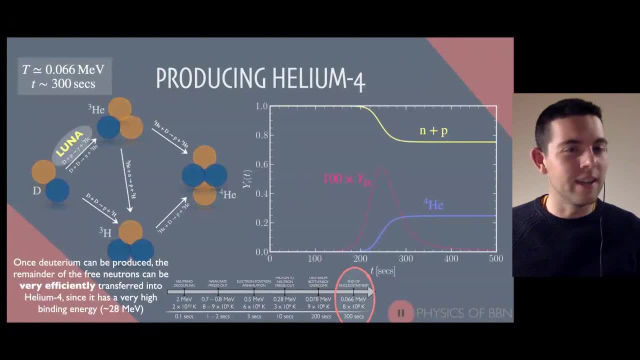 and it turns out that those actually give slightly different answers. so it's certainly not a daft question at all and i think actually it's right at the crux of the current debate, which has kind of evolved since the lunar measurements. a word that you might see in: 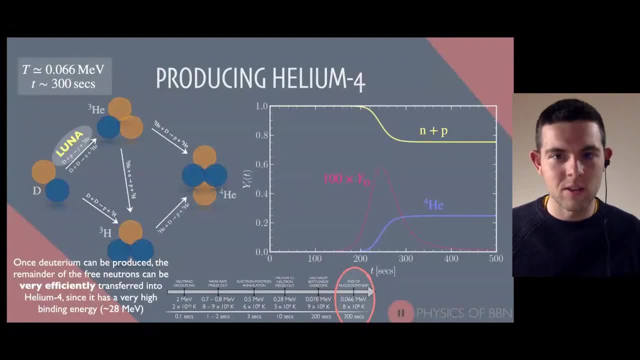 this regard is is like markucci rates. that's kind of the theory prediction for d plus gamma goes to three helium, just put some terminology on it. but yeah, i think you know that's a crucial part of it. i think i'll give a bit of outlook later on, but you know that's one of the key points. it's not you. 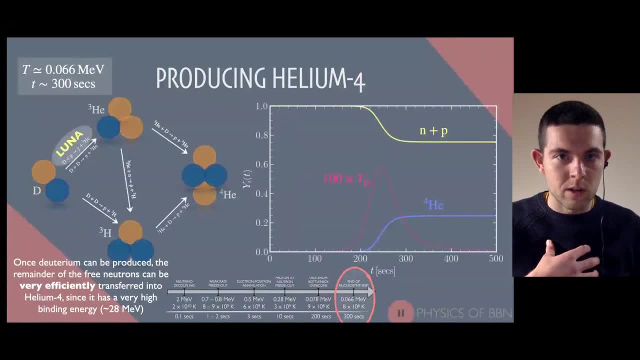 know it's not really my field is not making these measurements or doing the standard model predictions, but you know, consensus that kind of has emerged is that that's one of the things that needs to be pinned down, either with very, very good theory predictions or just improved measurements. 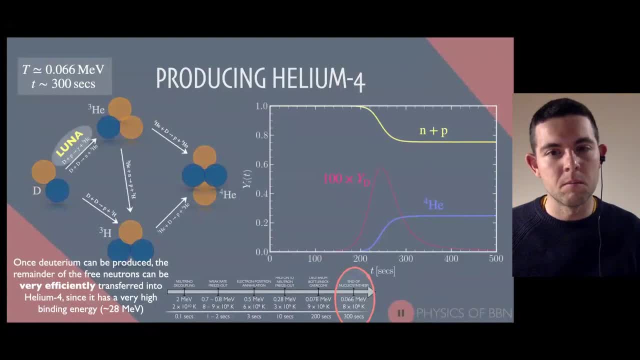 so that the theory predictions are almost become a little bit like just unnecessary, right? i mean, is the argument that they have, then, that the theorists say that lunar have got a systematic error and lunar tell the theorists that they're making approximations that are invalid, or or are they claiming there's some missing new physics that, yeah, no one really disagrees with? 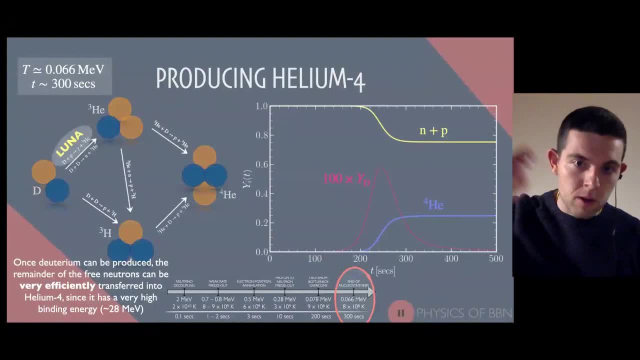 lunar. so lunar, lunar- i'll show the data in a sec. but lunar make a very, very tight measurement of the reaction rate. it's just, it doesn't really overlap with the theory prediction for that particular measurement. which means that if that theory prediction doesn't work- and it's a very 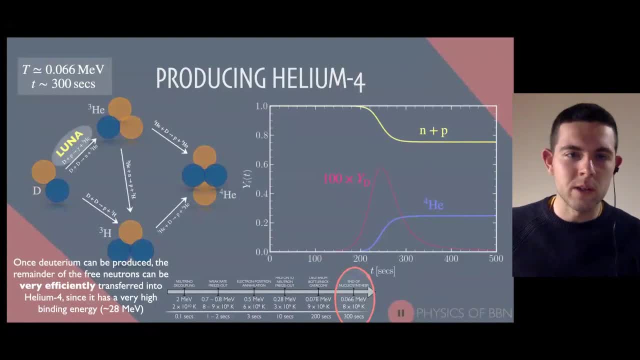 similar type of system. if you're using the theory prediction for that particular measurement, then you're not really making any predictions for that particular measurement. so the theory predictions, for example, for d plus d, goes to proton plus tritium as opposed to using the data. that 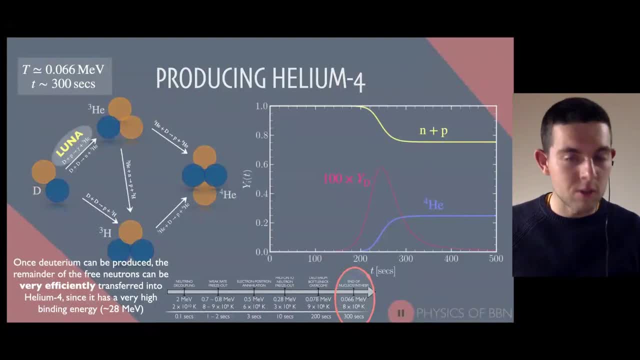 exists, only the data that exists, you know, are those two approaches compatible? are they consistent? you know, i think those are the questions that luna has has kind of brought up the optimal. i think all the the nuclear physicists will tell you the optimal way to go about this is to not. 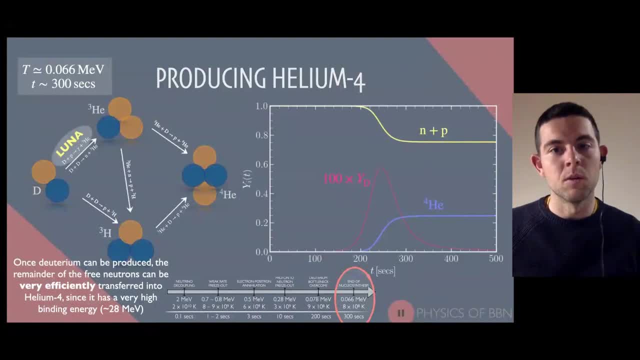 have to rely on theory predictions and just measure the rates. but that can be very difficult. so sometimes you have to, especially if you want to, so you may have some measurements in a certain energy range and you want to kind of extrapolate to another energy range. there are multiple options. 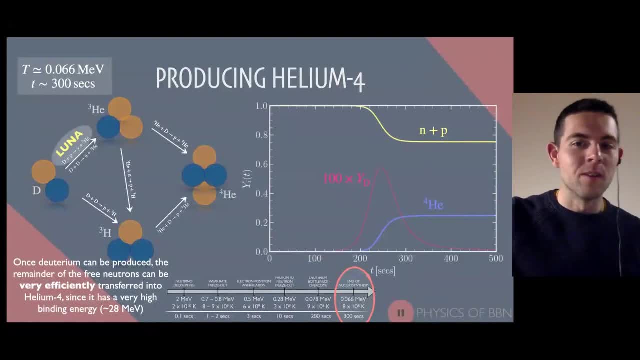 for how to do that. but yeah, okay, so we've produced helium-4, but as um you know, and one thing maybe just to note here- is that actually the total baryon number is is conserved in these interactions. just a nice thing. if you add up n plus p plus four helium, that covers basically all your baryons plus. 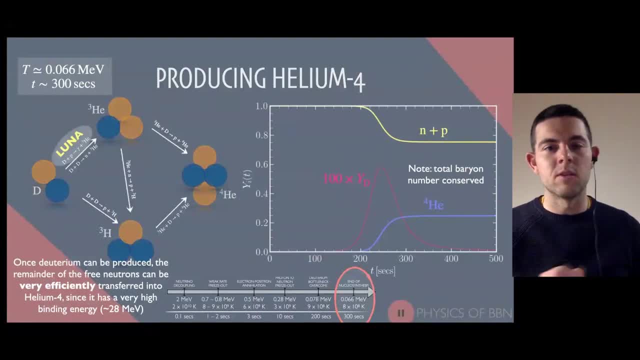 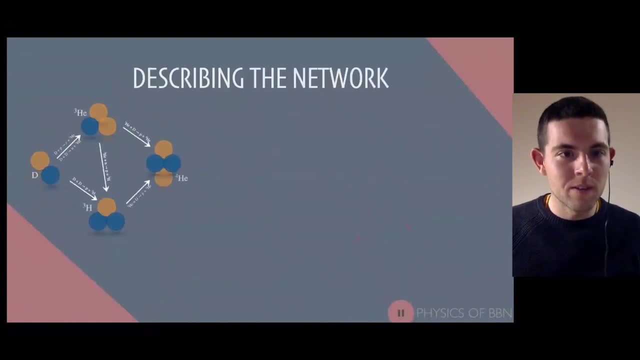 trace amounts of the other other elements. all that happens is that you have a lot of these trace amounts, and that's what happens is they just get transformed into different isotopes. okay, but, as we said, kind of what you really want to know is: what are these trace amounts in? 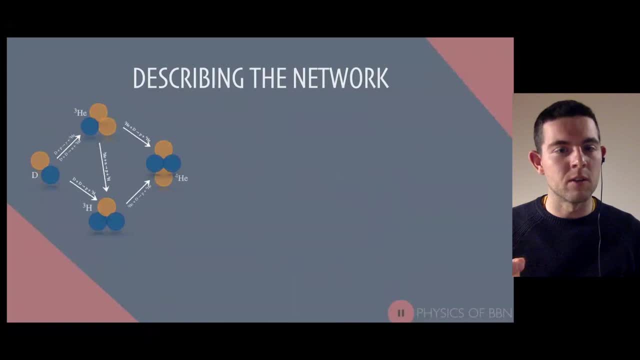 particular deuterium, because that's the thing that you have an excellent abundance measurement of and that requires some careful tracking. and one one question that arises when you try and do that is okay: how do i track each of the, the abundances? and what you need to do in a technical sense is: 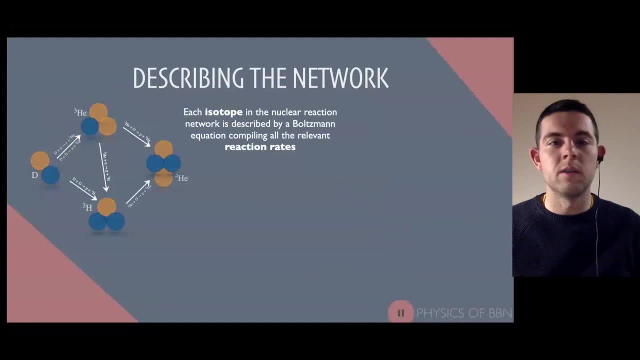 you need to take a boltzmann equation for each of these isotopes. so for deuterium, three hundred helium or, if you're interested in, like lithium, seven and you know any particular isotope, you have to do all of them. you have to solve these as like a kind of coupled system, because of course, 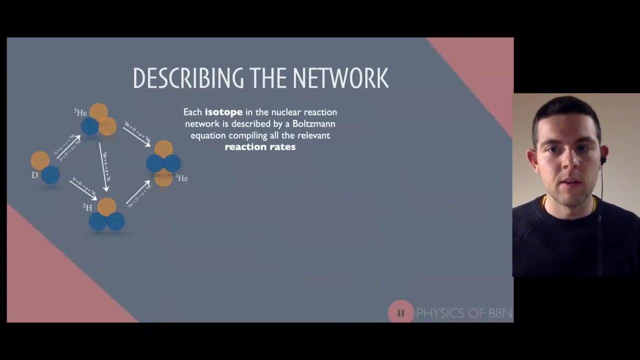 these reactions can transform one into the other and you write it down and then there's a couple of components here. so one of the things- there's a cosmology kind of dependence here, which is just your expansion history. if you just had no interactions on the right hand side and you 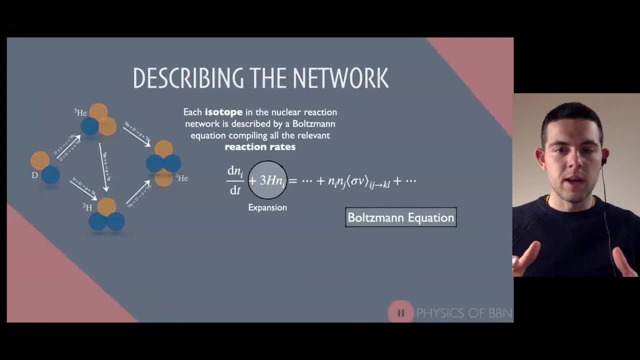 took a box of baryons or deuterium and you just let the box expand, the number, density decreases. you have a second component- and this is the kind of crucial part as far as luna is concerned- which is that you have reaction rates, that this is an out of equilibrium process and this is kind of 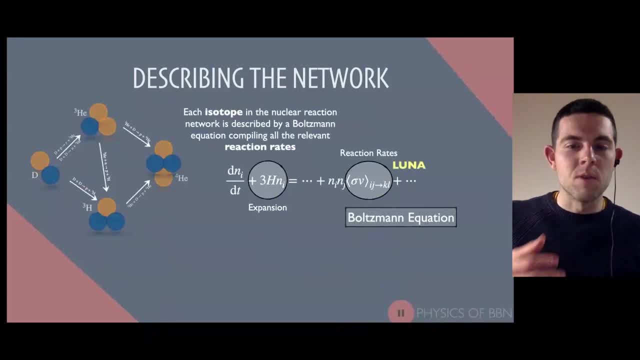 the statement i was making earlier, which is that, ultimately, the reason that bbn is a good probe is it's not just a box that has no interactions and it's expanding, you know, and it's not in thermal equilibrium. you are sensitive to these reaction rates. they're not in kind of thermal equilibrium. 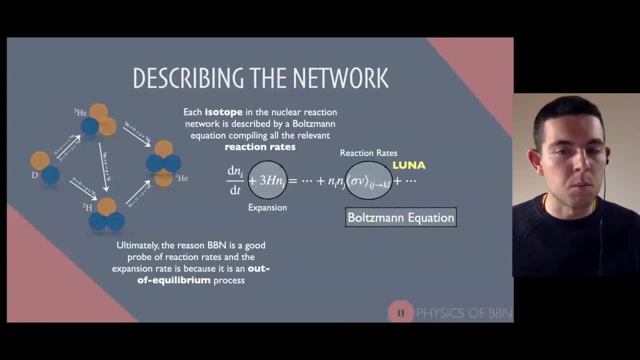 so you need to measure them or you need to predict them, and then you need to plug them into your system and solve it with some kind of high fidelity to resolve these kind of final abundances. so that's kind of how you want to actually describe the network and i say it's. 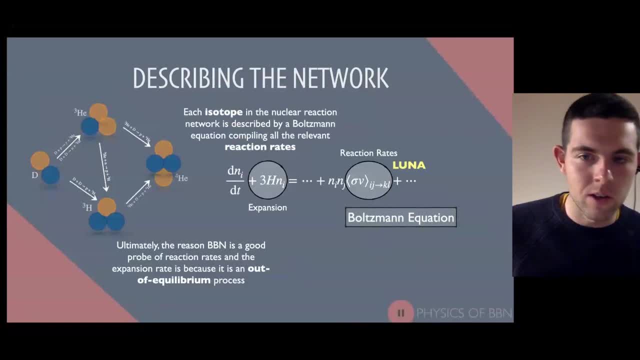 luna comes into really measuring this quantity on the right hand side, so you know the actual reaction rates. cool. so finally we can kind of get to deuterium and look at some data, because there's a lot of context that goes into measuring effectively what is kind of one number. 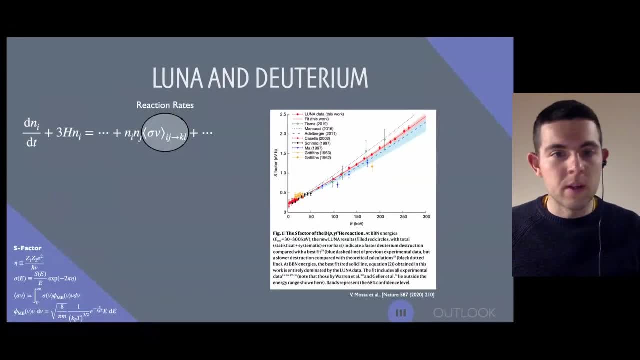 one function of energy. so luna experiment in 2020. they remeasured the reaction rate for this. d plus p goes to gamma plus three helium reaction. you know, one of the crucial arrows in in that reaction network, as you know, kind of maybe discussed earlier that that's not the only one, but it was. 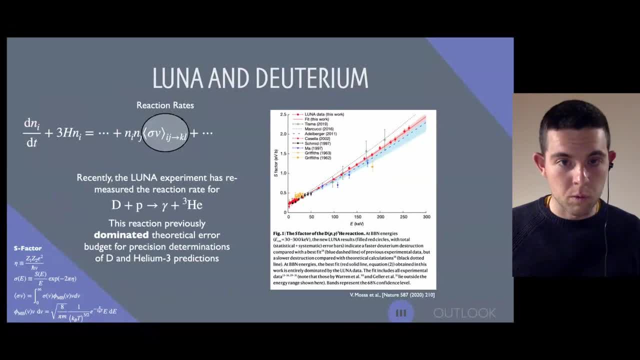 the one that dominated the theory uncertainty budget for, if you wanted to do, precision determinations of deuterium and helium-3. so this is this point about, like you know, the other ones, the better measured or just has less of an impact, because perhaps, for example, the rate is just 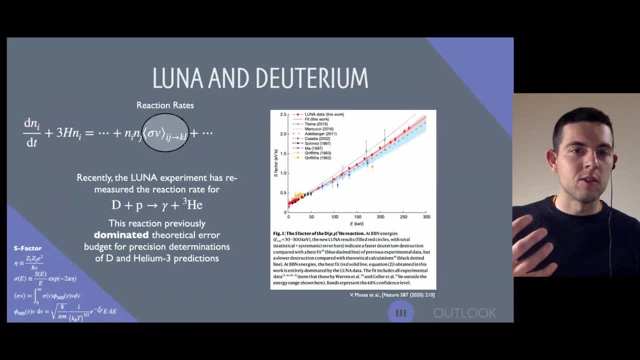 smaller. it's not just about the measurement, uncertainty, it's just about like, how much does the rate control the abundant? and i say previously this: this d plus dp, gamma to 3 helium completely dominated the error budget. so these lunar measurements, which are the red dots on the plot, 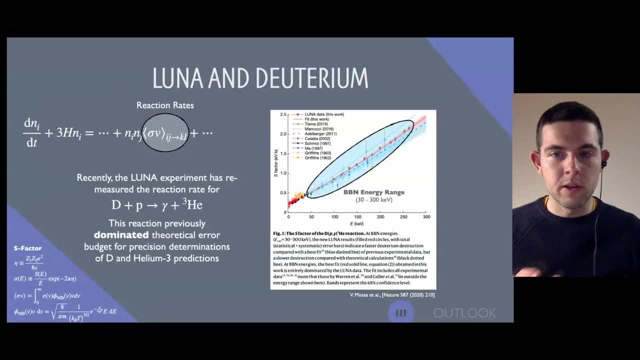 in this kind of bbn energy range of 30 to about 300 kev, you know, significantly reduced any, any uncertainty coming from this reaction. you can kind of see, compared to, for example, like the, the green crosses, which are from 2019 in the same energy range, you know, these error bars are significantly smaller. 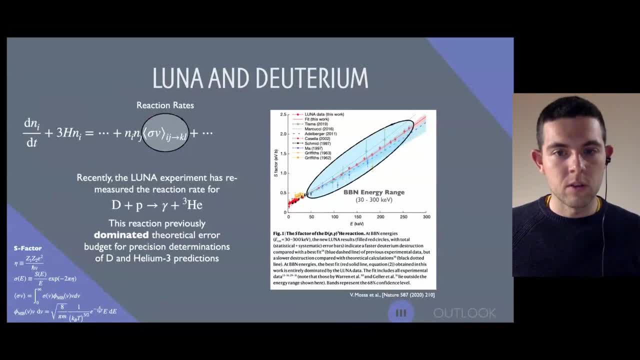 significantly more numerous and and very precise. so these lunar measurements are very important for for controlling these, these abundance predictions like. looking at this plot, the thing that jumps out to me by eye is that, at the lower energies, these yellow data points and these red data points are: 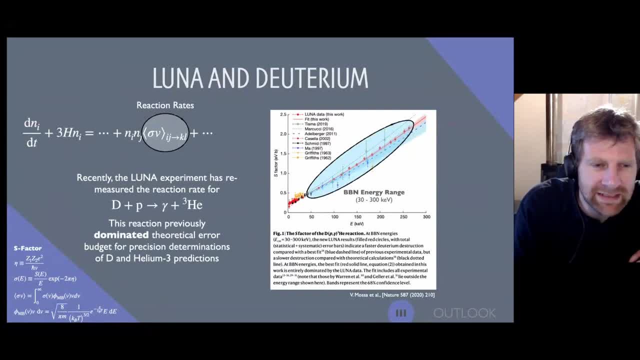 completely inconsistent with each other. but then i look at the date of the yellow ones: it's like 1963. are we just meant to assume that there's some systematic error there? i think so, yeah, okay, but i think there is something to. if you're, you know, talking about inconsistencies, i think that there. 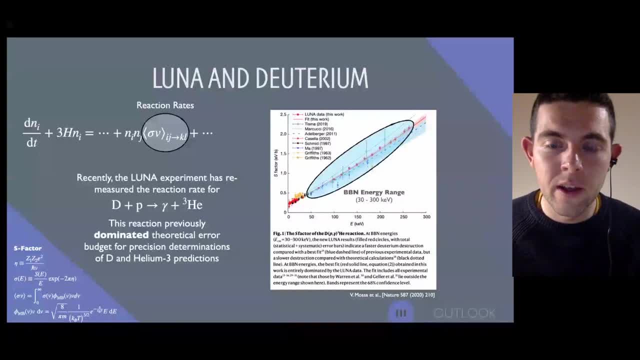 is something to note here and it's the black dotted line. if you can see it and if you want to compare that to the red dots in, in particular in the bbn, at the top end of the bbn energy range, that's this markucci line. this is the theory prediction. those two are not necessarily. 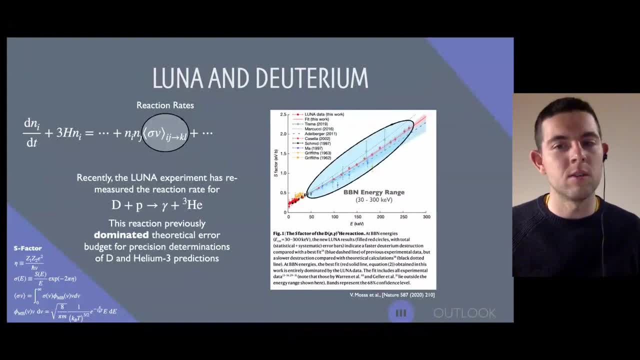 consistent. i don't think, you know, no one really has a problem with that. like the theory, predictions are very challenging and, as i say, the best thing you can do is go and measure it really really well. but it is, you know, telling someone in this reaction that those two things don't overlap. 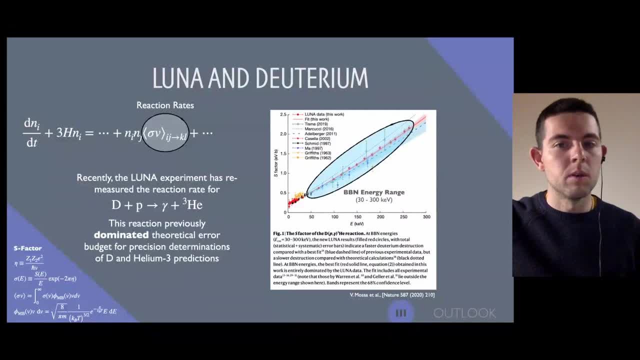 and i think that's something to to keep an eye on for for the future. right, so you know, this is the lunar data and you know, one question that you might ask is: what are the implications of luna, especially in the context of standard model bbn? so one thing that happened earlier this year was me. 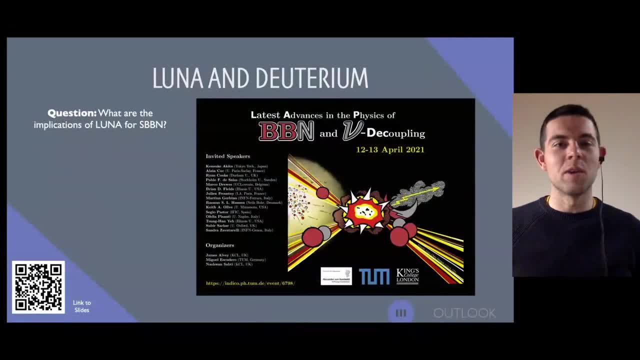 and nash. we ran a workshop on this, so it was great. we got to sit back and we hadn't done any of the work, um, but we got to listen. i think, you know, this was a huge reason for us being able to write the addendum, because we managed to get basically all of the protagonists from 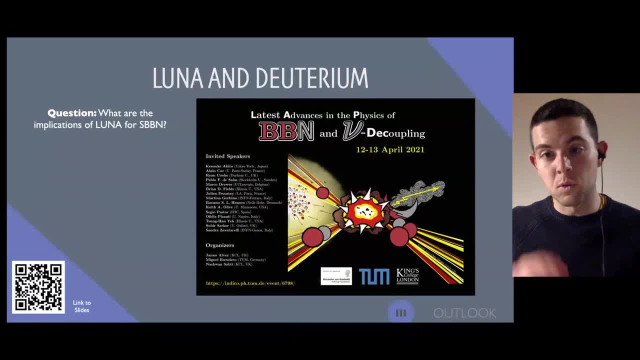 luna and the three groups analyzing the data. there was also an additional component, unlike the physics and neutrino decoupling, which was super interesting but not necessarily related to this kind of rates discussion. um, you know, we managed to bring everyone together and we got to. 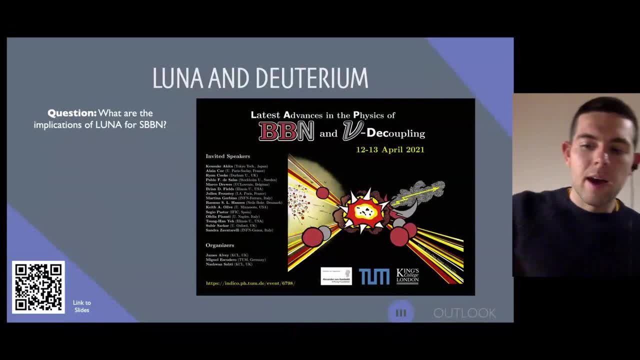 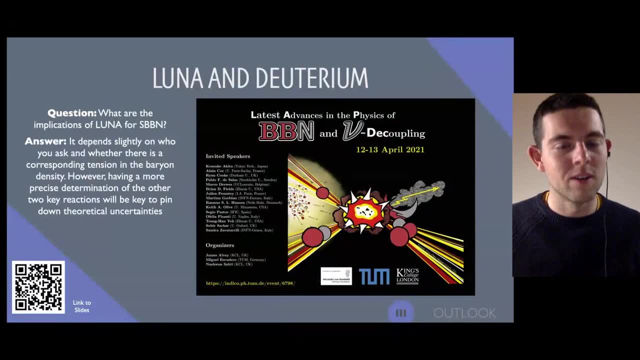 work together and it was hearing these kind of different approaches, and you know the answer to the question of what are the implications, are it? it does depend slightly on who you ask and, for example, whether that person will tell you where there's a, whether there's a corresponding tension. 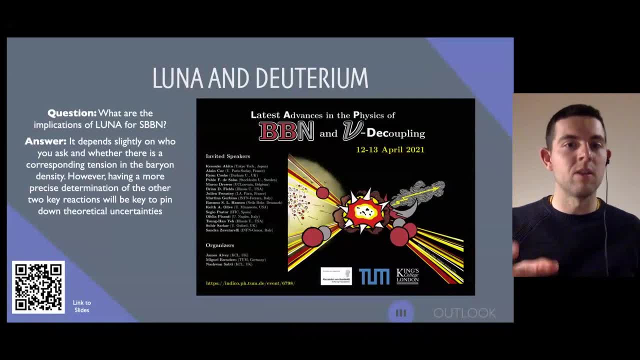 in the baryon density, because these rates, deuterium is an excellent what they, you know, i call bariometer. it is the thing that really tells you it's very sensitive to the baryon density. so deuterium and measure predictions and measurements of it. 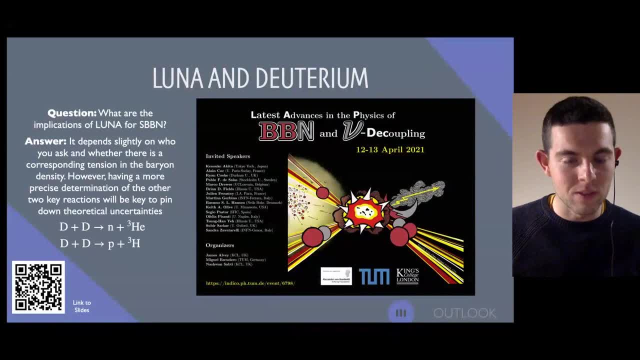 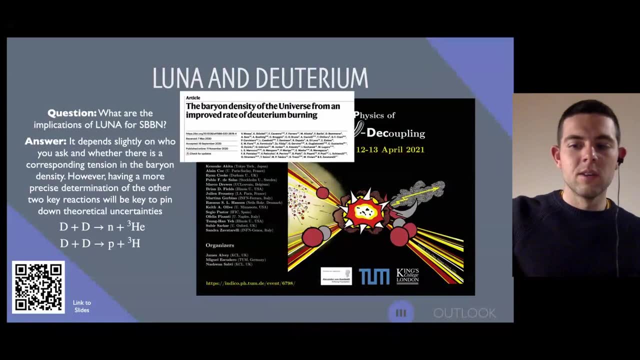 the key tool in using bbn to measure the baryon abundance. so you know, of course these rates have a have an impact on that discussion and i say you can flick through kind of some of the papers that appeared. so this is the luna paper. they did an analysis. there's an analysis from a group in 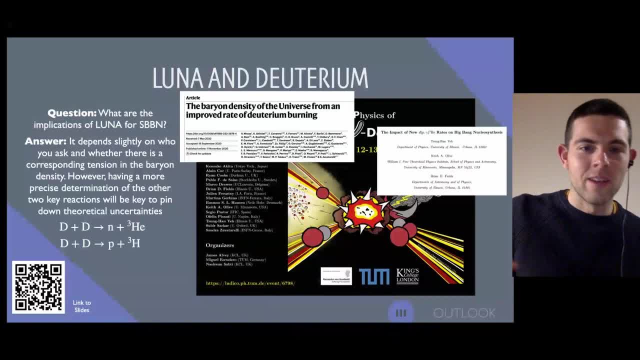 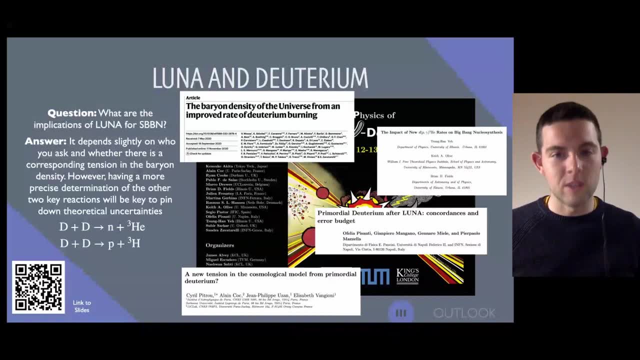 the us, there's an analysis from a group in naples and there's an analysis from the group in france, and you see that they kind of have- um you know, different conclusions. so, for example, the french group say: hey, there's a new tension in the cosmological model. perhaps there's this. 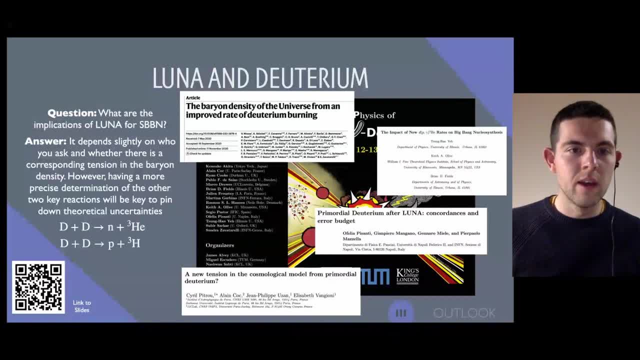 a sigma, two sigma difference between the baryon density and i think something that came out of this workshop that was, you know, super interesting was the fact that this was not due to the code, so they used different codes. but it was not due to the codes, but it was probably due to the way that 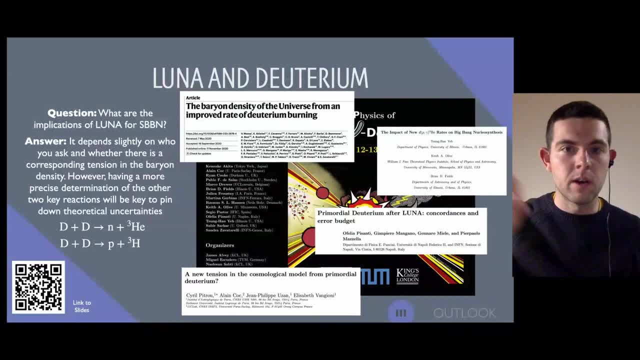 they dealt with, not the luna rate. so the luna rate, you know is, is very well, very kind of well determined. it's actually really how you deal with the other deuterium rates and they, you know whether you deal with them in. you know the same way: either you take the theory, predictions, or a 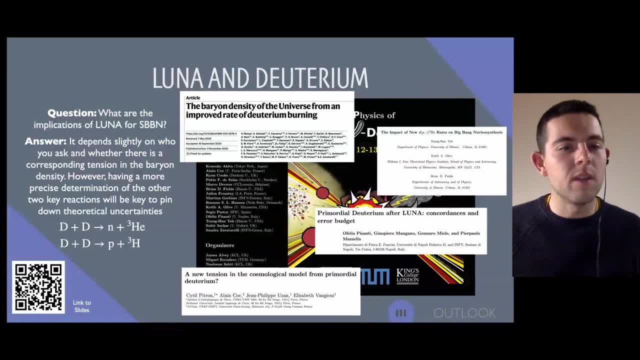 driven approach that can change your conclusions and kind of the. you know the outlook from that and i really recommend going to have it. so i've put like a you know a little link there that you can, you can scan, you go and have a look at some of the slides because you know it's easy to learn a lot. 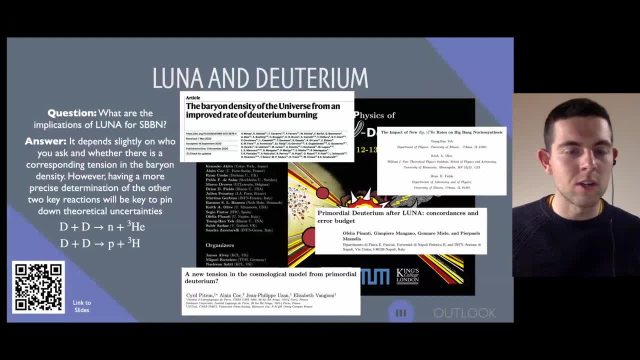 very quickly and you pick up the kind of subtleties of this discussion and i say there's a couple of papers that came out after this workshop kind of with some recommendations, and one of the key recommendations is exactly this: that these other two reactions, which were not, you know, the luna, 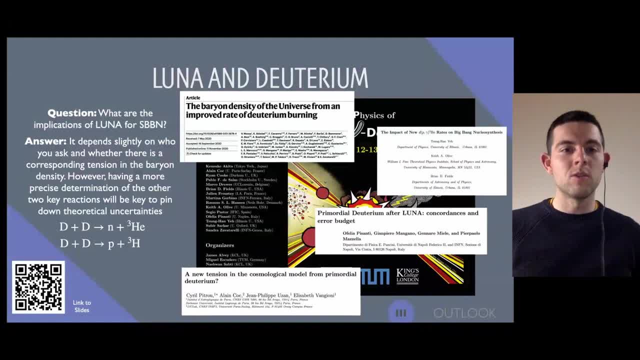 reaction that started all of a sudden. you know, the luna reaction that started all of a sudden debate is not listed there, but those two reactions we could really do with either pinning down, like the theory, uncertainties in them, or just having an excellent measurement at the level of kind of 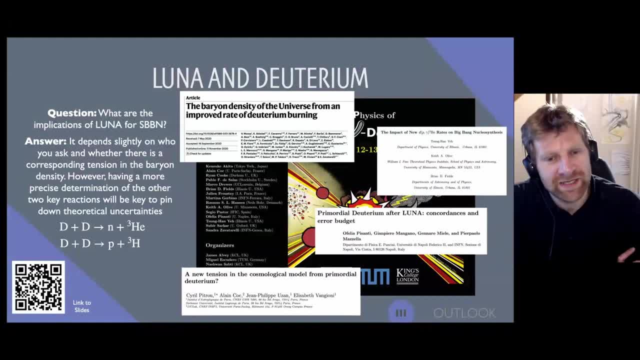 luna, right, yeah, so two years ago these ones were the well-measured ones, and now luna has has obviously improved a particular one, and so these ones are now the leading uncertainties, exactly, exactly. so now it becomes relevant to kind of take a look at this: how realistic and 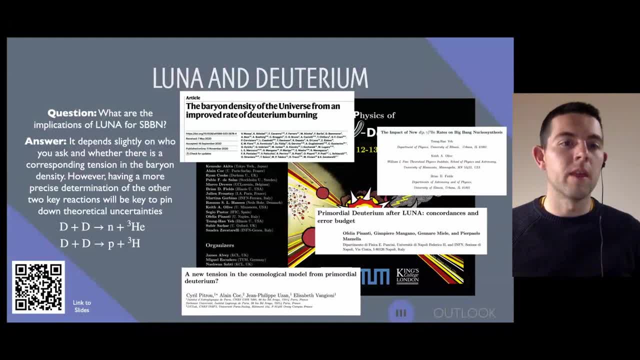 what sort of timeline that happens on is is not so clear. but you know, i think this is a sort of context that i find super interesting, because now you know that's something to look for. uh, you know, you go on the archive and you see, our new measurement of d plus d goes to p plus tritium. 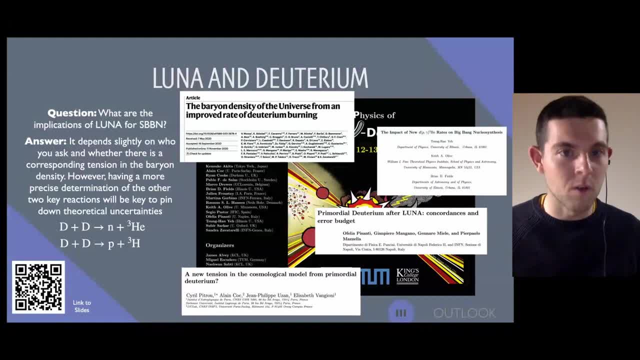 i think you know, in 2019 would i have opened that paper? perhaps not, but now i'm definitely opening that paper and that's the sort of context i think has appeared in the last couple of years about, like you know, why these rates are important and how to use them, and do we know of groups who? 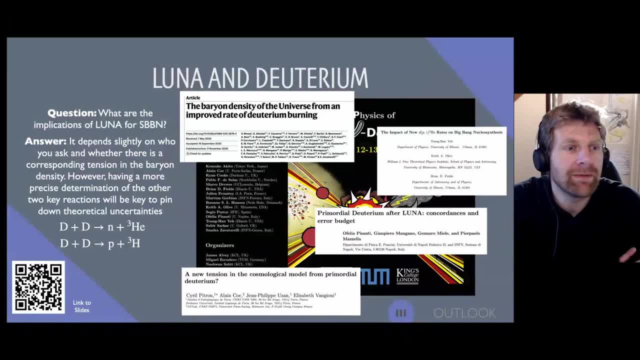 are like now out there, i mean maybe even the lunar people, i don't know who are out there intending to measure this exact thing, because obviously you've made a good case that it's important. i think, um, i think luna are looking at whether they can, you know, i think they will do. 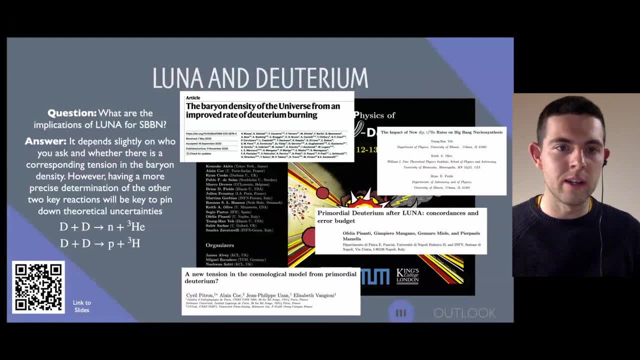 if they have the capability. i i think it's not 100 clear yet who will be the people to to do that. this is kind of what raises the question. i guess you know why did we write the addendum. we've come out. you know it's been a long way to. why did we write the addendum, but it comes. 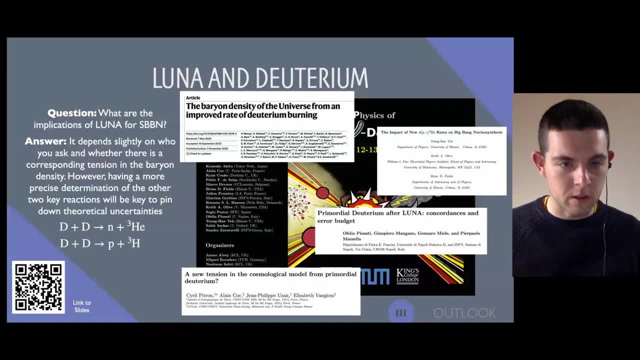 to the question of how do you proceed and keep using bbn as a a precision probe, especially if you want to use it at this level, if you want to use lunar data, for example, in making your predictions, because you know they tighten your theory uncertainties, how do you deal with this? and you know i'm going to suggest in a, in a bit like the: 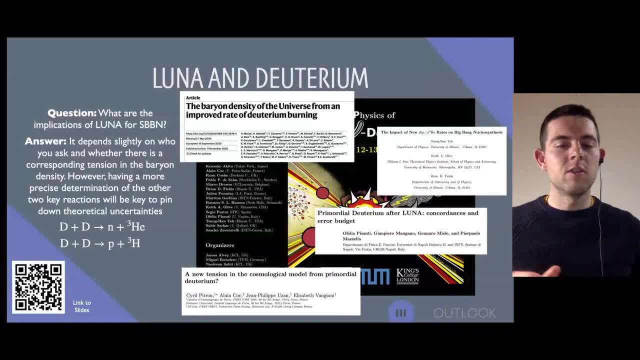 kind of the approach that we took was, in some sense you should consider all of these possible approaches, because i i certainly you will not catch me saying that one is right or wrong. i don't think that's really the the correct way to see this. i think the way to see it is kind. 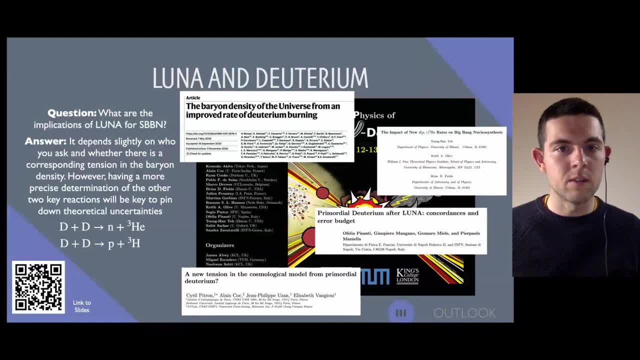 of along the lines of that. they're different, you know, they give slightly different answers and actually from a kind of practitioner point of view of using bbn as a as a tool to understand my, you know, perhaps beyond the standard model physics, i should kind of almost kind of marginalize over that. you know that is an ongoing discussion and i 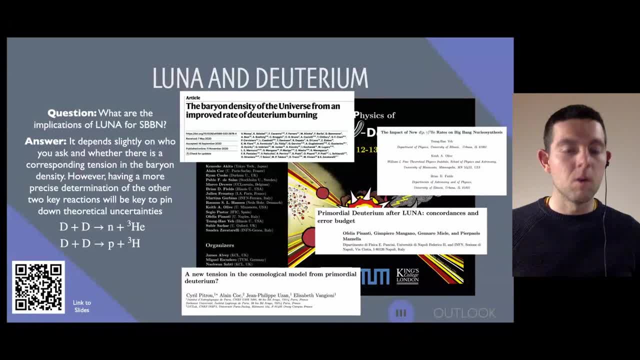 i want my results to be insensitive, to kind of, or at least i want to present the reader- or you know whoever's using my numbers. i want to present them with the option of whatever numbers come out of that debate, you know. so that was really the motivation for writing, you know. 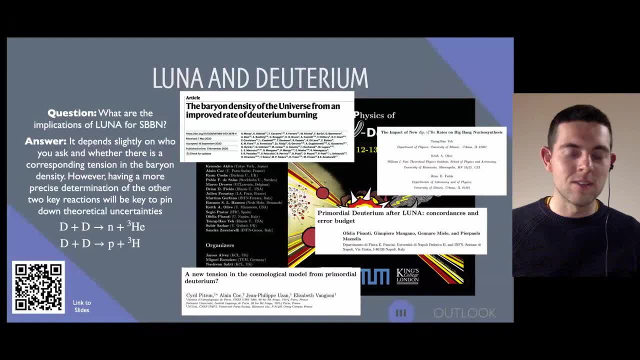 this whole long story about how do you get down to these three reactions, that that was really the motivation for writing, you know, writing the paper in the end, and it was a useful excuse to to learn all about all about this physics. but yeah, so maybe just kind of a final thing of like, okay. 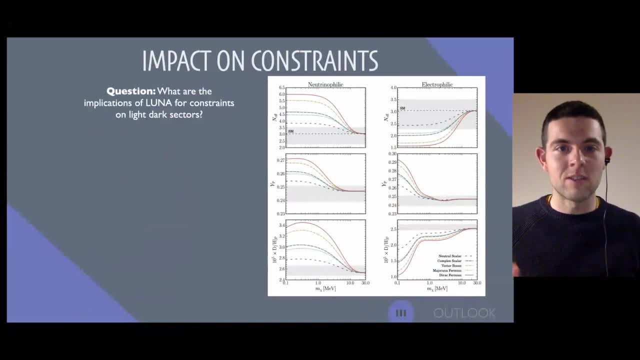 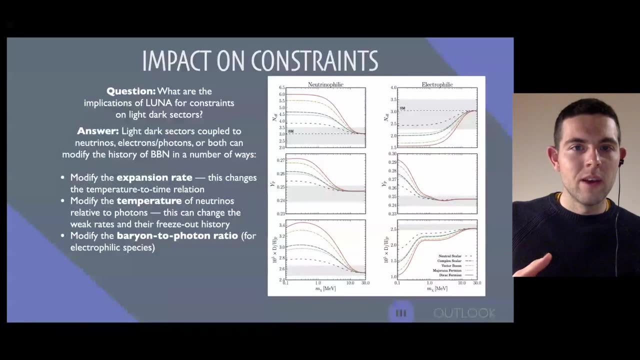 what are? what are the implications for constraints on on our like dot sectors? fortunately, with you know the the discussion we've had so far, it's not so difficult to to explain what happens. and so if you have a light dot setter- and you have, maybe it's couple. 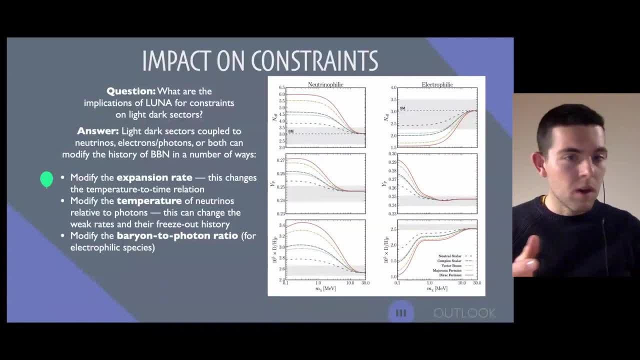 to neutrinos or electrons and photons. maybe it decays into them or it might be coupled to both. then it can kind of modify the history that we've talked about so far in a couple of ways. so the first thing it can do is it can modify, like, the expansion rate. if you have a particle at the mev. 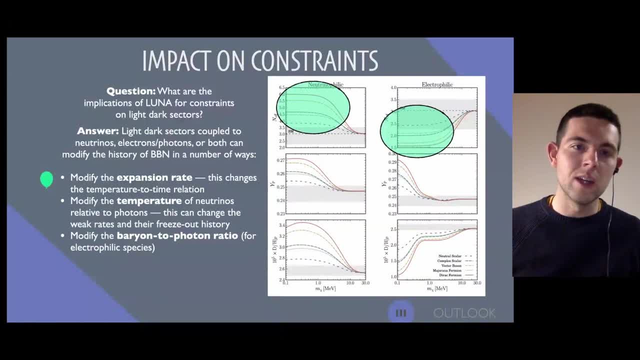 scale. you know that that is a dominant component of the energy density at the. you know the temperatures relevant to bbn, so that can affect exactly this kind of temperature time relation and you know you can see this, for example in the parameter like n effect. it's something that counts. 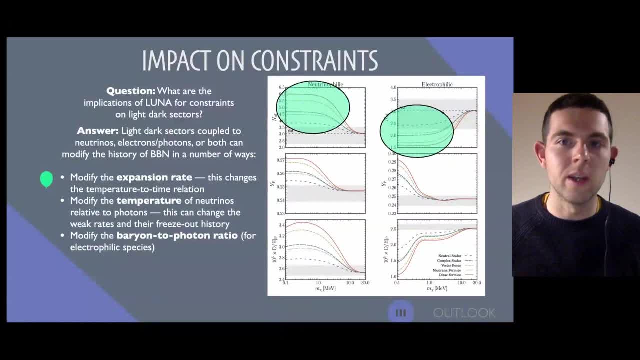 kind of the, the relative number of times the energy density of the energy density of the energy density, relativistic degrees of freedom at this time. So you can either boost it in the neutrinophilic case or decrease it in the electrophilic case And that will change your temperature to time relation. And indeed that kind of is the. 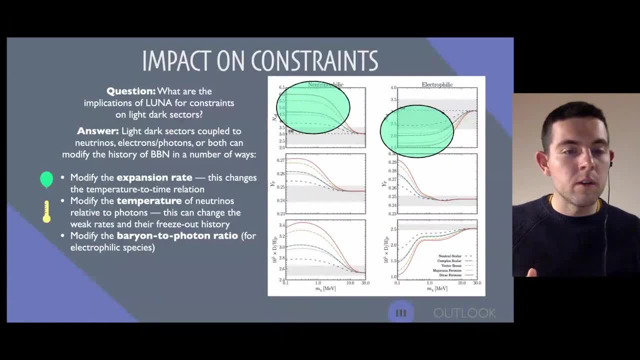 dominant force for things like the helium predictions. It can also do something else which is a little bit more non-trivial, So it can modify, for example, the temperature of neutrinos relative to the photons. And again we kind of mentioned this briefly- is that the weak rates which 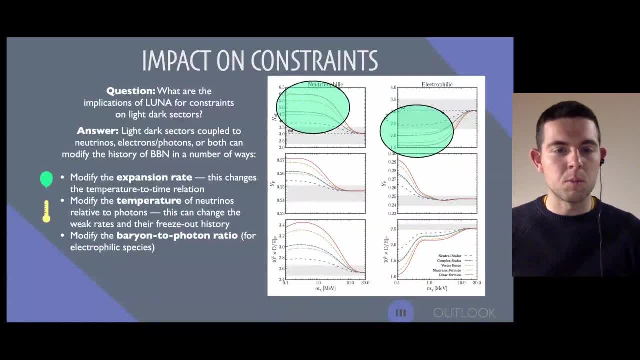 cause all of these different timescales and the interactions between them. the weak rates can actually change if you change the temperature of neutrinos. So you do really need to kind of solve for the full weak rate history to understand this effect, And I think that's a little bit more complicated to have some deep intuition for, but you should include it. 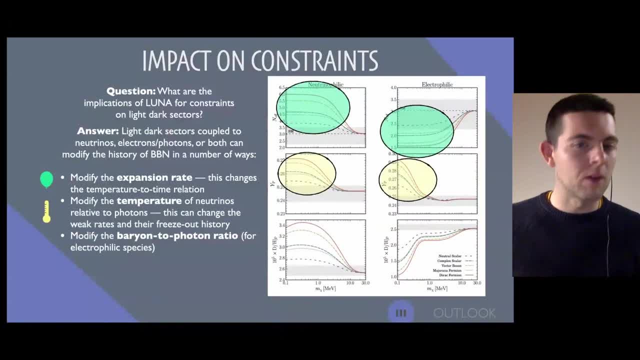 And the final thing that you can do is you can modify, like the baryant to photon ratio If you decay, for example, into photons, in exactly the same way that electron positron annihilation heats photons up if you have some light. dioxide. you can modify the baryant to photon ratio If you decay, for example, into photons, in exactly the same way that electron positron annihilation heats photons up. if you have some light dioxide, you can modify the baryant to photon ratio If you have some light dioxide. 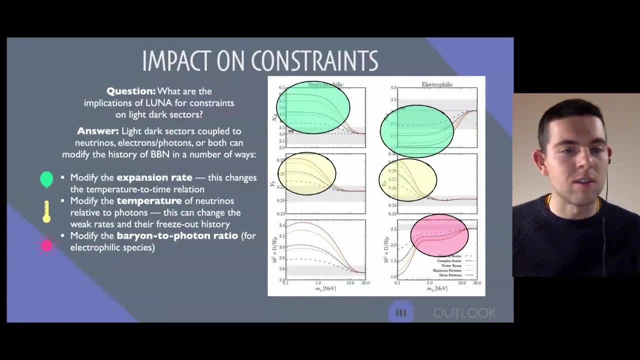 you can modify the baryant to photon ratio. If you have some light dioxide sector that decays into them at like, a later time, that can change the temperature and, in particular, you can modify the baryant to photon ratio And that can lead to effects like the following, which is where actually you can decrease, for example, 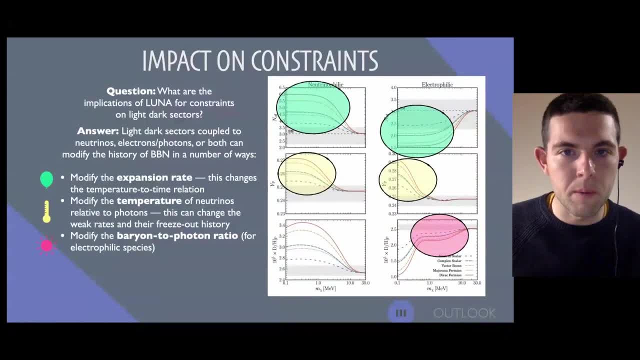 the deuterium abundance. So now you have to think about constraints. and where do the constraints come from? And to answer this question about, about Luna, And it's in the regions where they are dominated by Yp or the helium. you know your constraints and this is typically 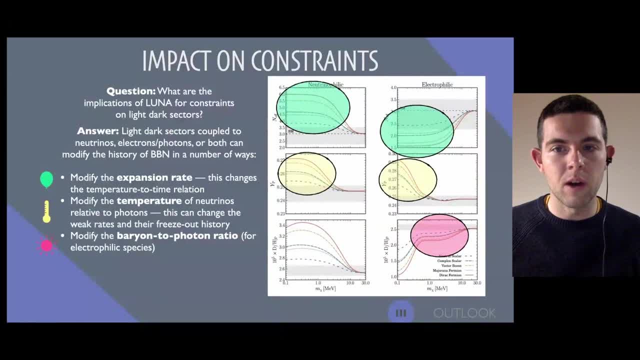 at the kind of slightly lower mass end, or you can see where the kind of yellow highlighted bubbles are. That really has very little to do with Luna, And we, you know, when we did the reanalysis, we did find that There is kind of a couple of cases, though, in particular for these kind of electrophilic particles, where 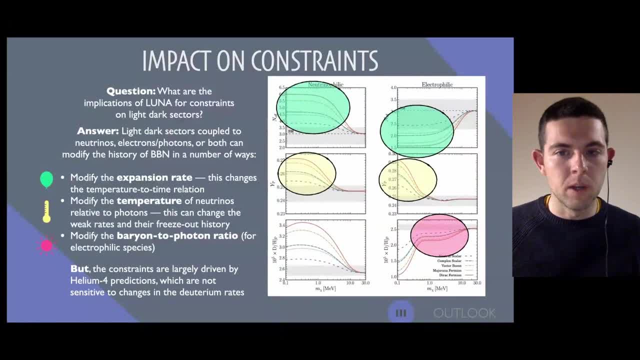 the deuterium predictions can shift up and down a little bit And you know we found that for a bound of kind of four to seven MeV that can shift by a couple of MeV. Now this is my point. It's, you know, if you're driven by helium-4 prediction. 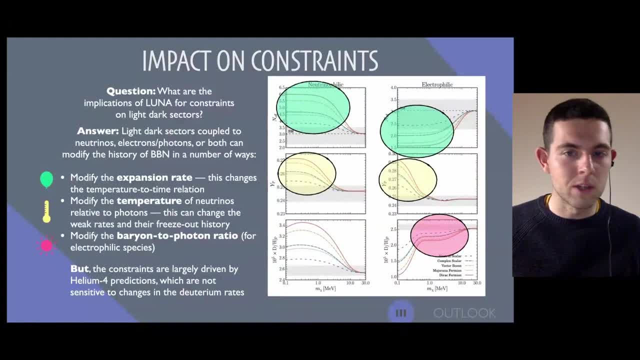 Luna, really doesn't have too much consequence for you because the helium-4 prediction doesn't really change. If you do have a BSM scenario where deuterium is kind of your dominant constraining factor, then actually you know, taking into account these different approaches for the three reactions relevant to deuterium, predictions could be quite important. 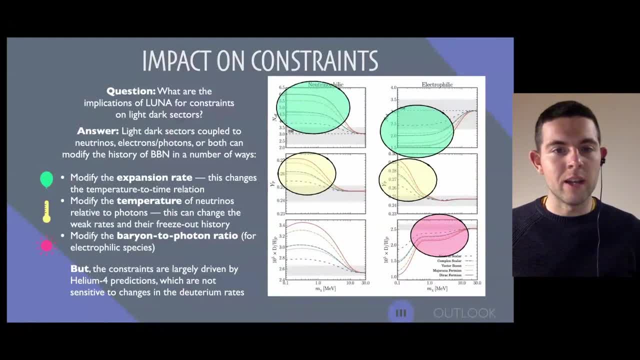 And I say the approach that we took was to basically consider all possible sets of rates and see how the constraints vary, And and I think the reason for that is, ultimately it's an ongoing discussion, as I said kind of just before, and it's not our place to take a position on that discussion yet. 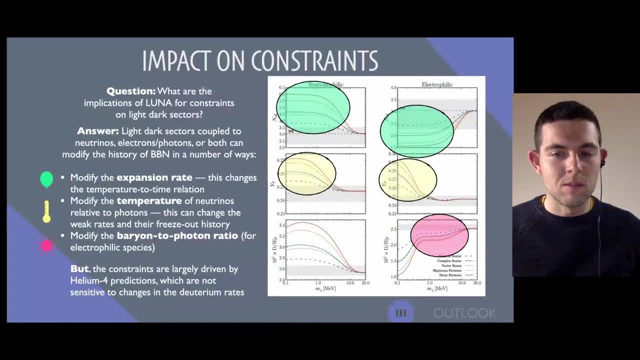 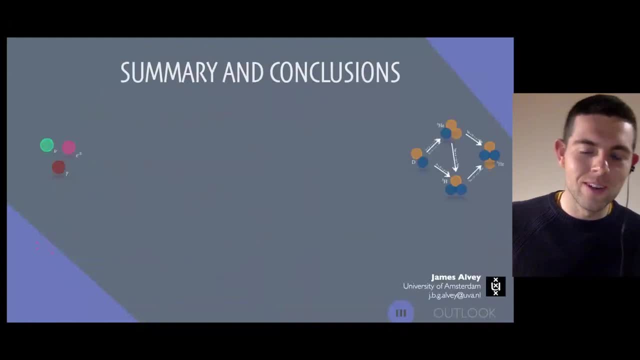 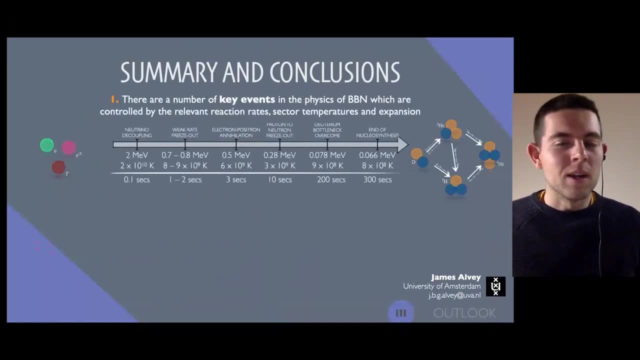 so what we can do is we can, you know, still marginalize over over that kind of effective kind of discussion- uncertainty if you want to call it, but yeah, that's kind of all I have to say in that regard. so just kind of flash up some kind of summary and conclusions. the first one is: 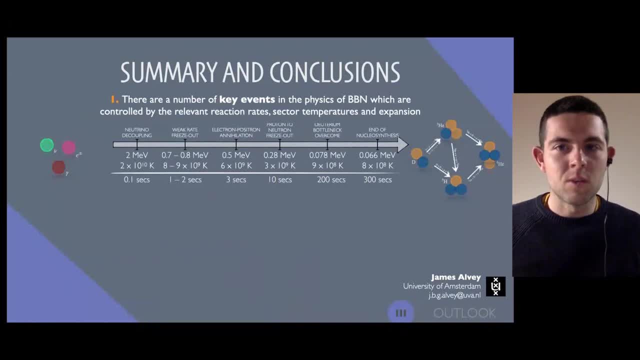 that there are a number of key events and the physics of dbn is is relatively complicated, but they can kind of be delineated and the cosmology can be sold separately to the nuclear- the nuclear reaction network as we discussed- and you end up with this kind of. 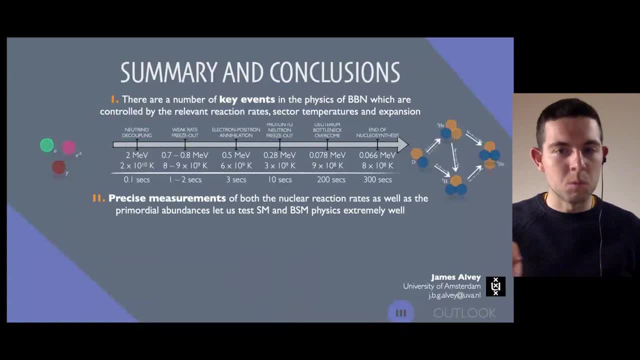 nice, clear picture of what physics impacts what temperature and at what time. and given this context, so given this kind of good understanding of of the physics, then we have precise measurements of the physics and then we have precise measurements of the physics and then measurements both of, like many of these nuclear reaction rates, but also, most importantly I think, 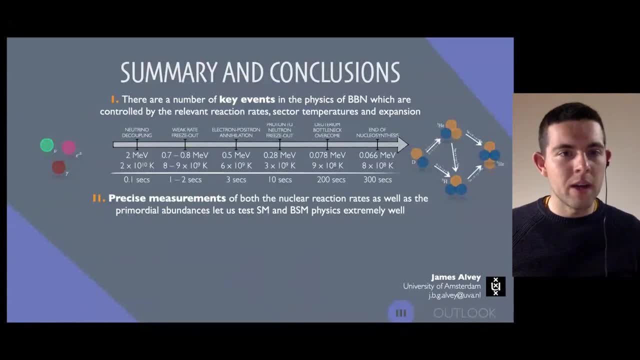 like the primordial abundances and combined with a good theory prediction, those, let us test standard model and bsm physics really very well. you know, in number of regimes these are like perhaps the most relevant constraints. and then, finally, you know, these new results from luna. they do require. 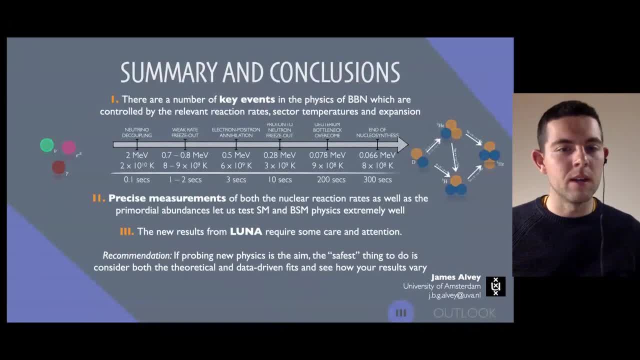 some care and I think the the discussion- hopefully I've made it a little bit clear- is is quite subtle. that means that you know if I was going to provide a recommendation on it, especially from the point of view of someone who's interested in kind of probing new physics. really you know if the aim is the kind of the safest thing. 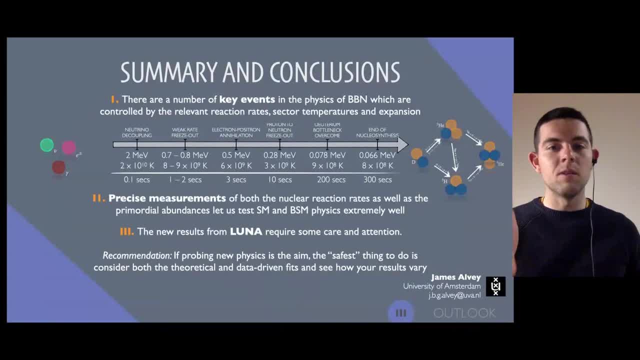 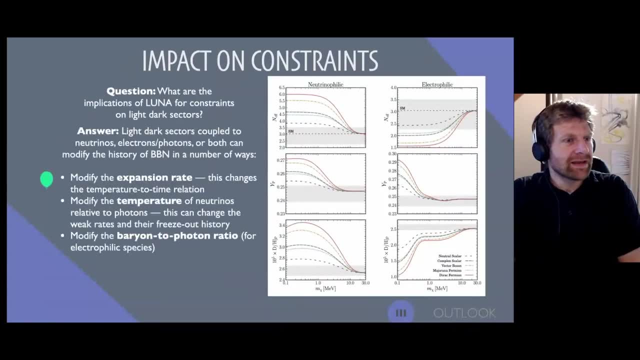 that you can do is to really consider all of these things- you know, the theory driven approach, the data driven approach- and then look at how your results vary. cool thanks. I was just wondering another thing. that's kind of complete tangent, but in all of your on the previous slide, all of your. 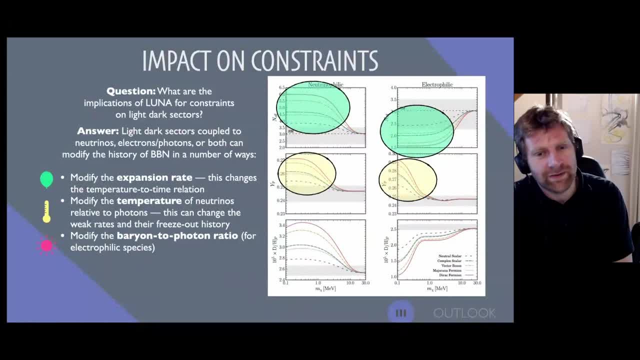 beyond the standard model. stuff increased the helium abundance. is there any way where one might have a model that decreases the helium abundance in the context of the physics that we were? so? I mean, actually, if you look, there is an intermediate region. it's quite hard to see on this. 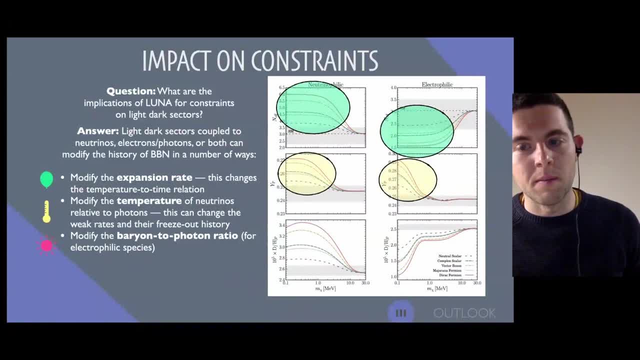 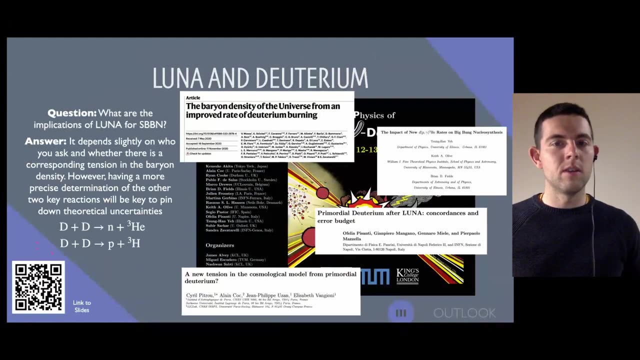 plot on the right hand side, about two to three mv, there is a tiny dip. yeah, it's quite hard to do because you have to effectively decrease the energy density of the universe at the times relevant to the bbn. typically, if you add new light species, they increase the- and you know the- expansion rate. 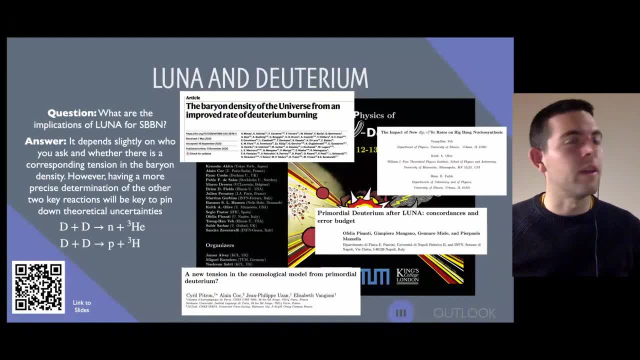 and that's usually the case. and then you have to look at the energy density of the universe and that's usually the dominant effect. you know, the outlook from a kind of community perspective is towards resolving and, I think, also understanding this issue and I think one of the 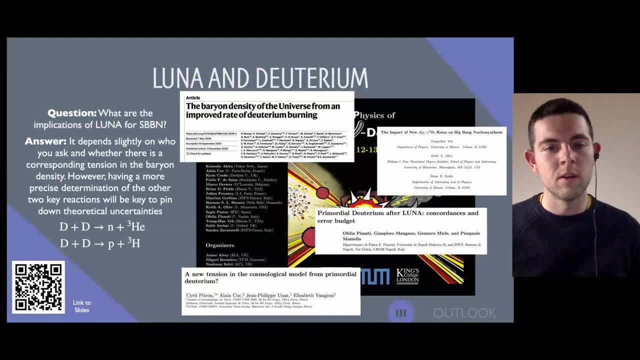 most interesting things that came out of that workshop that we had was you know that often these details can be stuck in papers, that if you're not a practitioner can be quite difficult to to follow the discussion. but actually, you know, the discussion is very relevant and it comes very deeply into that and I think that's a really important point and I think that's 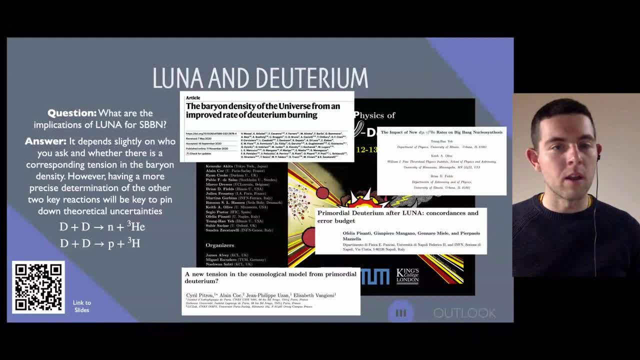 how you make predictions and how you use bbn as a probe. you know, I think a nice thing to do, especially as a bsm community, is to kind of get involved with these discussions, try and understand them, and then you can write better papers because of that, or at least ones that hold a little bit. 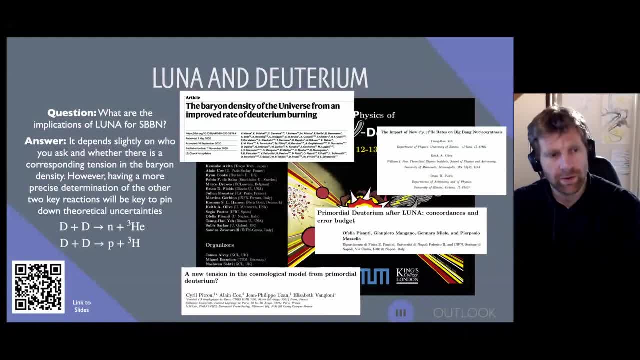 more to the test of time. it might also help the people who are having those discussions to know what is relevant to a community that is using their, their output. indeed, you know, using bbn as a standard model, physics probe is, you know, I think it's still relevant today, but it's still relevant. 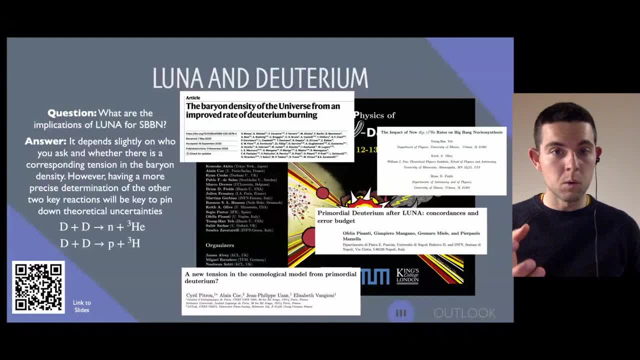 it's becoming less relevant, given the kind of relative concordance between a number of probes. so, you know, using bbn as a a real, you know, given it agrees so well with the standard model, typically as a, as a constraint on new physics in the early universe, I think it's an extremely relevant probe. 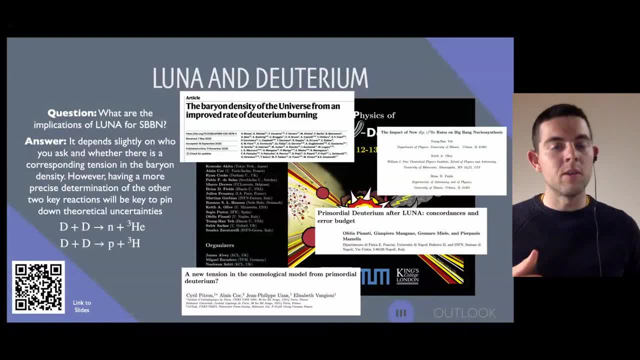 and therefore like understanding all of the physics. you know, I think typically it acts not so much as a place to look for new physics but it acts as a way to kind of rationalize your models. at this time, you know there are things that you can't do specifically, but you can do things that. 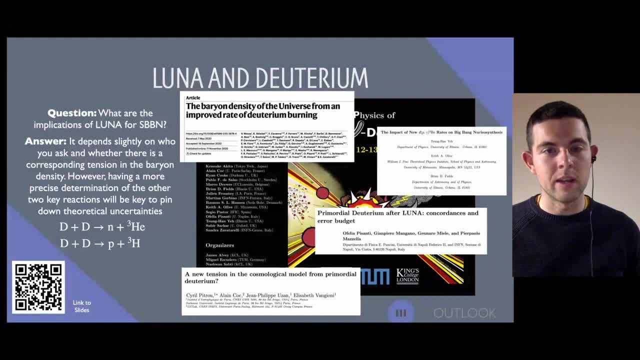 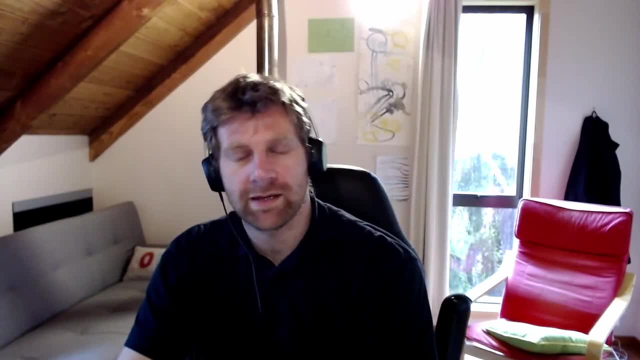 information comes from bbn. I think it's still a very relevant process today, particularly in the context of kind of the uses of precision probe. so okay, final question of what work being done in cosmology at the moment do you think is particularly underappreciated by the 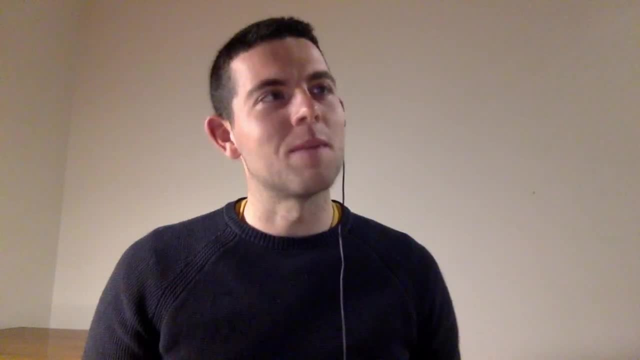 community as a whole cool. so I had a good think about this question because I saw you'd asked it in like a number of it. I think it's a really tricky question and I'm actually gonna. the work I'm gonna pick is based on, actually, the discussion we just had, so about neutrinos and what we know. 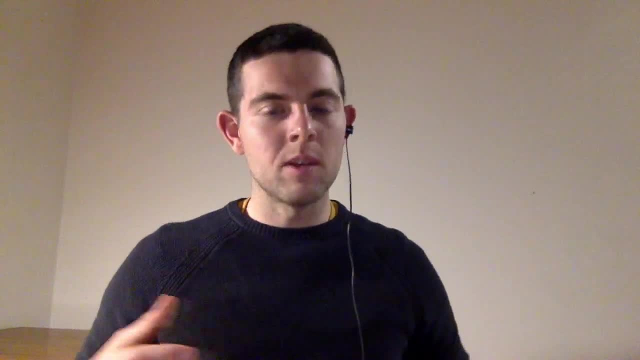 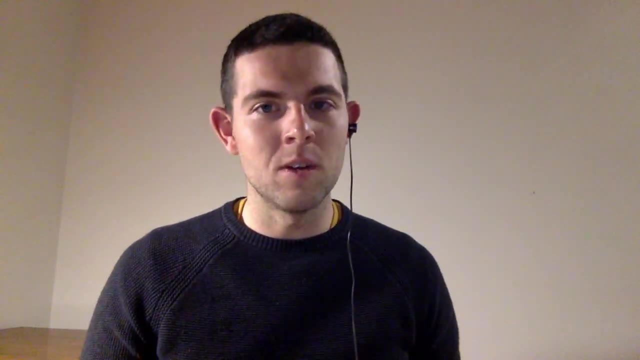 about neutrinos from cosmology and in particular, you know this- this prediction of kind of a cosmic neutrino background. so I think detection of the cosmic neutrino background is something I'm personally extremely interested in and I think it's a really good question and I think it's a 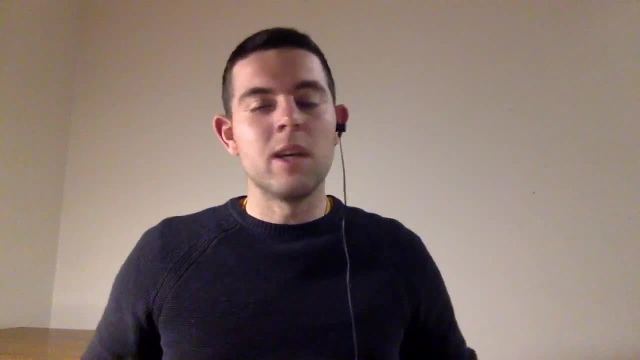 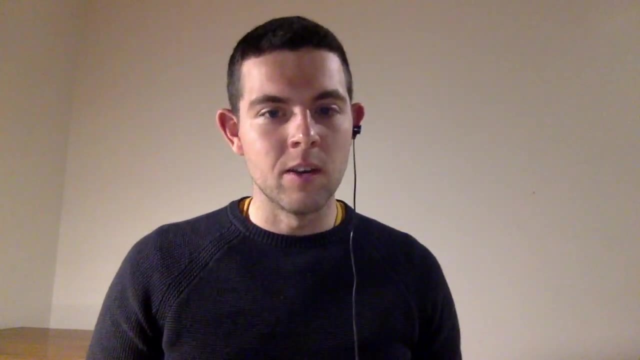 really good question and I think it's a really good question. but actually when you look at the literature is relatively kind of under it. there's a couple of like suggestions of how one might directly detected things like Ptolemy or project eight. you know, it's clearly an incredibly 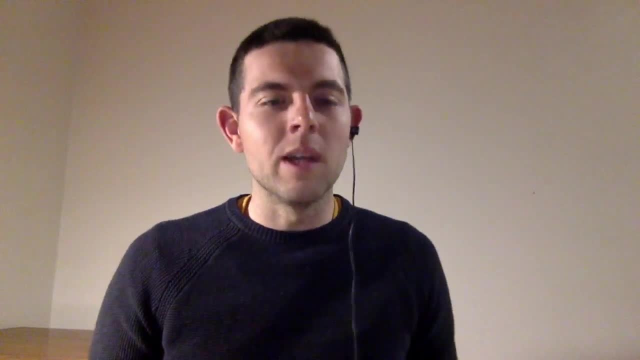 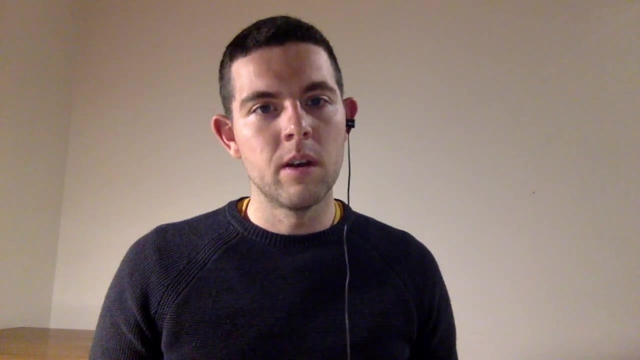 challenging detection. I don't think there's any doubt about that. but equally, you know, the payoff for such a detection is is potentially huge. I think any detection of the cosmic neutrino background we would learn a great deal about physics in. you know the to me the temperature. 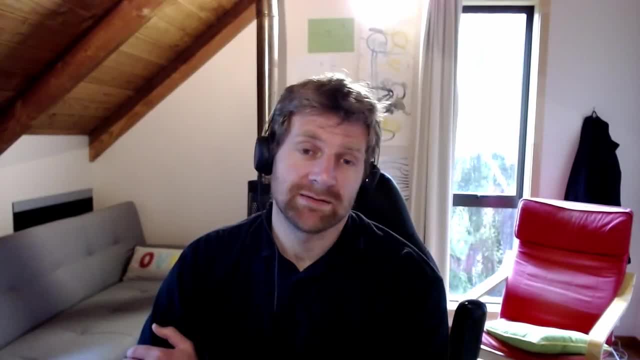 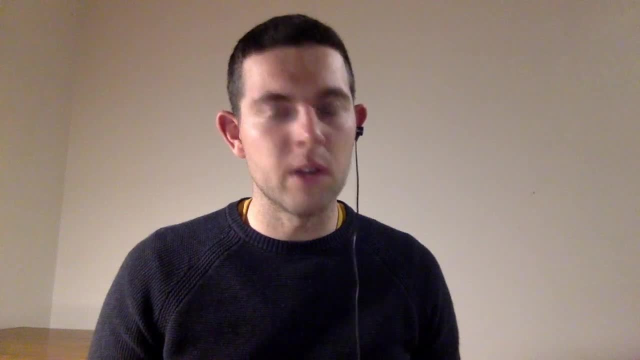 window in the very, very, very early universe. you mean, even if we literally just measured- not the anisotropy is obviously, but just the say- you measured the temperature of the neutrinos, I think you know you, you would learn something very deep about physics in the first tenth of a second in the universe. and you know that strikes me as someone. 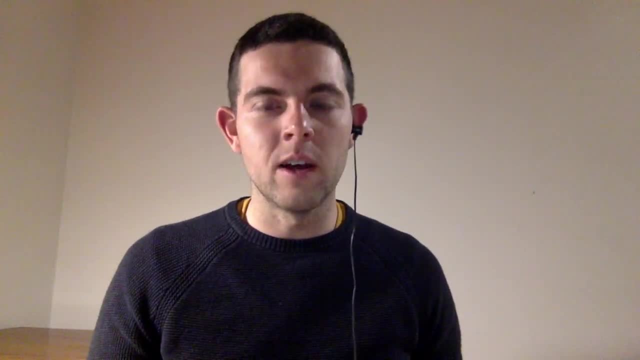 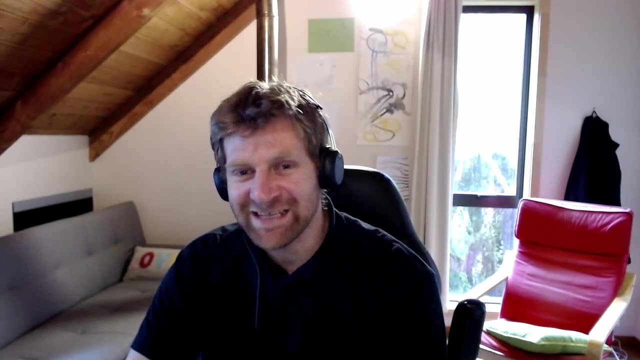 with huge potential, but it's actually relatively underexplored, especially on the kind of experimental side. yeah, yeah, I think this, this is this is like a very good answer to this question. certainly this is the sort of thing that if it comes up, if like a first-year PhD, 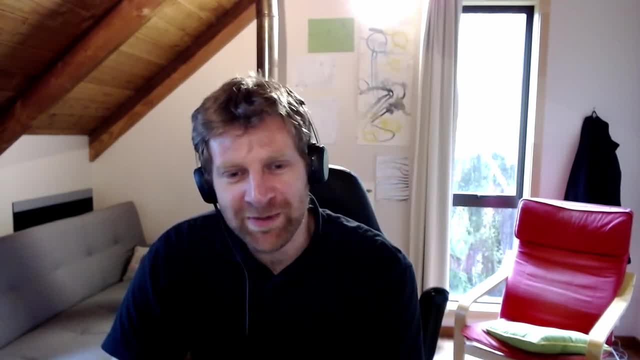 student asks the question at a at a conference of: oh, could we measure the cosmic neutrino background, everyone's like, oh, what a silly question? of course not, whereas, as you said, if if we were clever enough to actually measure it, it would be amazing. so if, if there are prospects for it, and then it's.